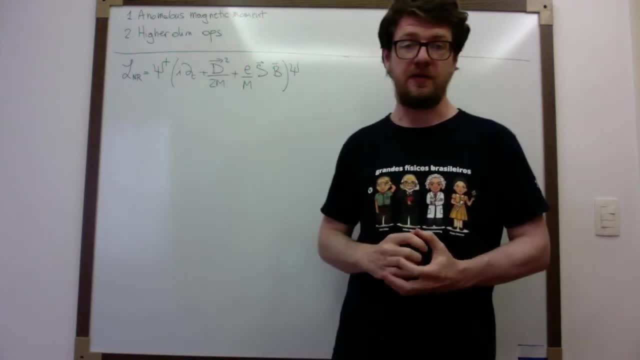 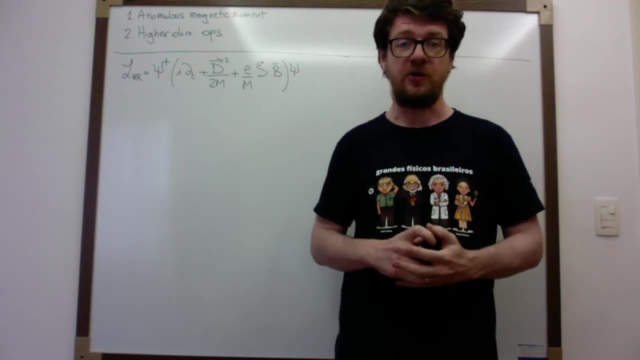 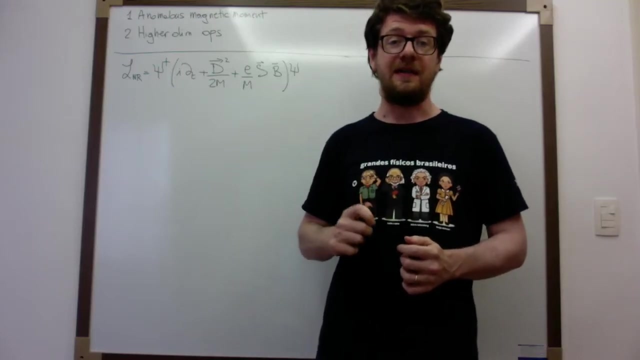 say some things about higher dimensional operators. Up to now, we just discussed the lower dimensional operators present in our Lagrangian, And today we're going to say something more about what happens when we turn on those operators that are inversely proportional to the carton. 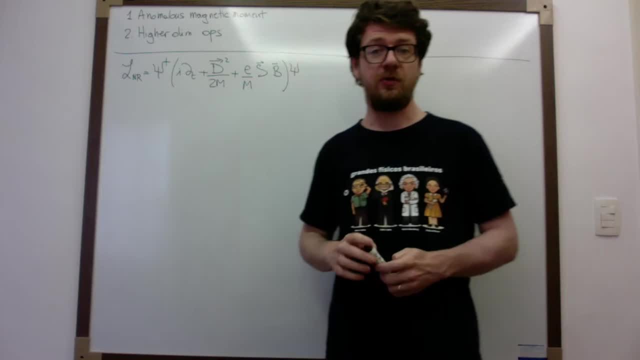 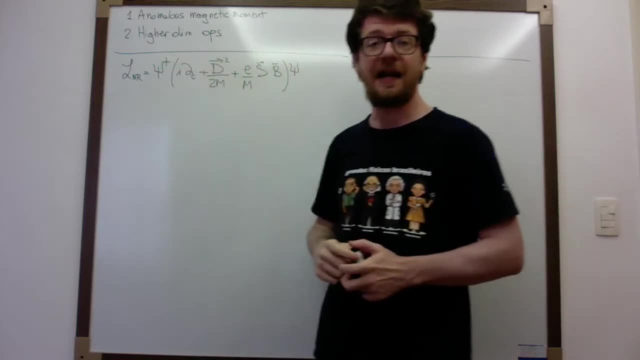 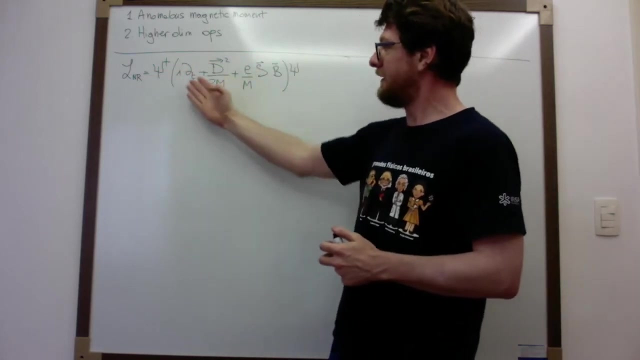 So let's start with the anomalous magnetic moment. So in the last lecture we discovered that a non-relativistic version of our QED Lagrangian is this: one in which the fermion field has a part of this Lagrangian, which is precisely the one that you expect in a non-relativistic. 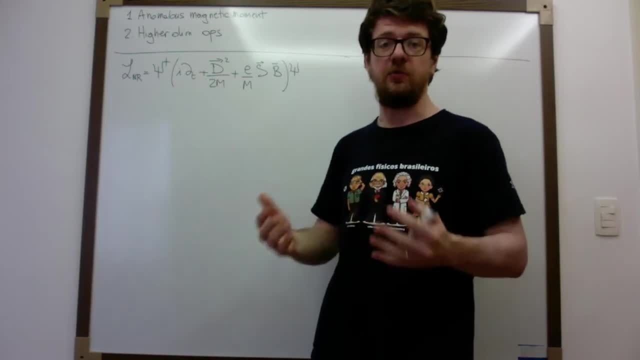 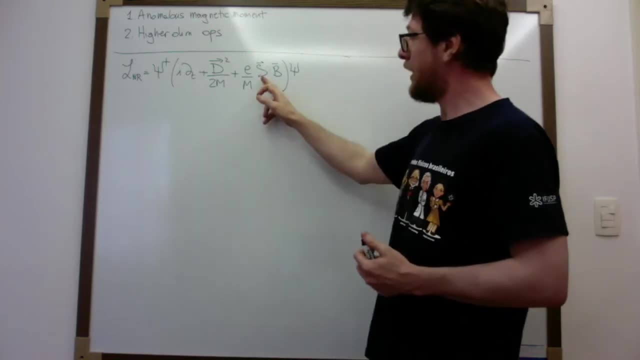 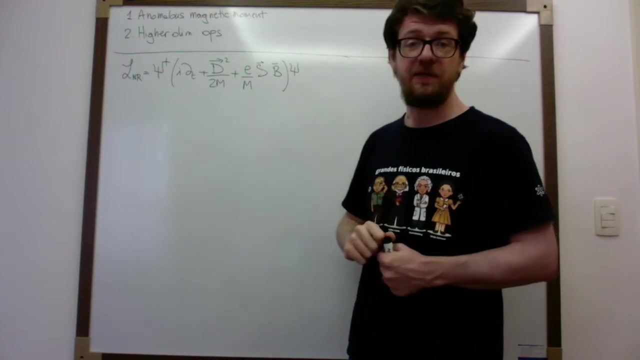 quantum field theory, which is very nice because this allows us to recover non-relativistic field theory starting from a relativistic theory. But then we discovered that, because of the non-vanishing spin of our spinor, of our fermion, there is a coupling with the magnetic field. 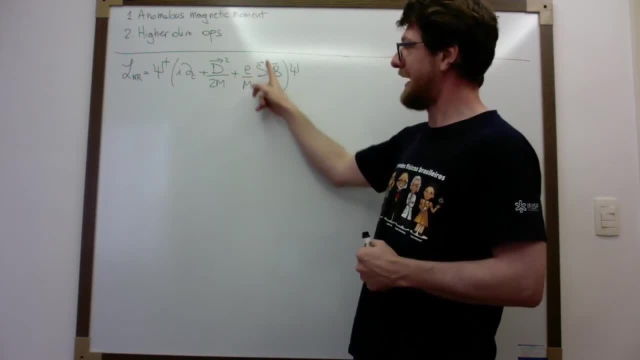 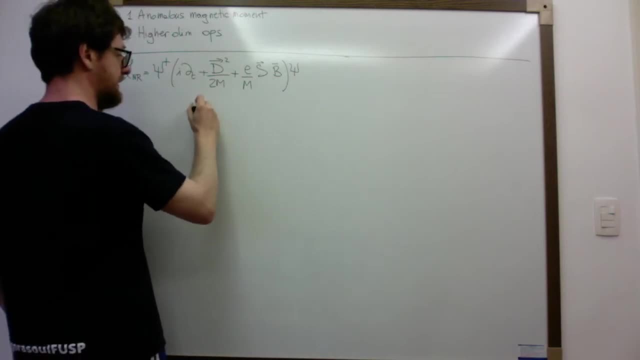 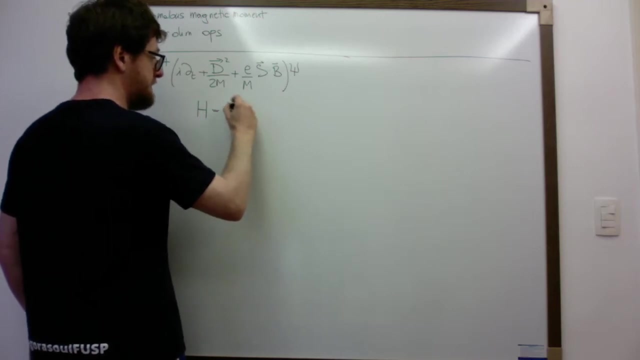 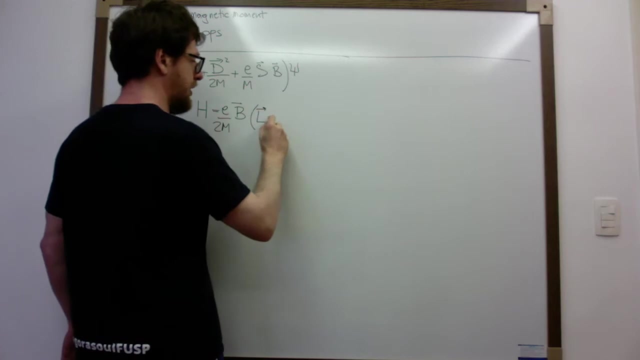 This object is called the magnetic dipole moment. okay, And usually, as we saw, what we write is something like Neville Tony is something like: let me write this: b, E over two m, And then here there is the orbital-orbital momentum plus. 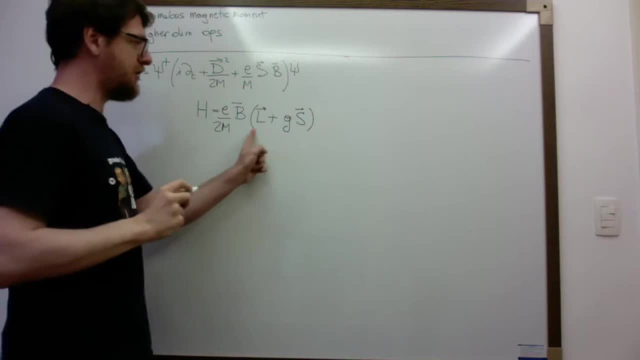 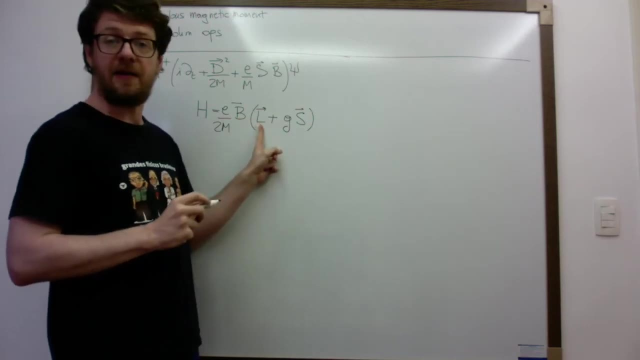 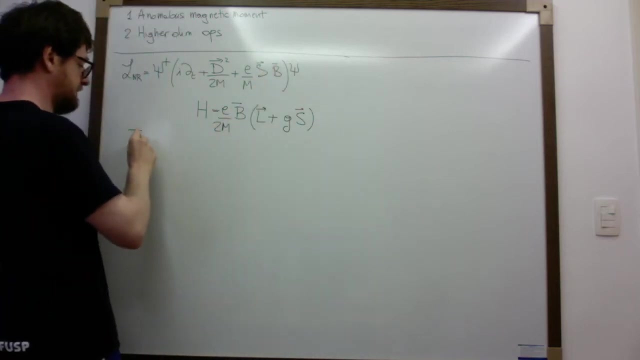 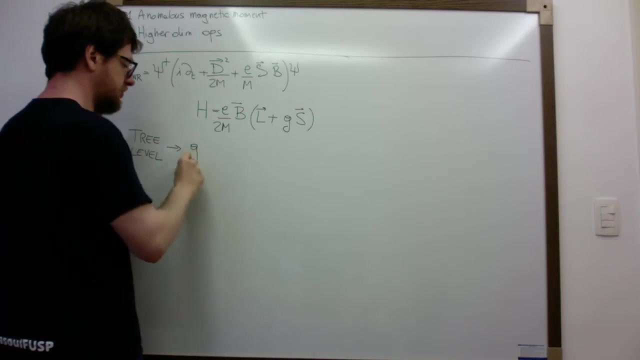 the effective g times s okay. So g measures the relative strength between the coupling between the magnetic fields and the orbital angular momentum, or the spin angular momentum. And what this is telling us is that at three levels. so before considering loop corrections, g is exactly equal to 2.. 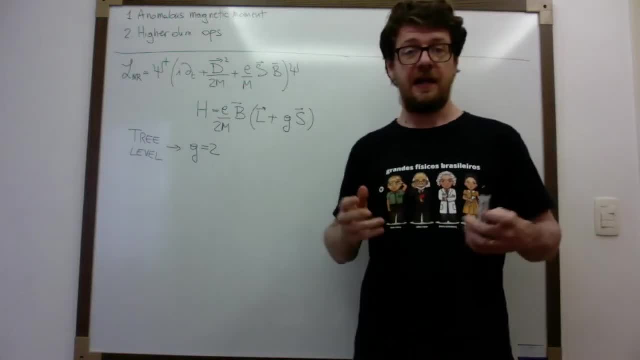 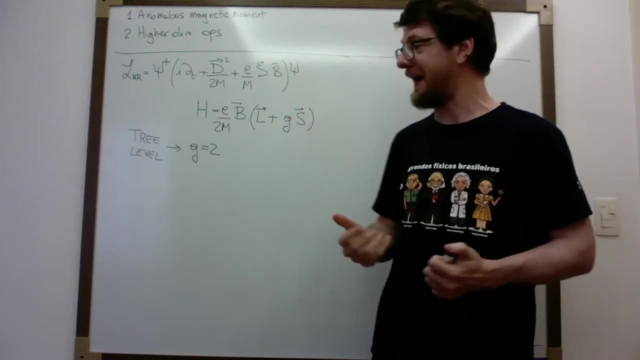 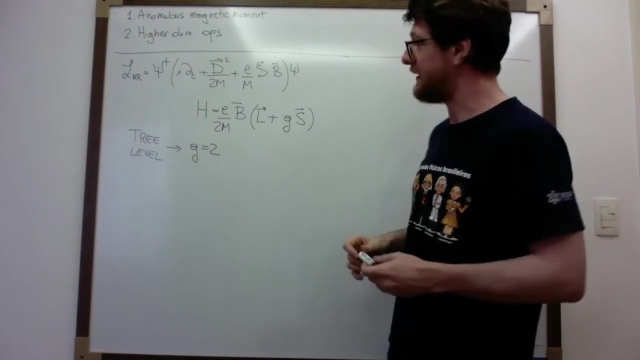 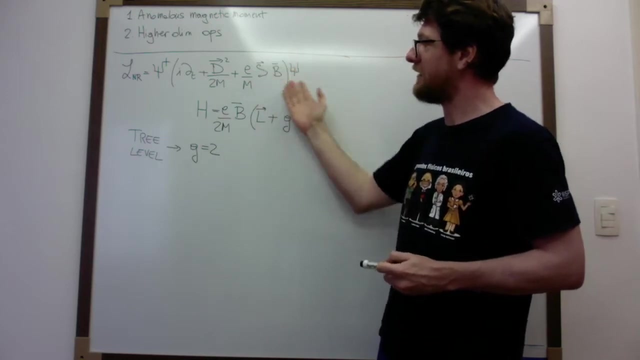 This was one of the first and greatest successes of the Dirac theory. This is the quantum field theory version of the Dirac theory, And this first prediction was very successful because this was something that was starting to be seen experimentally. Now the question is: what is the type of terms that we can write in our Lagrangian that will 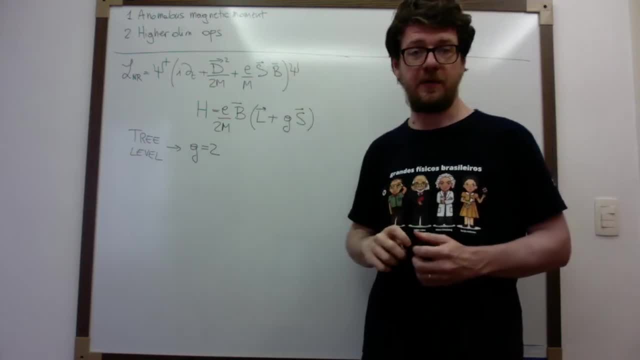 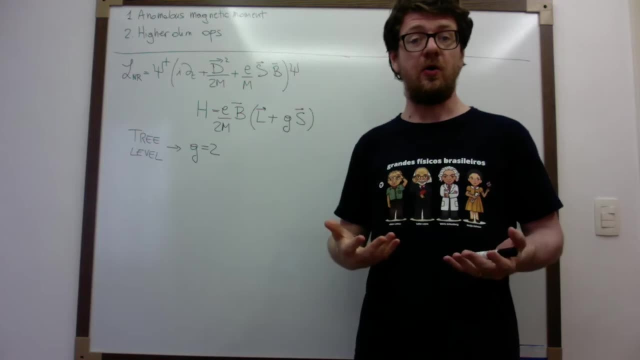 allow us to keep track of these terms. Okay, As we're going to see, radiative corrections will generate some operator. Okay, And once we know the coefficient of the operator, we will know the gradient of the operator, And then we will know the gradient of the operator. 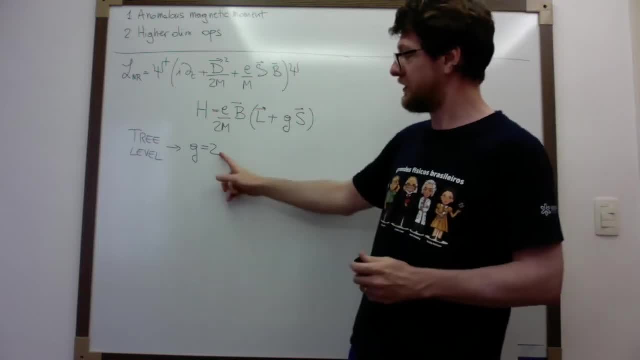 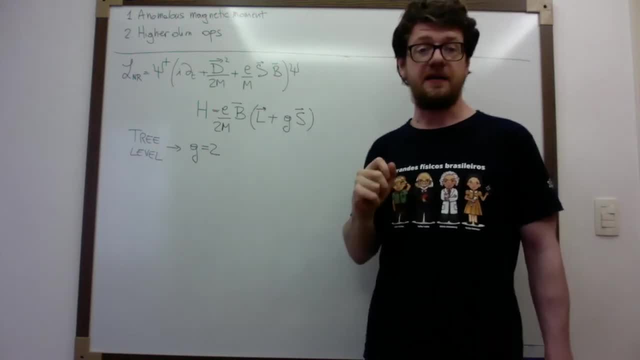 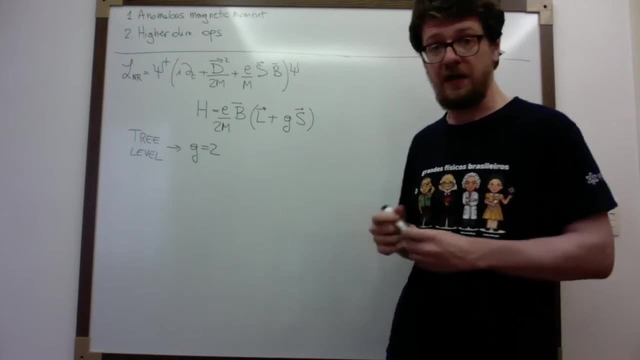 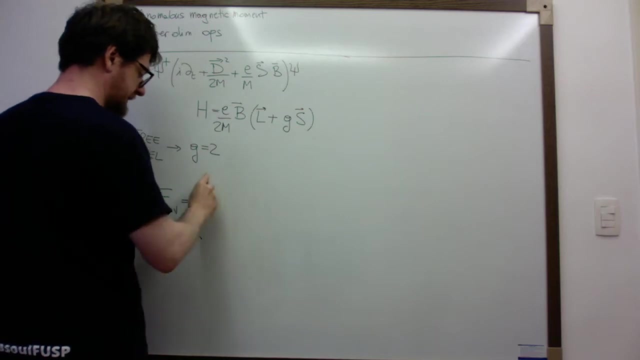 think a bit about where the magnetic field appears. Well, the magnetic field appears directly in the field. strength of the photon. Okay, Let me just remind you that F mu nu is something like this: It has zero on the diagonal because it's an anti-symmetric tensor. 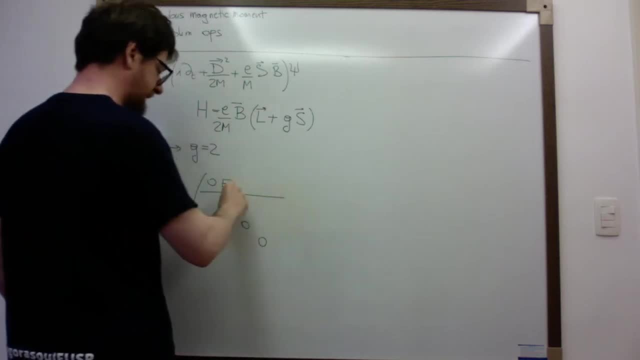 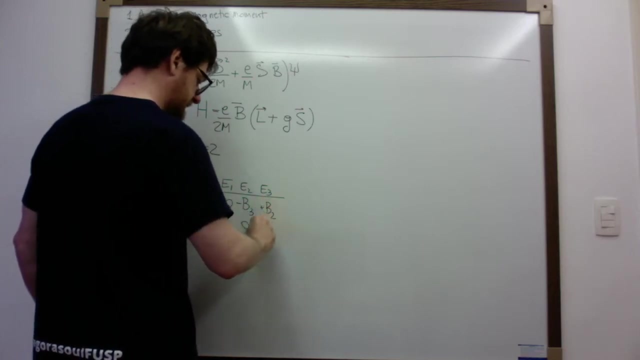 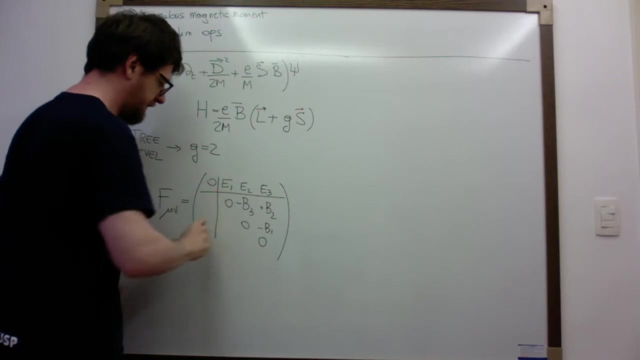 Then here in these entries, it has the components of the electric field, And here it has the components of the. I think this is a minus plus B2, minus B1.. It has the components of the magnetic field And then of course you can fill the rest just by anti-symmetry. Okay. 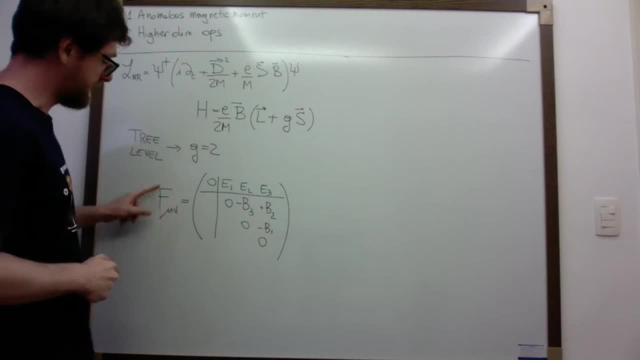 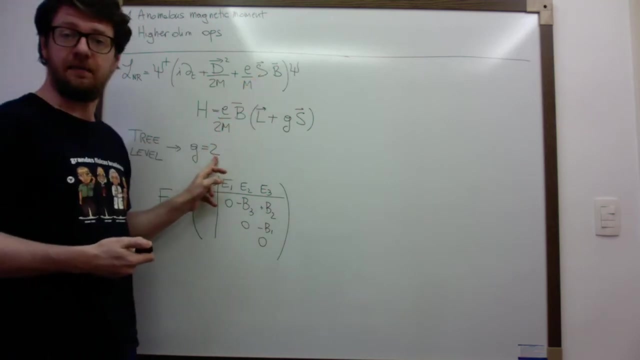 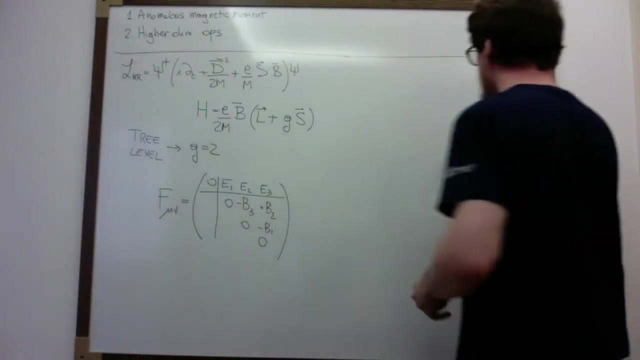 So you see that if we're able to write some operator that involves simply F mu nu without involving directly the full potential, then we're going to couple our fermion to the magnetic field directly, And so we're going to modify the magnetic moment of the fermion. Okay, Now if we want to write some interaction that contains F mu nu, 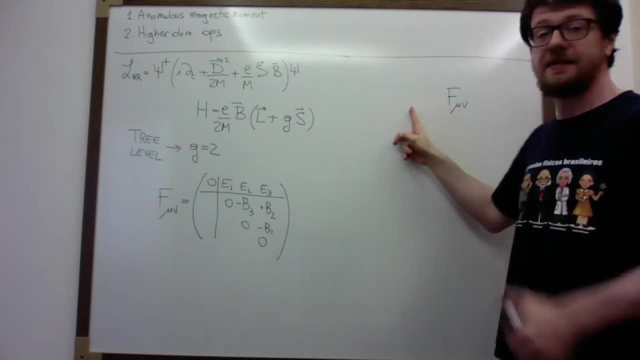 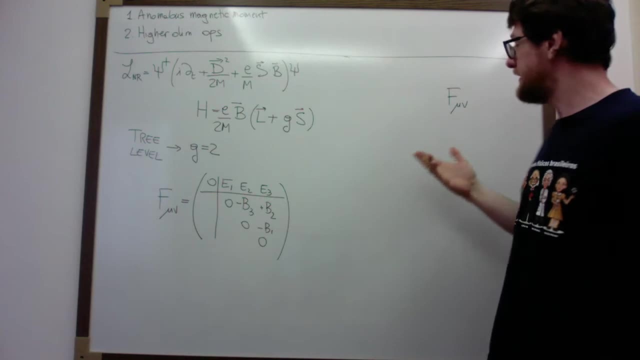 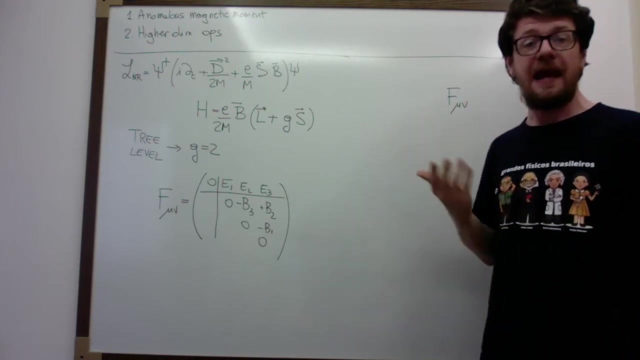 this F mu nu must be contracted with something which is anti-symmetric. Okay, So, since the only object that carry Lorentz indices here in a QED are the field strength itself, the full potential- which is already included here, so we can't use- and the gamma matrices, 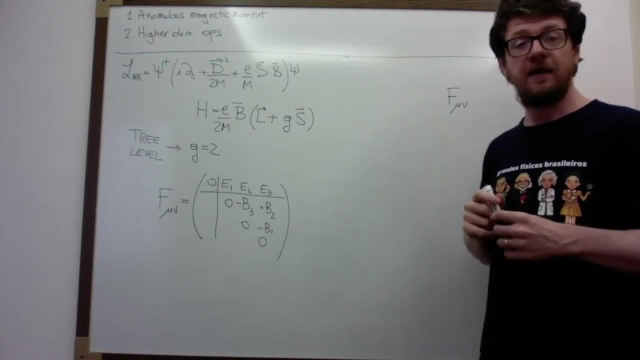 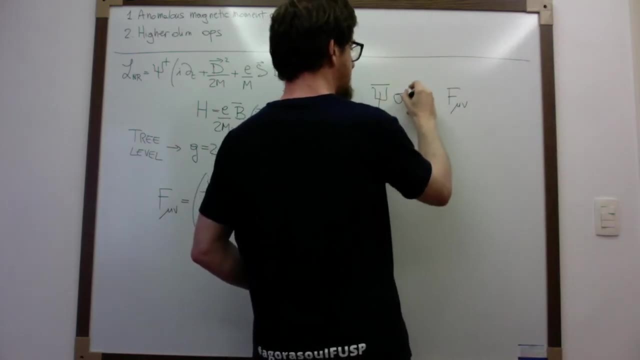 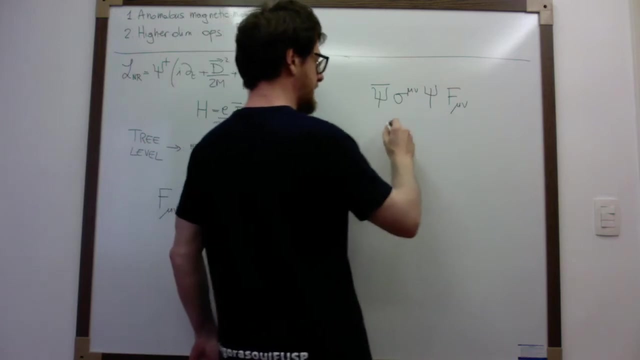 this means that here we need to put some anti-symmetric combination of the gamma matrices. Okay, And the correct one is the power. So this is the fermion field, And let me introduce an object which is called sigma mu nu- Again psi, Okay, And this sigma mu nu is defined in the following way: It's a factor of i. 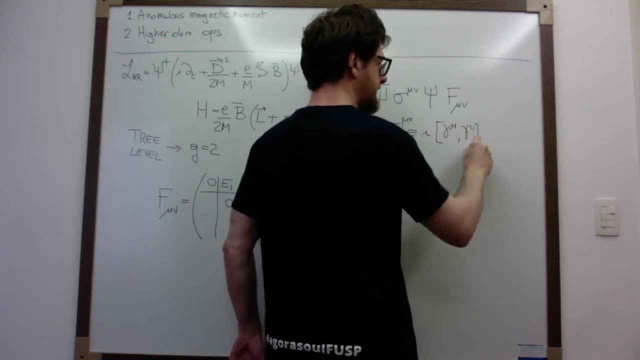 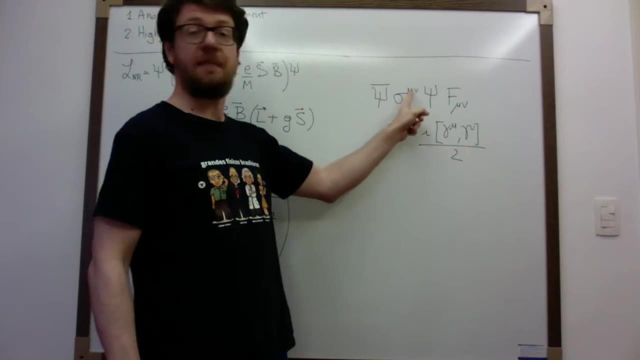 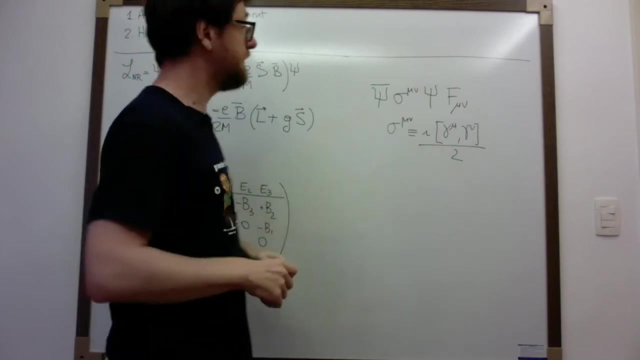 Then there is the commutator between the gamma matrices, everything divided by u. So since I'm putting here the commutator, this combination is automatically anti-symmetric in the two indices, And so it can contract with the anti-symmetric indices of the field strength. 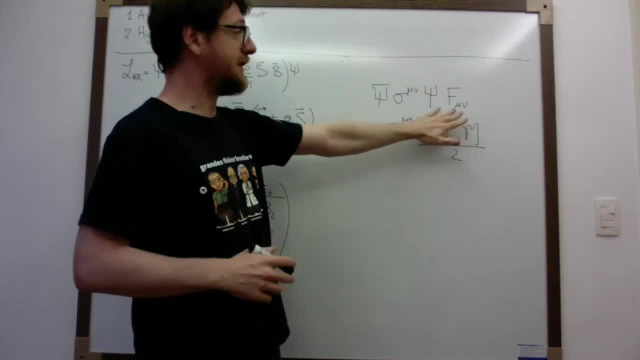 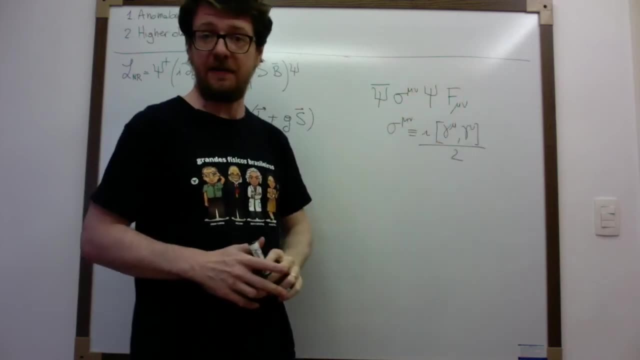 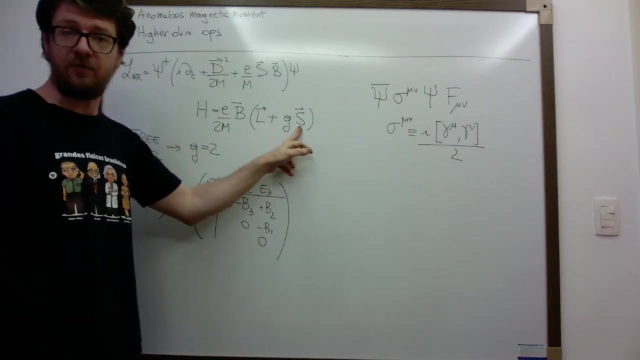 So from here we know already from four constructions that this has some coupling between the fermion and the magnetic field. Now we need to understand if this coupling is precisely of the form that we need, meaning if we are coupled to the spin of the particle. 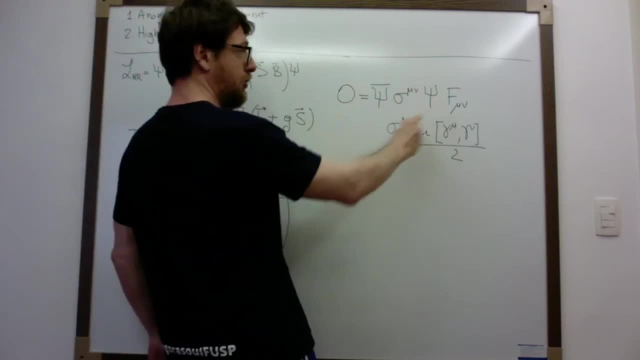 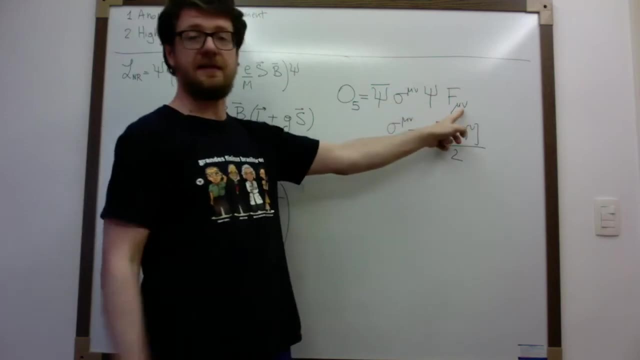 Okay, So this is some operator. Notice that this operator is a dimension five operator, right, Because you have dimension three for the fermion bilinear, and then this is an object of dimension two, So altogether you get something of dimension five. You can take this operator. 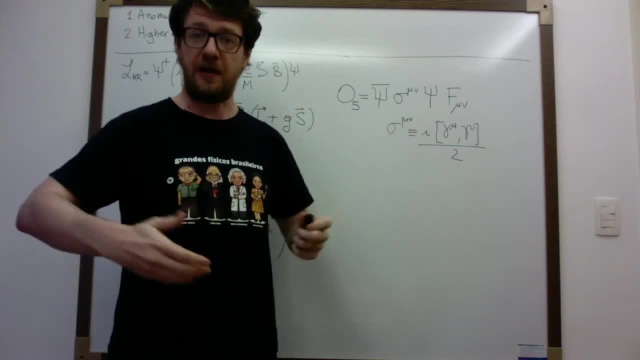 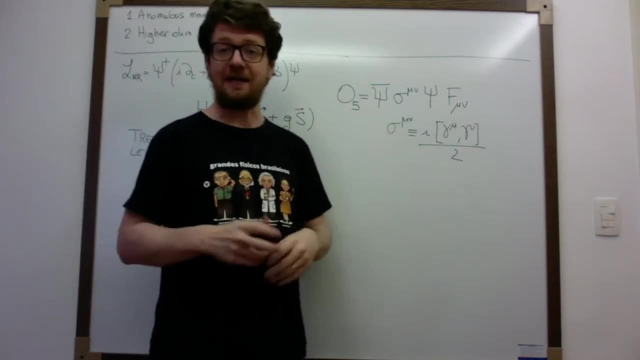 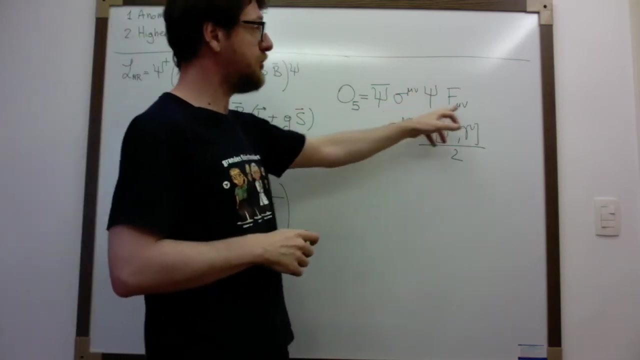 and play the same game we did in the last lecture, So going to the non-relativistic limit, separate the positive and the negative projection part of psi in terms of gamma zero one plus or minus gamma zero over two. You play that game. you compute what sigma mu nu f mu nu is. 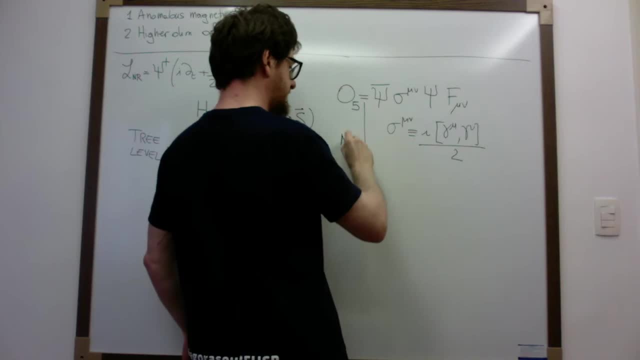 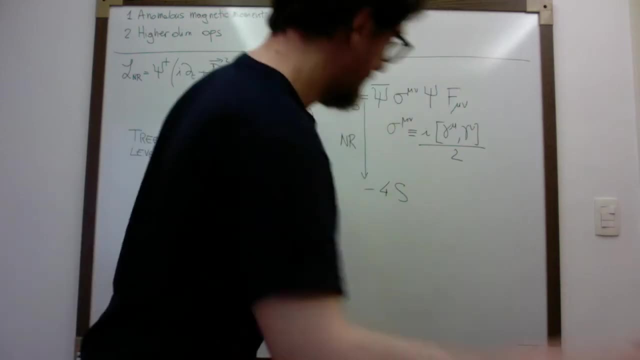 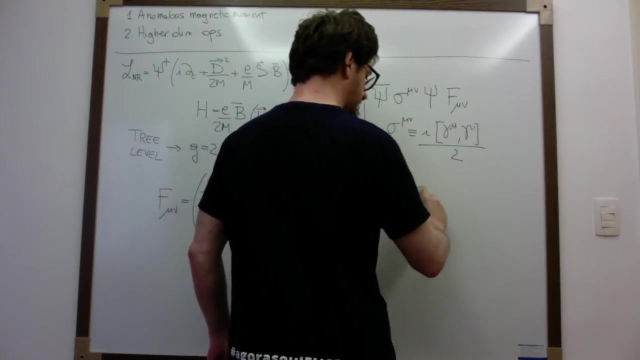 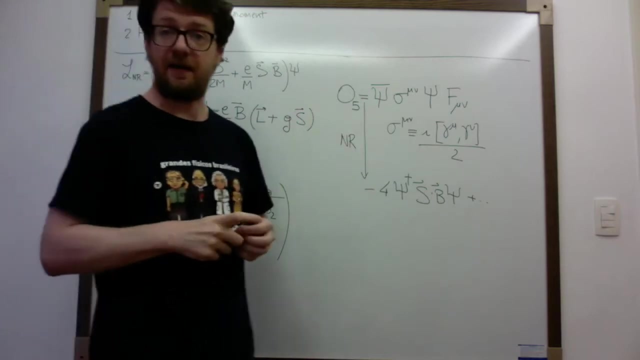 and you discover that this operator in the non-relativistic limit gives you something like this: It's minus four and you write the fermion field here: psi, dagger s, dot, b, psi, plus other terms that involve the electric field and are not interesting for us. Okay, So you see that embedded in this structure, 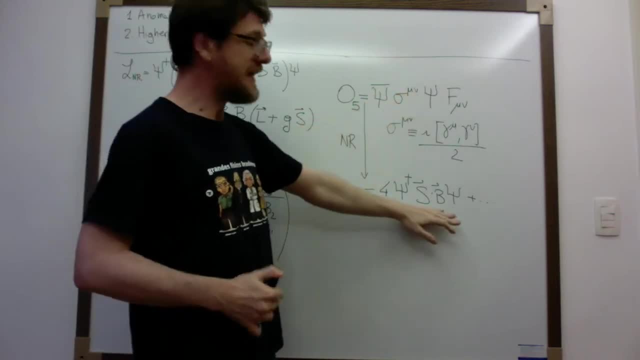 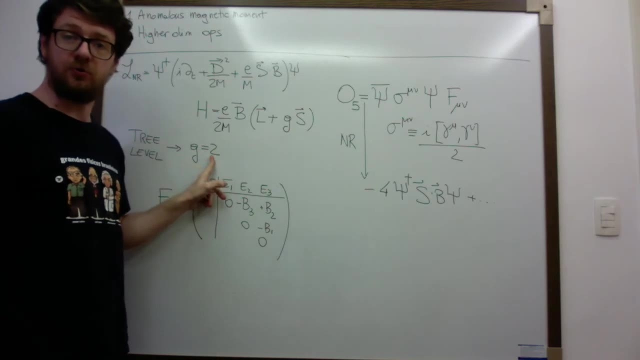 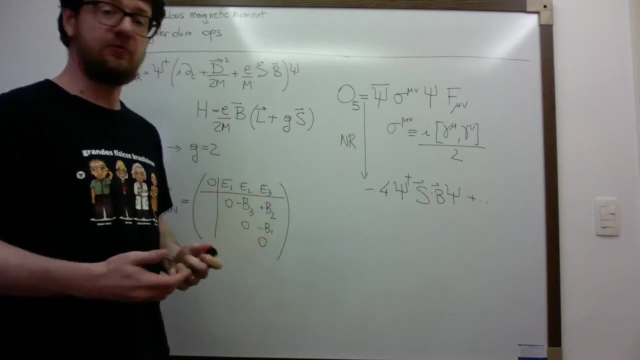 in this relativistic structure is precisely the form of term that we need in the non-relativistic expansion to compute what are the modifications to the g anomalous to the magnetic moment of the fermion? Okay, So what I'm now going to show you. 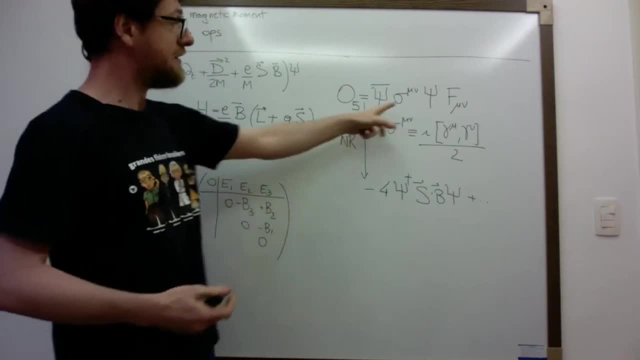 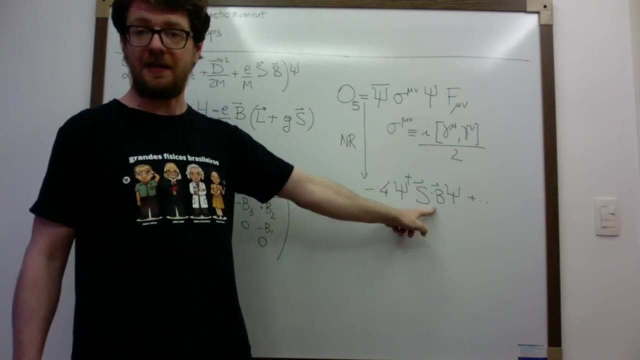 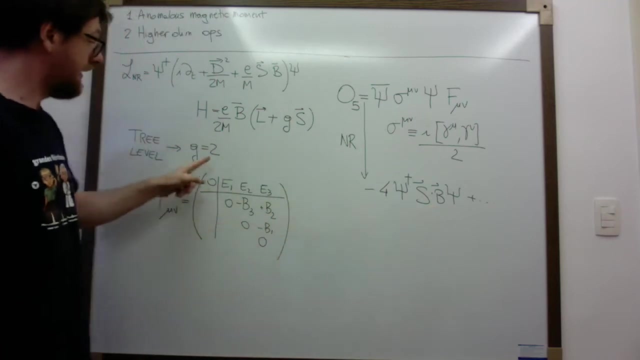 is that radiative corrections in QED generate precisely this term. And since they generate precisely this term, we're going to obtain a correction to the magnetic moment of the electron, which is called, then, the anomalous magnetic moment. Anomalous because it's something 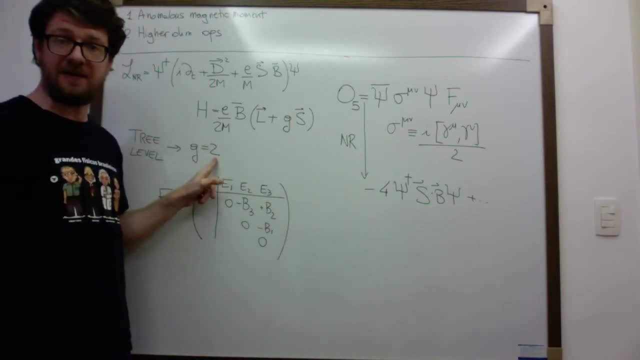 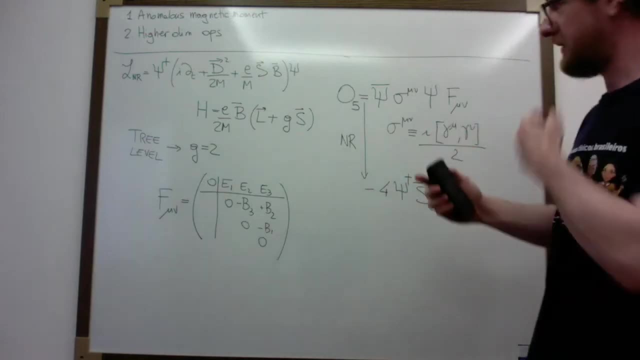 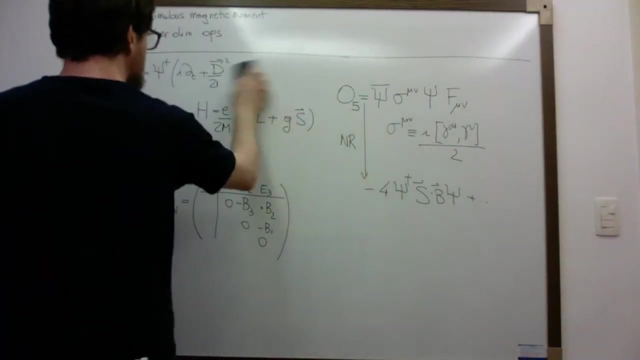 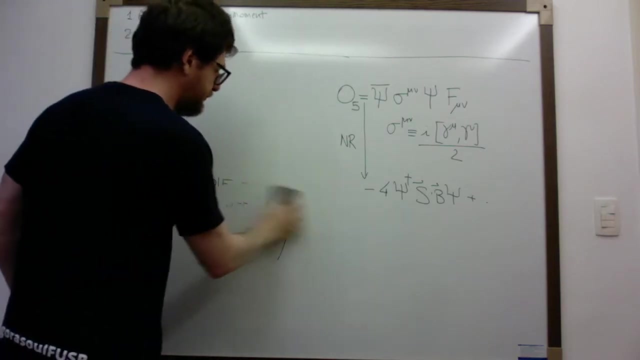 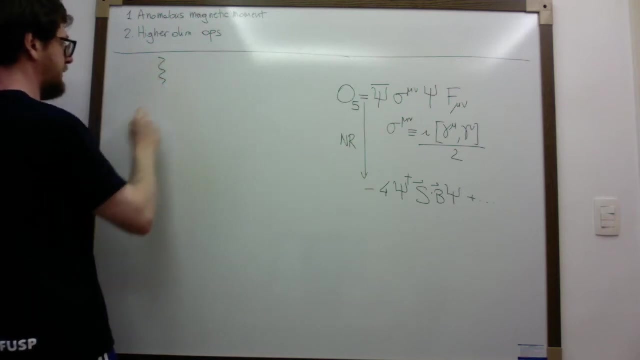 that happens in addition to what we have at three levels. So what are the diagrams that are interesting for this computation? Well, you see that somehow we need to couple two fermions with an electromagnetic field. So the diagram that we want must involve two fermions and one photon. It must be something like this: One photon, two fermions. 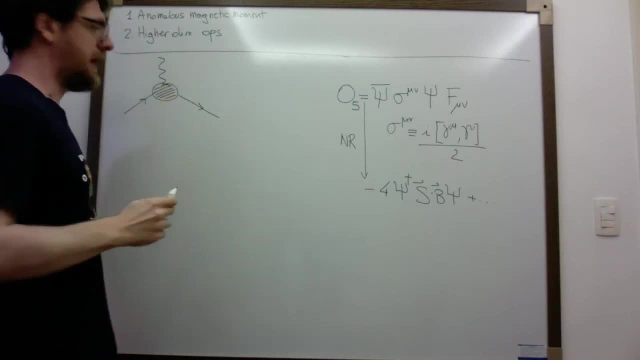 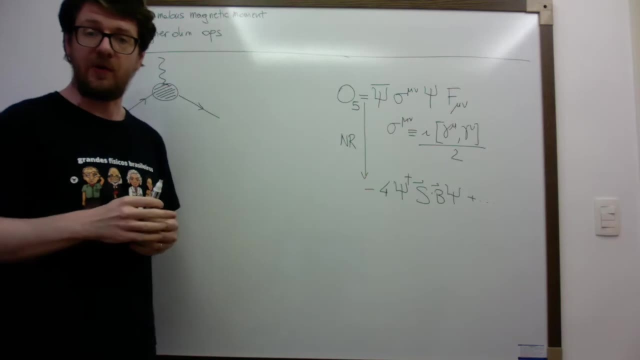 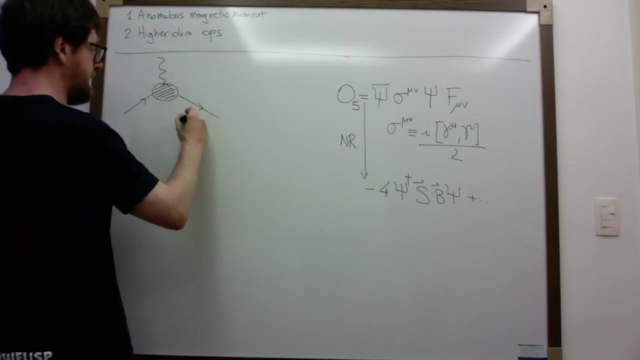 and here we will have something. Okay, So you can always imagine these as the one particular reducible diagram, Exactly as we did when we were computing the radiative corrections and the running of the electric charge. So let's give some name to the momenta. So let me call the outgoing 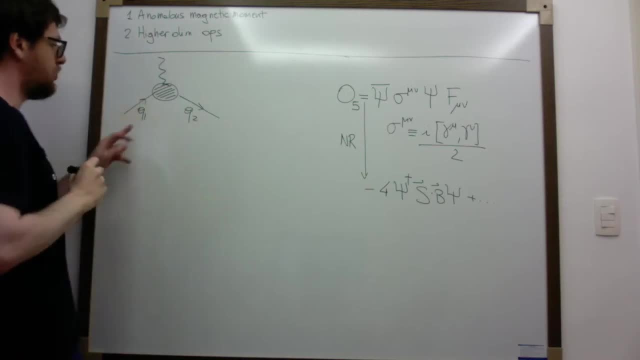 momenta of the Firmium Q2.. Then we call Q1 the in-going momenta of the Firmium. Then we call the peak and the incoming moment on the Firmium Q2.. And then in the future we click the momentum. 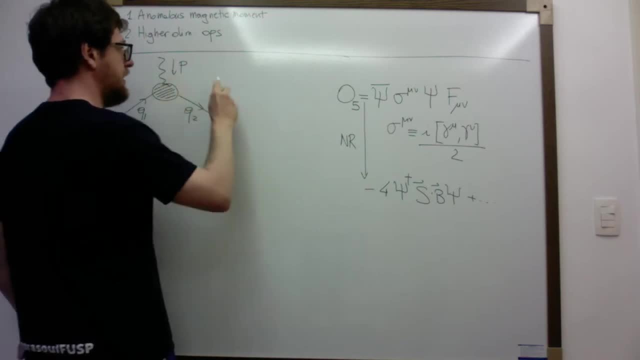 of the� MoM of the e et al last moment, and we will be learned how it goes. Horrification is generally a different equation. That means that key to production is simply the computer不是 momentum of the photon, and so this P must be equal to Q2 minus Q1.. Okay, 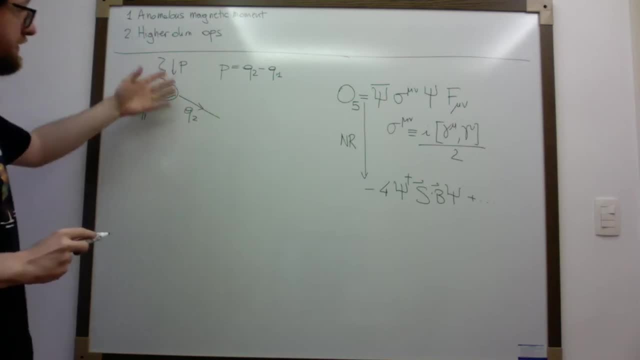 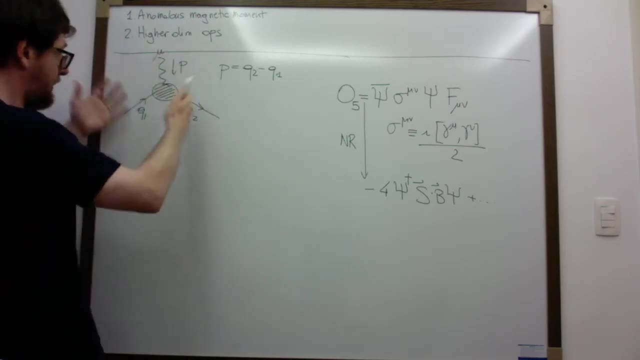 Now, what is the possible structure of this object? Well, remember that here we have an Lorentz index right. So at the end of the day, this object here must be something like this: Just by covariance under Lorentz transformations, it must be some U bar, depending on Q2,. 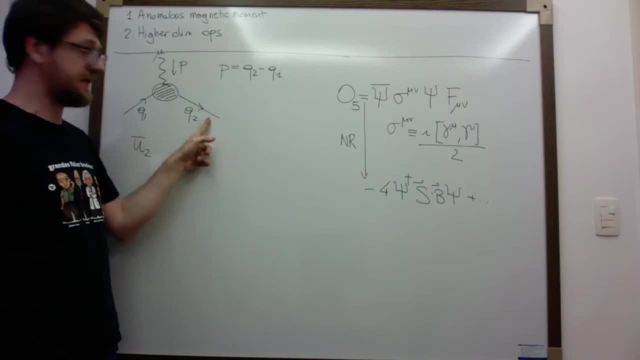 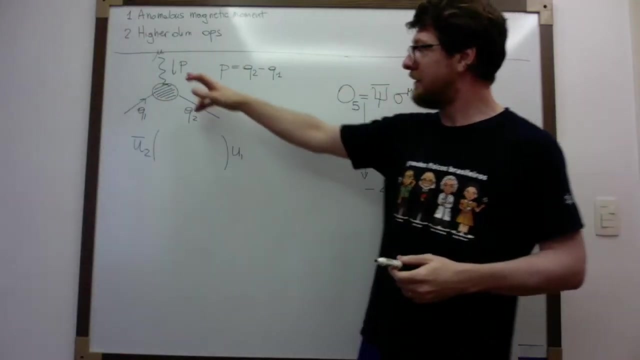 which takes into account the creation of this fermion here. Then there must be a U1 here that takes into account the destruction of this particle, And then here in between I'm going to write all possible terms that have one Lorentz index. So we start with a gamma mu, because it's 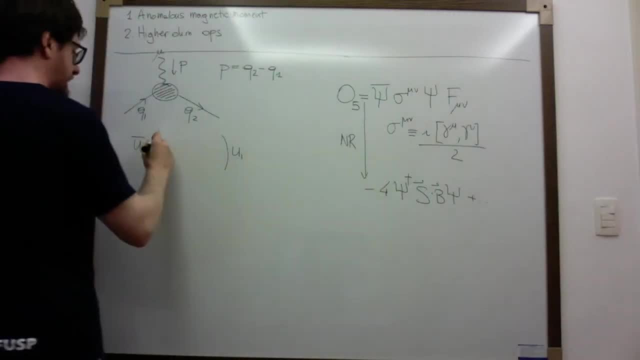 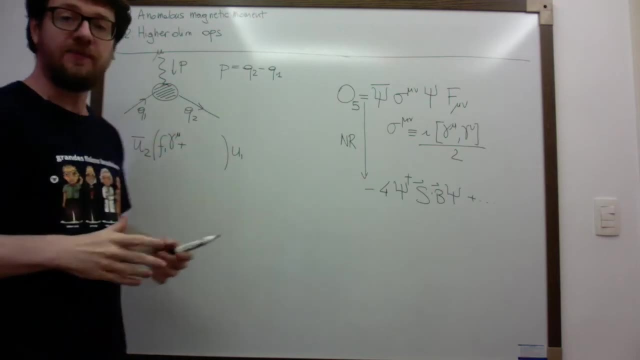 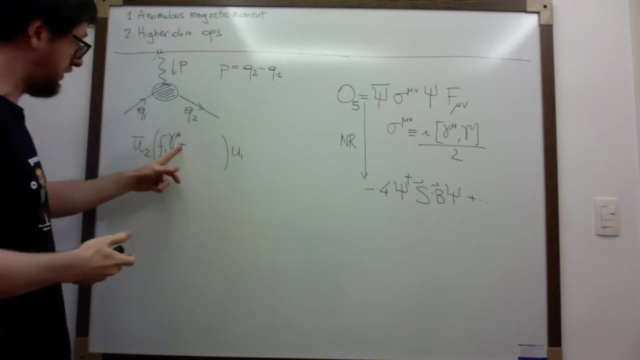 something that, for instance, at three levels we obtain gamma mu. So here I will have some function F1 times gamma mu. Then what are the other objects that I can write? Well, I have three objects. in principle I have three momenta, and all of them are four momenta. So in principle all of them should appear here. 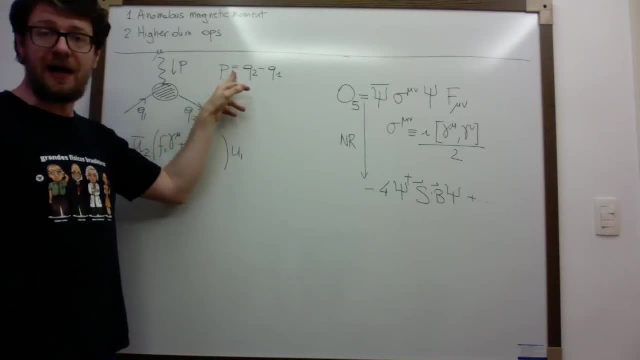 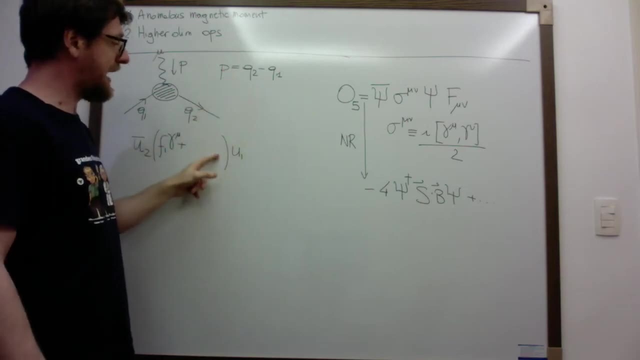 One is redundant because of this relation, So I can simply avoid to write the term proportional to P mu here, because I know that I can always rewrite that term in terms of Q1 and Q2.. So here we just write these two terms. 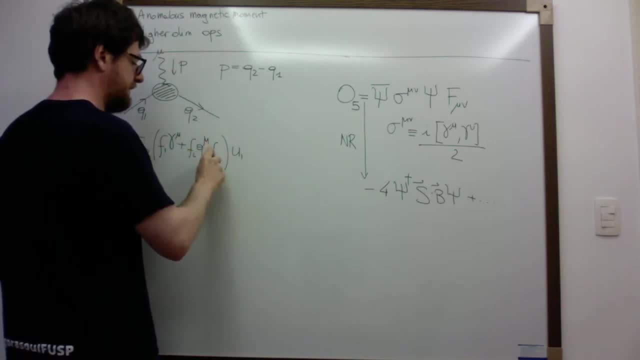 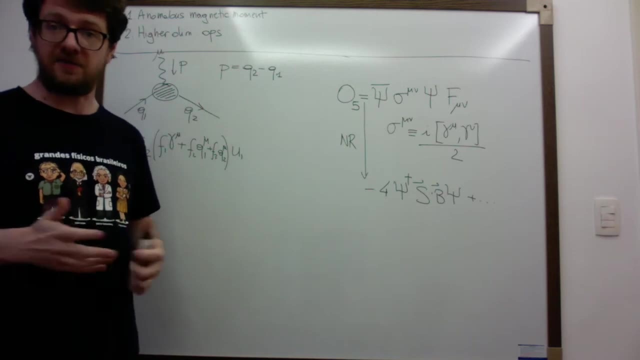 F2 and Q2.. Q1 mu and F3, Q2 mu, And that's it. There is nothing else that has the right transformation properties under Lorentz transformations. So this F1, F2, F3 are not. 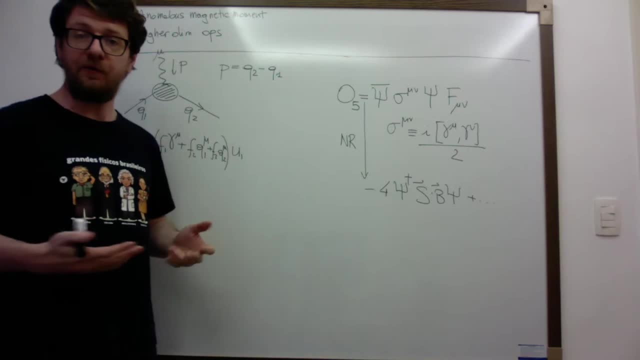 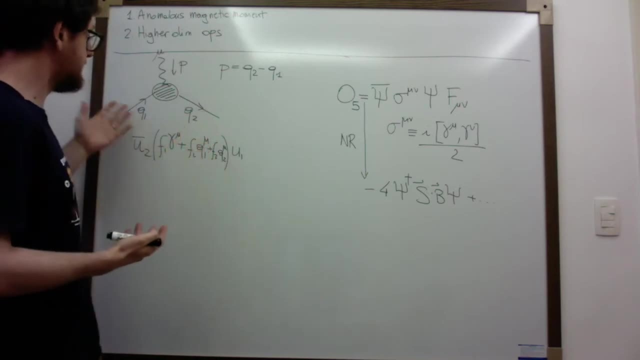 constant, but they can be whatever function, which is a Lorentz scalar. that depends on the kinematic structure. here, At the end of the day, the only kinematic structure that can appear here, you see, that are either the masses, so they're constant, or the momentum of the photon. So there is this. 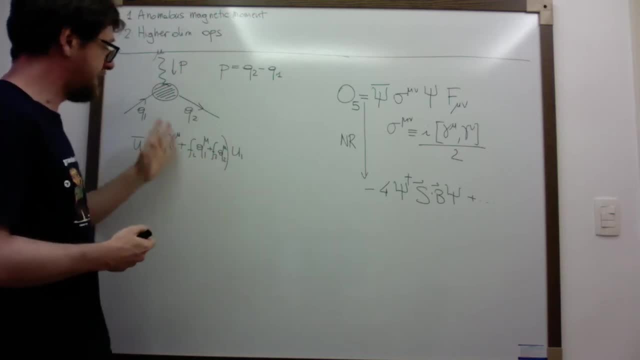 F1,, F2, F3 are simply functions, So there's 1,, 2, and 3. They can only depend on P squared and if you want capital, M squared, which is the mass of the particle, Very good So. 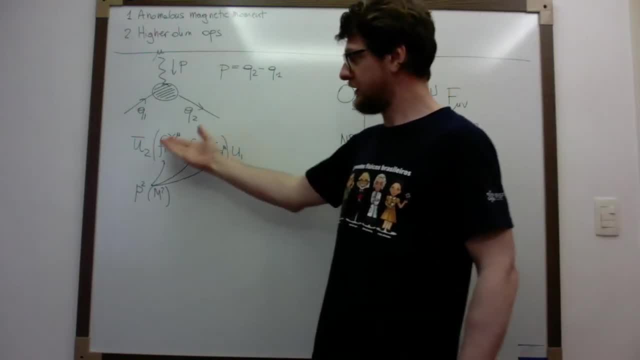 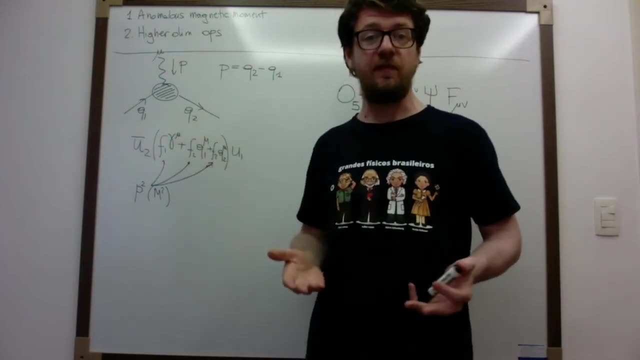 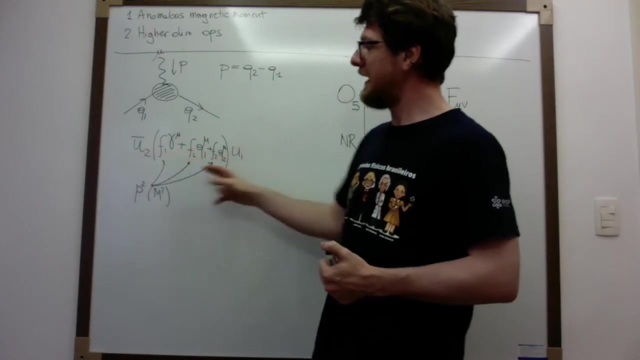 can we use some other line of reasoning to constrain this object? Well, yes, Yes, we can, because this is an amplitude. So since we know that the gauge invariance must be satisfied in our theory, then we can try to multiply it by P? mu and see what happens when we impose that this. 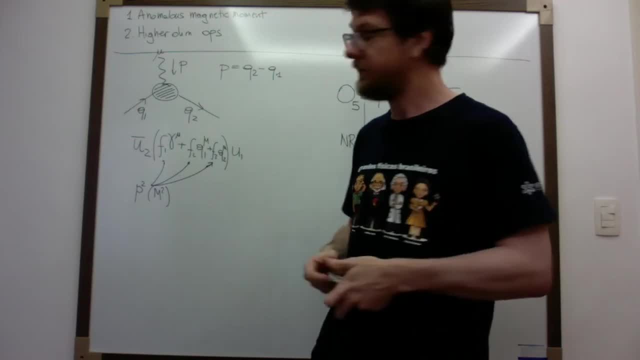 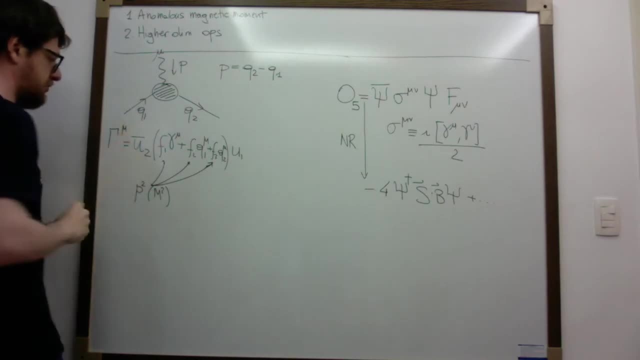 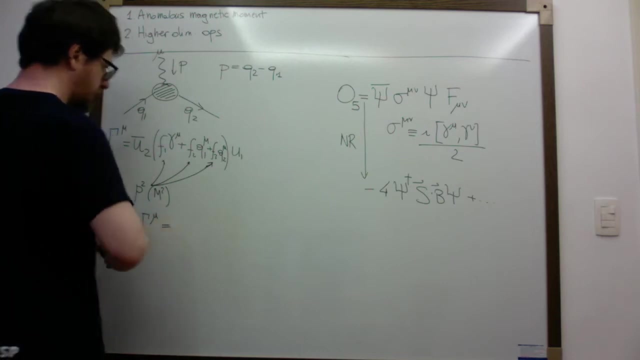 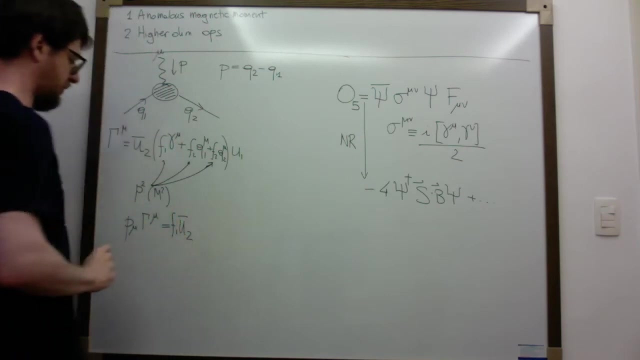 multiplication, that this contraction must be equal to Z. So let me call this object capital gamma mu, just to give it a name. So if I compute P mu, capital gamma mu, what do I get Well, from here? the first term gives me a U2 bar, so there is a factor of 1. Then I have a P. 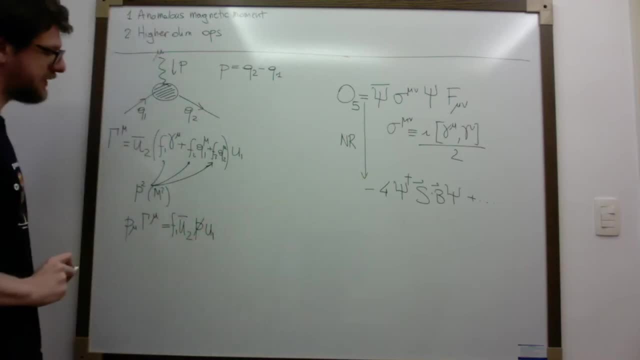 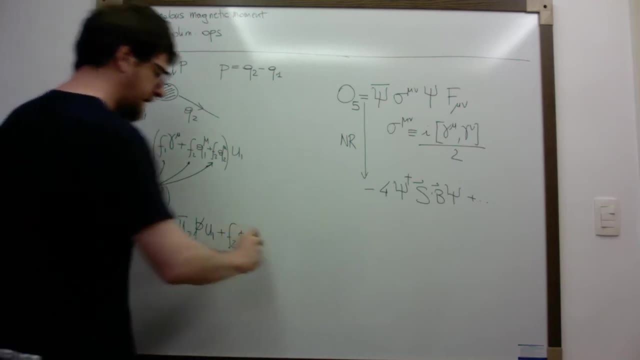 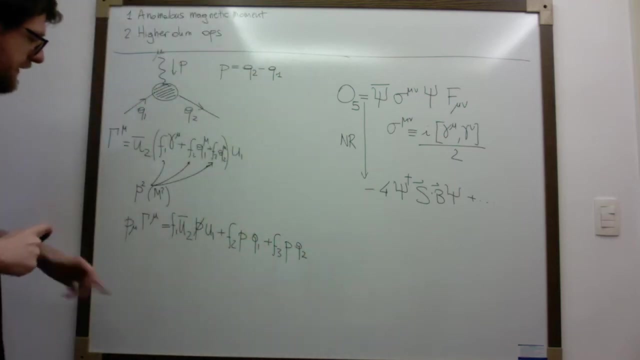 slash and then I have a U bar. Then the second one is giving me P dot Q1, and the third one is giving me F3 P dot Q2.. Okay, So now we will try to simplify this expression. So the first: 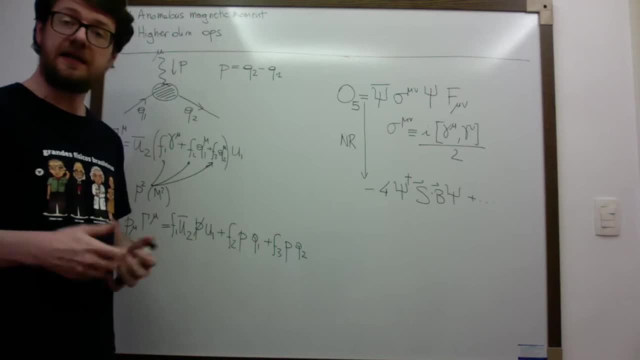 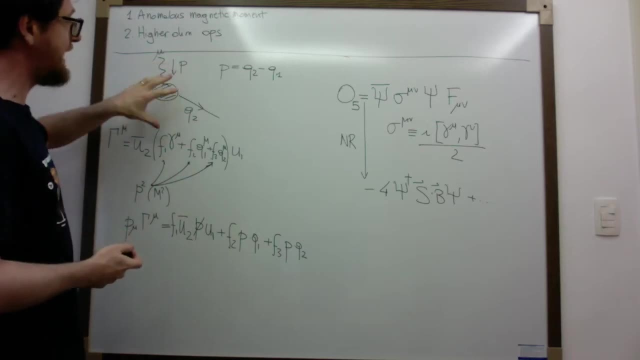 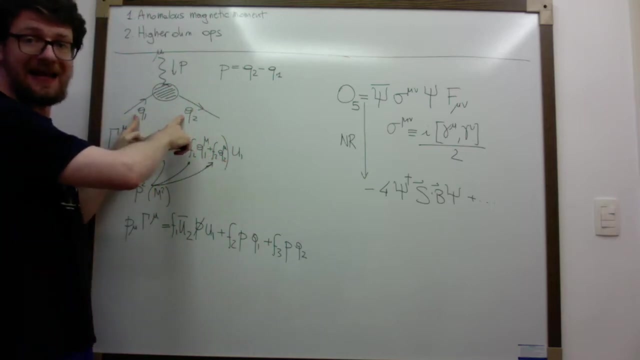 simplification that we can consider is to put the fermions on shell. Okay, So we will suppose that we are considering this diagram as a part of a higher diagram, a larger diagram in which the two external electrons are on shell. Okay, So we will suppose that the two external electrons are. 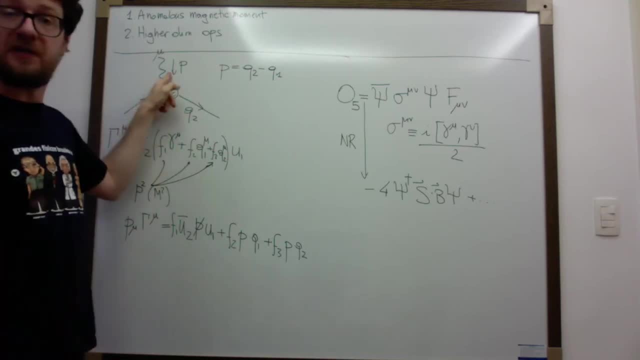 on shell. Okay, So we will suppose that the two external electrons are on shell. So we will suppose that the two external electrons are on shell, So they are physical particles and the photon is not. Okay, So I can't have a physical amplitude that involves. 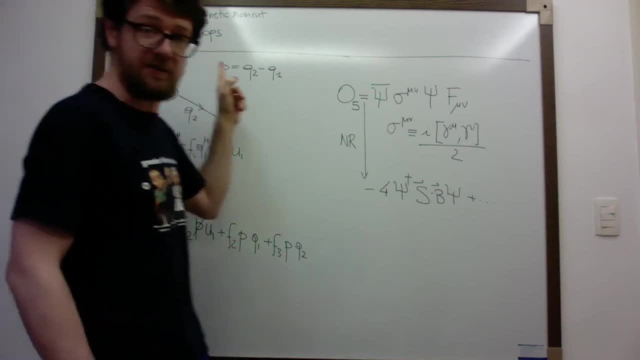 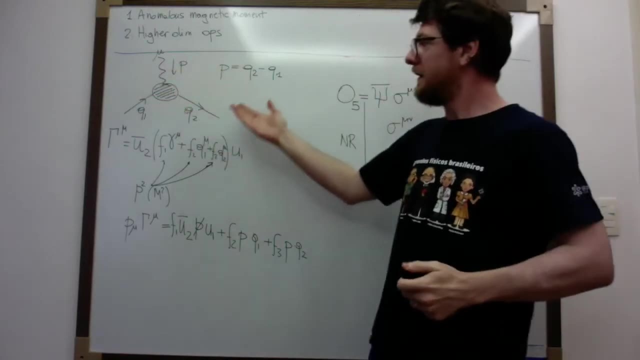 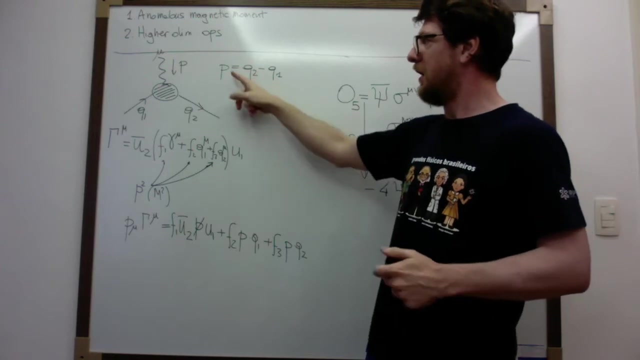 two master particles and one master particle, because kinematics concludes it. Okay, This is a simple exercise in special relativity, but you want to keep in kinematics. You see that if you try to put these three on shell and you start to compute the squares of this form, momentum. 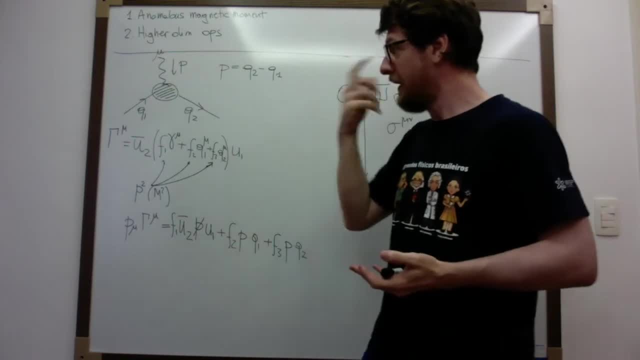 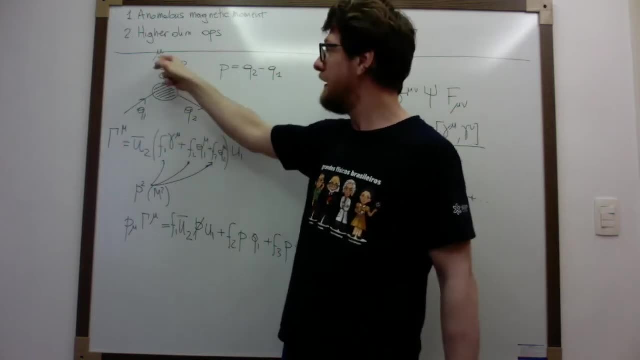 then things are not consistent, So this is something that I can't have. But what I can have is an amplitude in which the electrons are on shell, so they're physical, and the photon is not, So I'm coupling the photon up here to some other diagram. 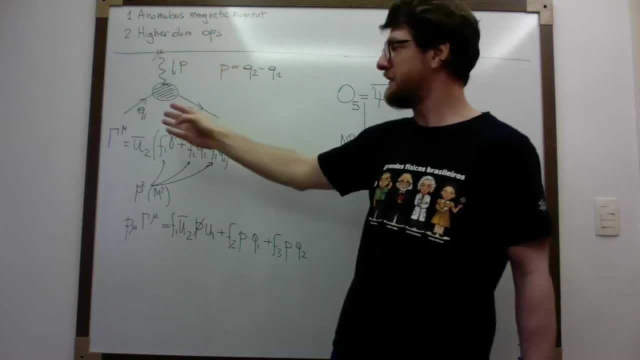 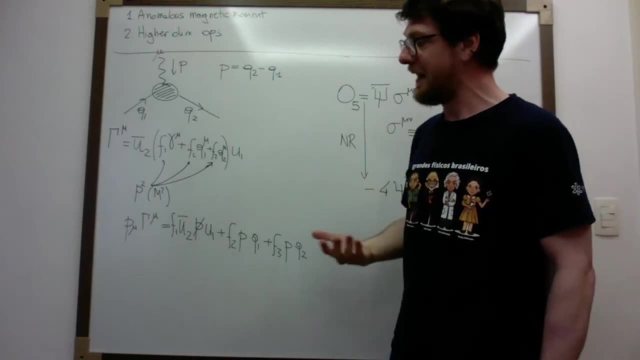 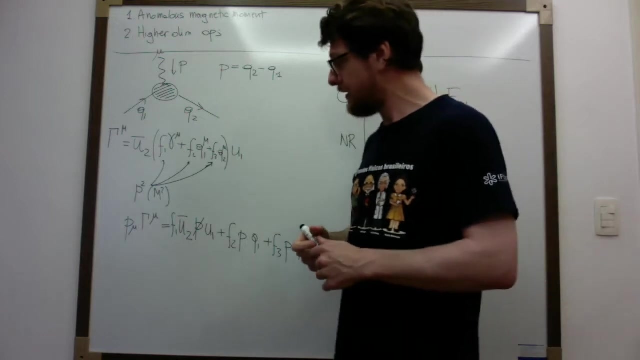 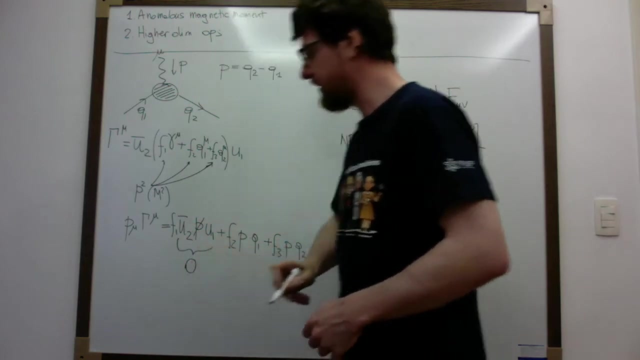 For instance, this can be a T-channel of some electron-electron scale. So that's the game that we're going to play. So why do I play this game? Well, because if I take the incoming and outgoing electrons to be on shell, then using the equation of motion for the electrons, you discover that this object here is equal to zero. 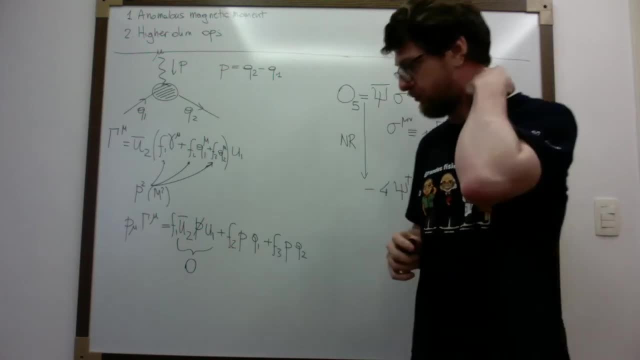 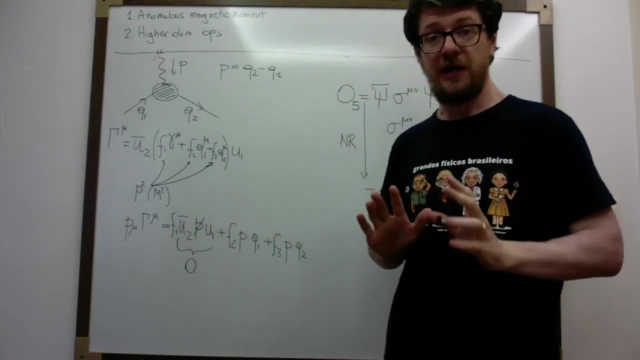 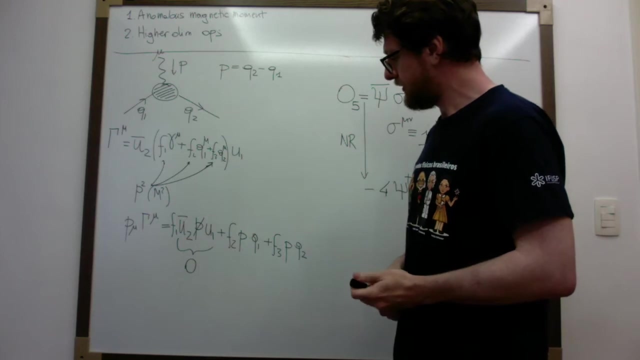 So this is something that I invite you to check explicitly and to show that this is true. But this object here is precisely equal to zero on shell, only on shell, So I'm left with these two. So what can I do about these two terms? 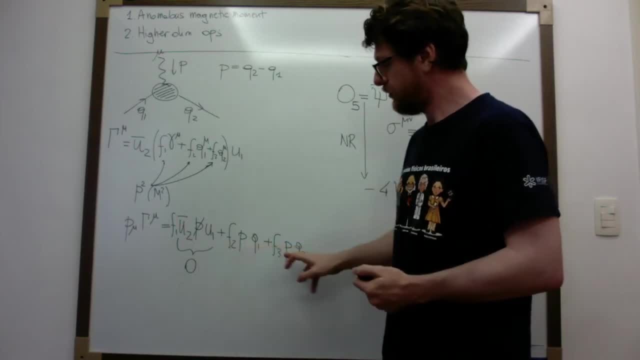 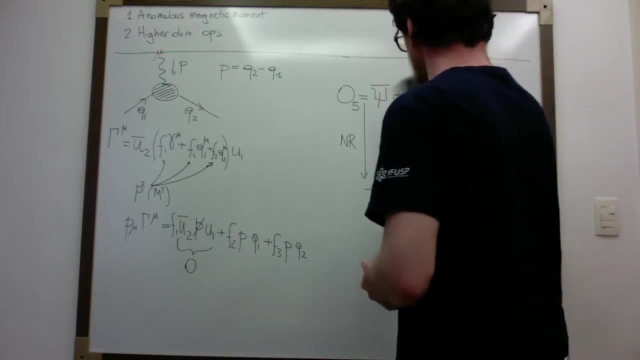 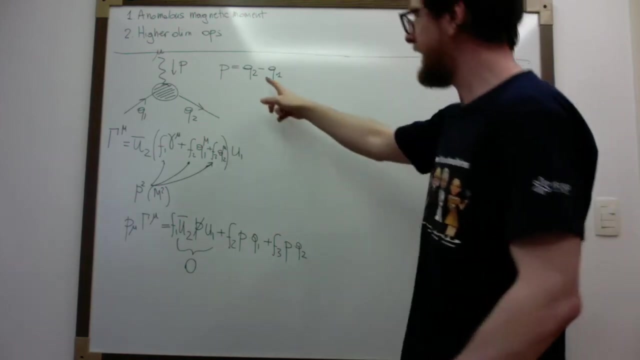 Well, if I try to compute these two scalar products, maybe I will have some idea of what's going on. So let's do it. Let's compute these scalar products, since they're very easy and very quick to compute. So to compute the scalar products, I will start from the conservation of momentum, this one. 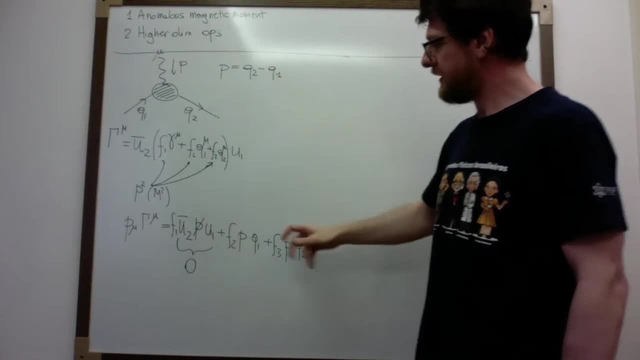 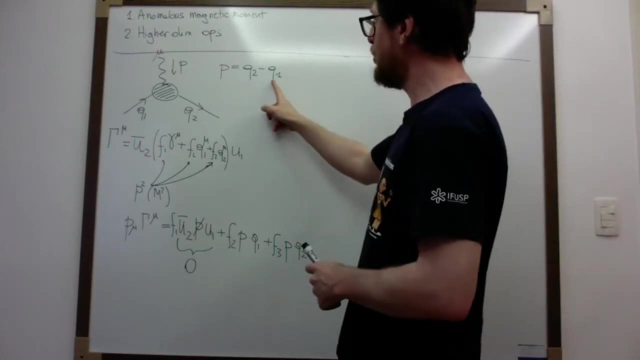 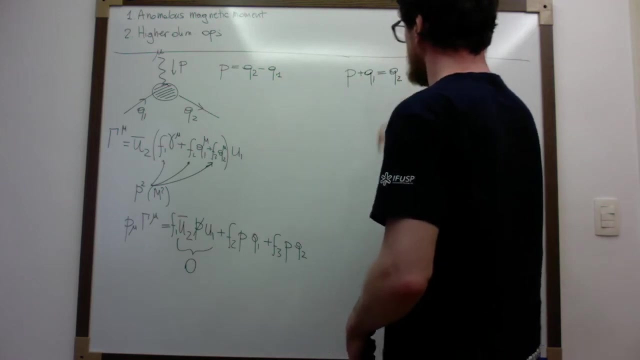 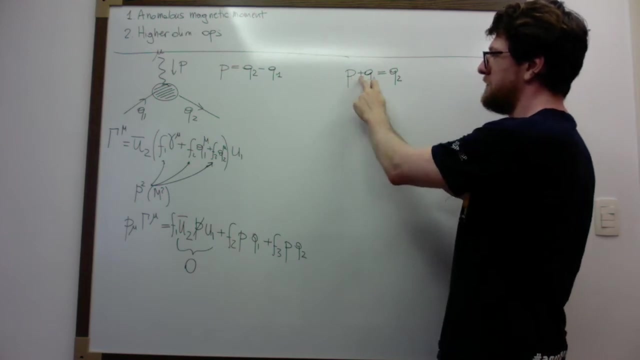 And then I will try to arrange the terms in such a way that this product actually appears and this other product appears. So let me first take q1 and put it on the left-hand side. So I'm going to write p plus q1, equal to q2, and then I'm going to square everything, because if I square everything here, I will get the product, which is p dot q1.. 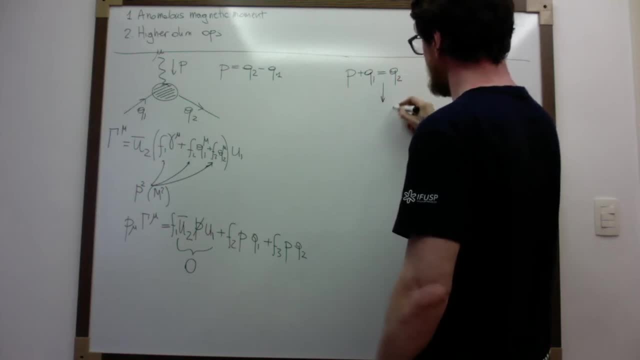 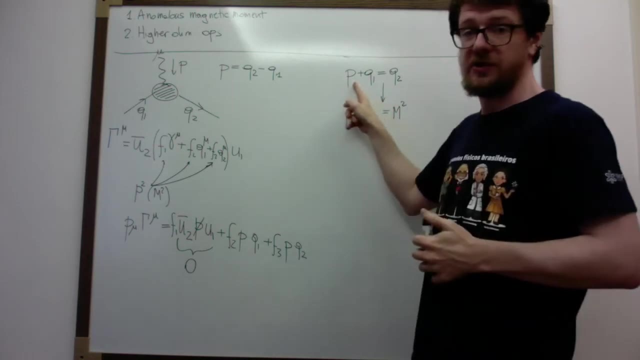 So when I square here, I get the mass of the particle, so it's capital M squared Here, I get p squared. Remember that the photon is not on shell, So this is not zero. p squared is not zero, it's simply p squared. 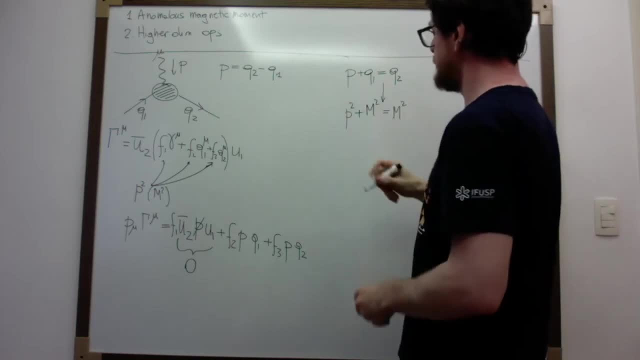 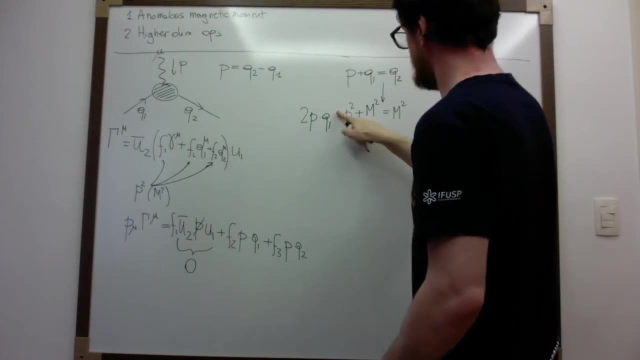 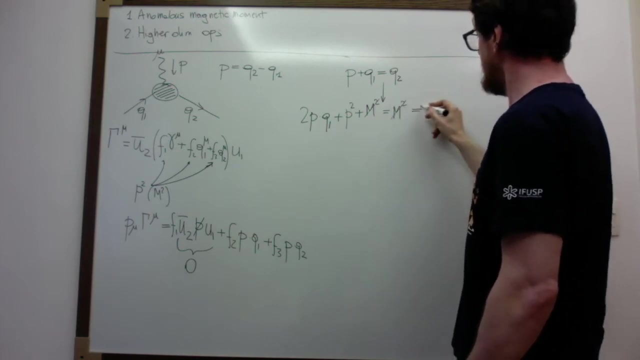 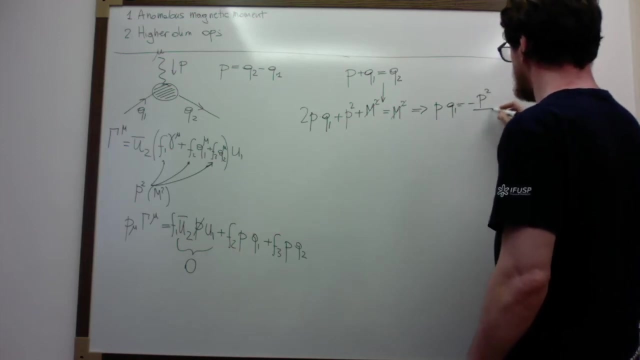 Then I have M squared, which is this mass here, and here I have the double product, which is what I want, this plus sign. So you see that this M cancels against this M, and what I get is that p dot q1 is equal to minus p squared over 2.. 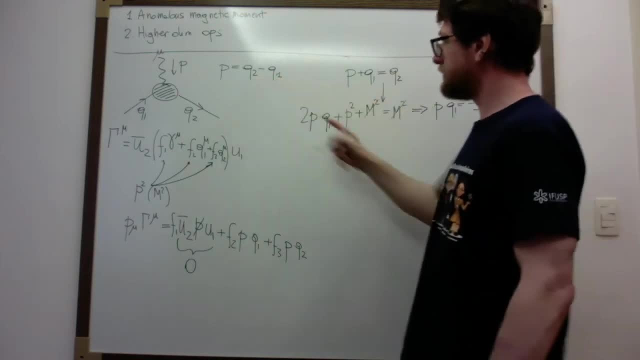 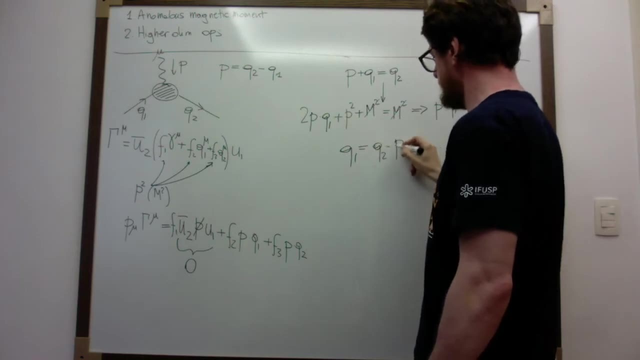 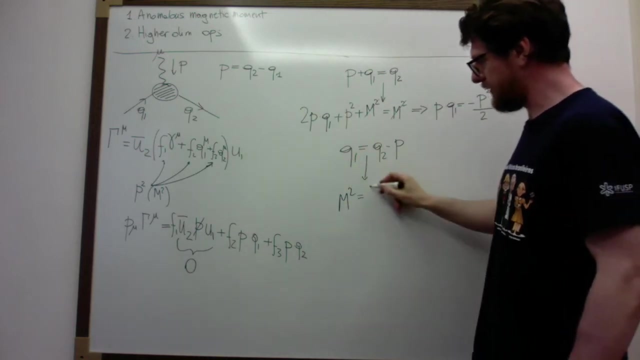 Okay, now let's play the same game with q2.. So when I play the same game with q2, I obtain that q1 is equal to q2 minus p. So again I square, I get an M squared from q1 squared, then I get another M squared from q2 squared, then I get the plus p squared from this and then I get the minus two times p dot q2.. 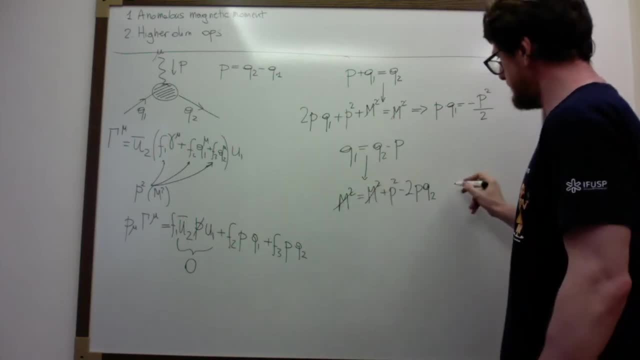 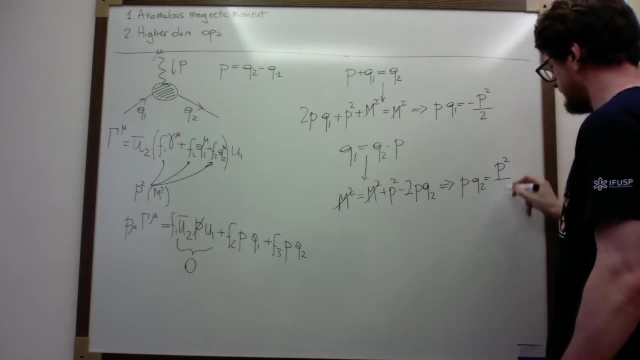 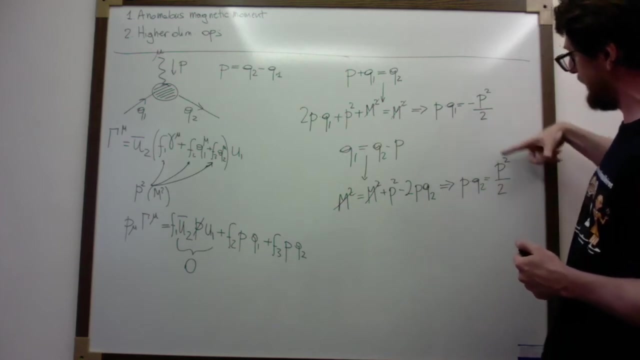 Okay. So again the mass is canceled in this process and I discover that p times q2 is simply equal to p squared divided by 2.. But this is a very nice result because you see the two scalar products are one minus the other. if you now compare the right and side, 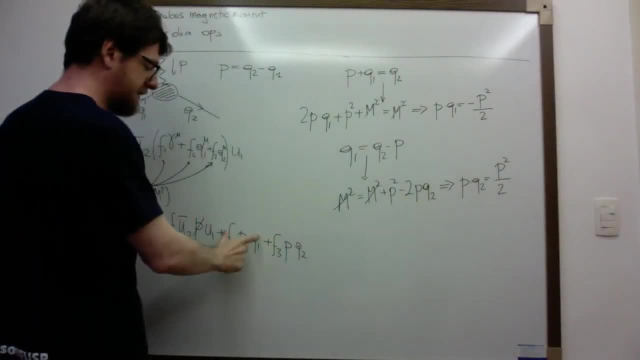 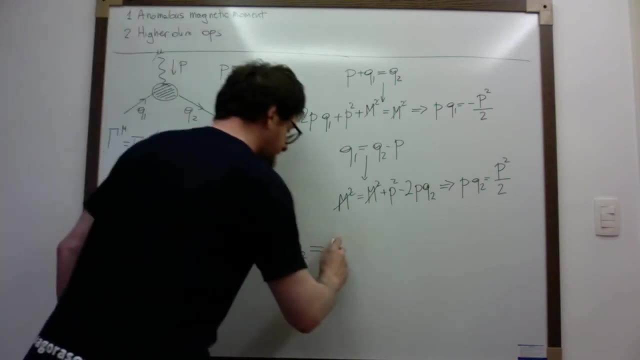 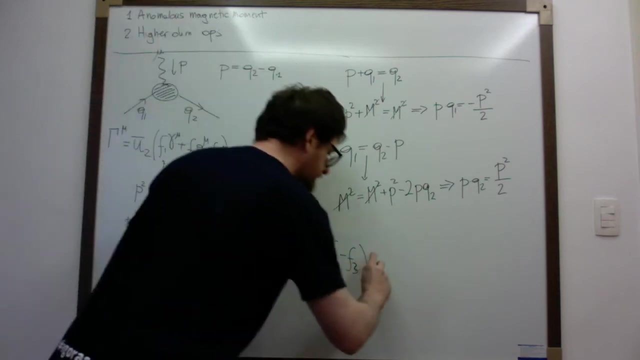 So this means that this term, as it is, is minus this one. Okay, So at the end of the day, this allows. This allows me to write the things in the following way: This is f2 minus f3, multiplying p dot q1.. 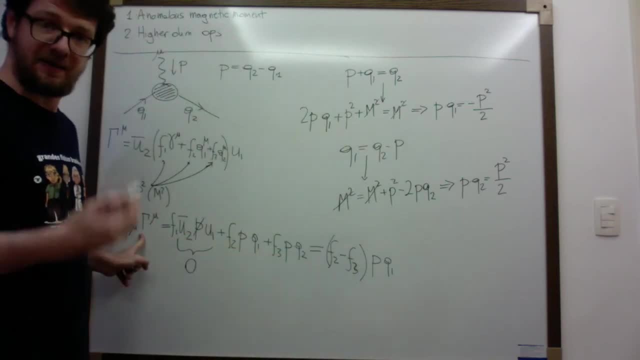 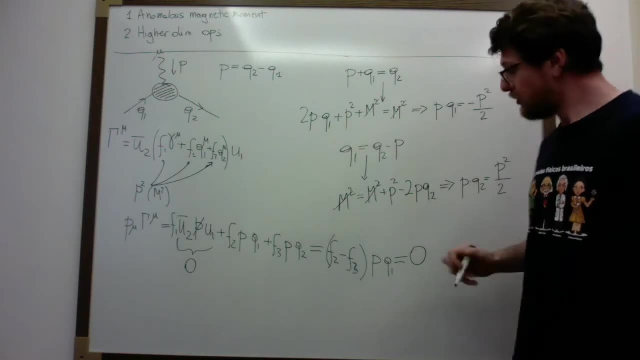 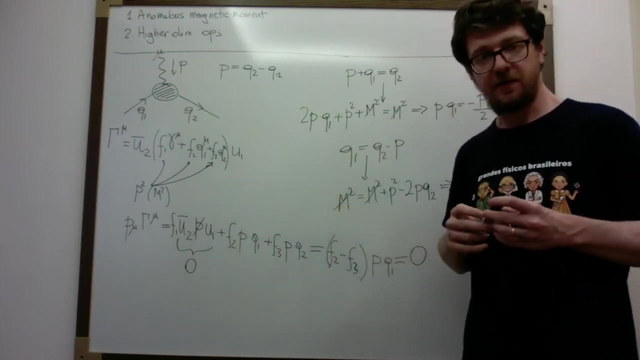 And since I want gauge invariance to be respected at all levels, in my theory this must be equal to zero. So you see immediately that f2 must be equal to f3 for gauge invariance to be respected. Okay, So, since we're constructing our theory in such a way that it is gauge invariant, we know that f2 must be equal to f3. 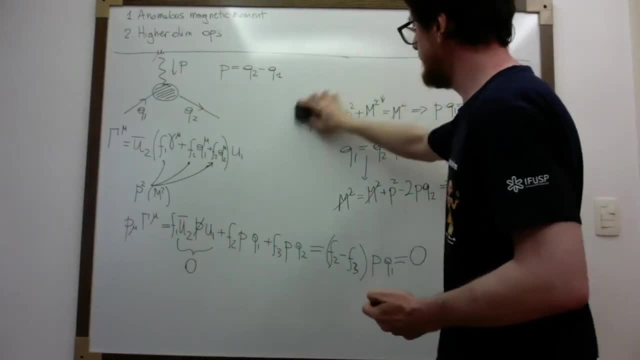 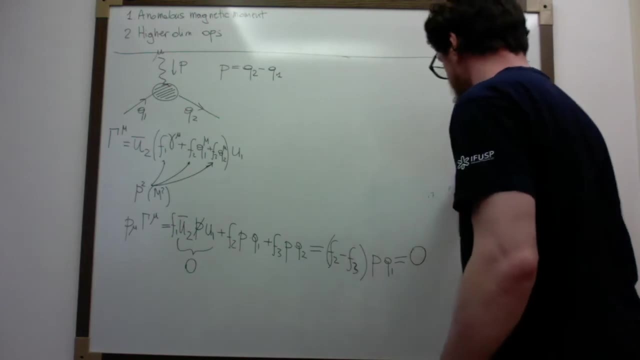 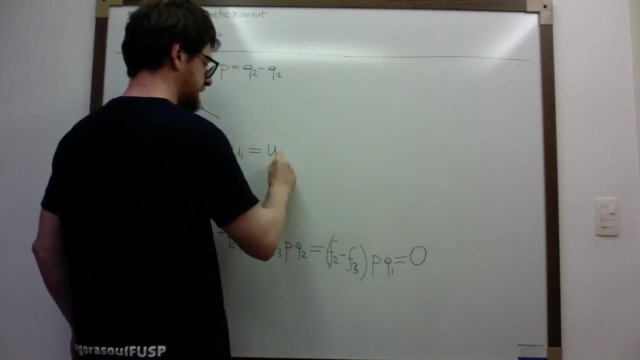 Excellent. So now that we have this information, so let me cancel these scalar products And let's go back to this expression and let's see what we can say. So let me rewrite this in the following way: This is u2 bar, f1, gamma mu. 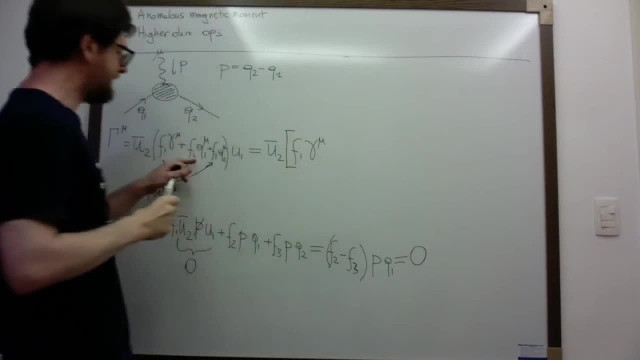 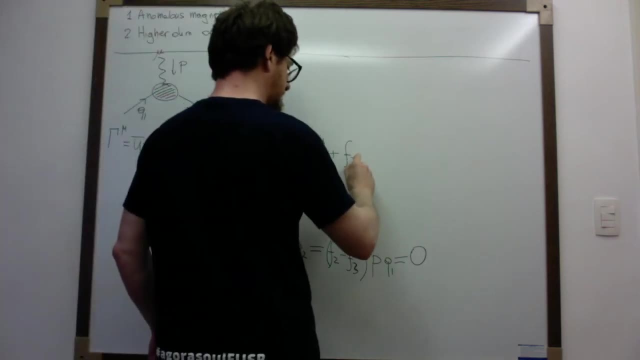 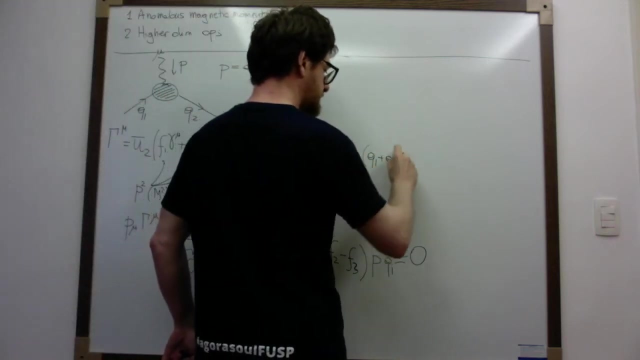 And now we take into account the fact that f2 and f3 must be equal because of this condition. So here I will have plus f2.. And then I get the sum of the two, for a moment q1 plus q2, mu, all multiplied by u1.. 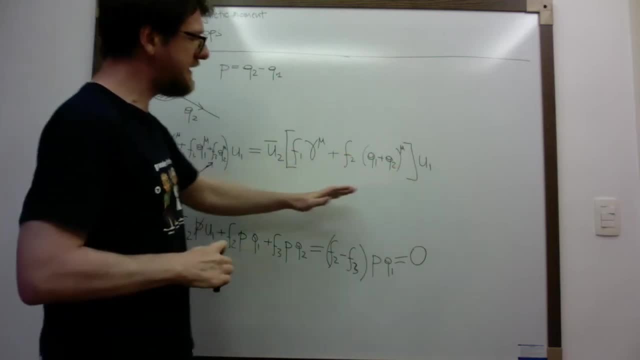 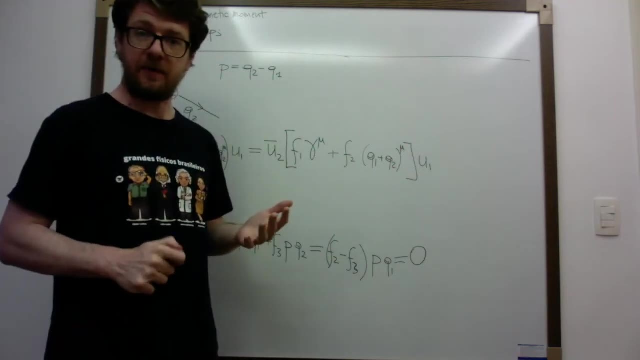 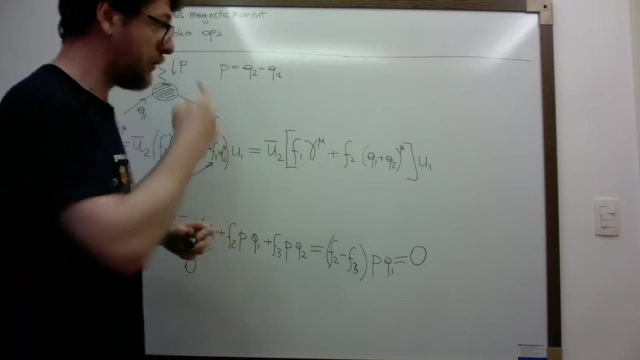 Right, Very good. So it seems that this is the most general form of this vertex that I can have. Actually, I can do something else. Okay, I can do. I can take one step, the computation one step further, because there is a very nice identity which is called Gordon identity. 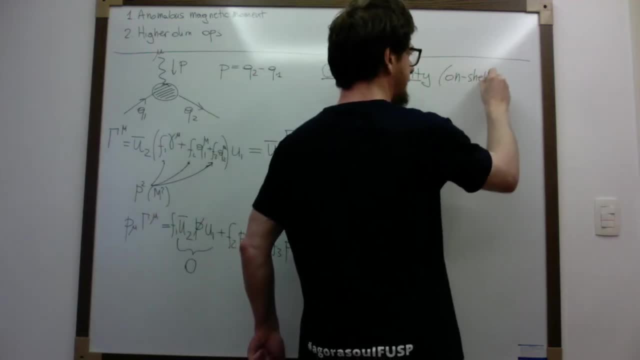 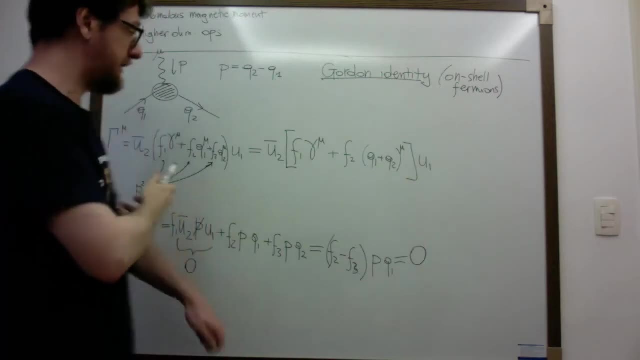 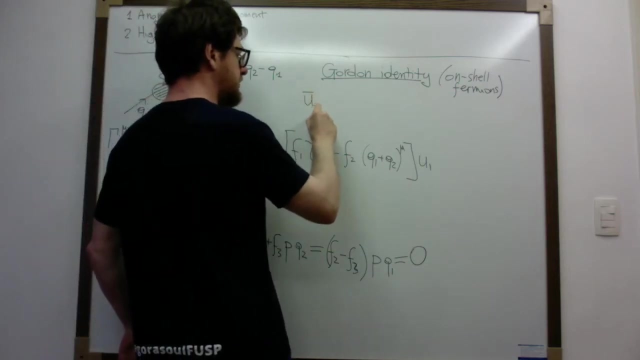 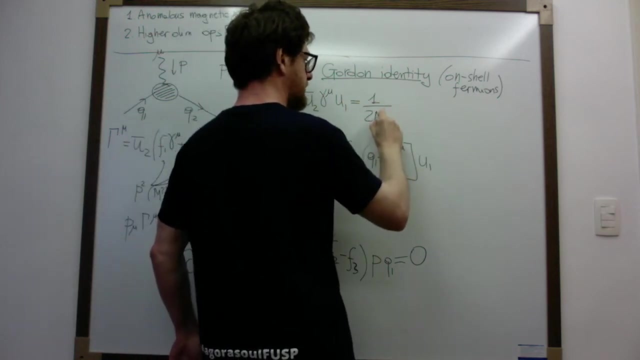 Which is valid for on-shell fermions. So exactly the situation we are considering. Remember that these two fermions- I took them to be on-shell And the Gordon identity tells me the following: So u2, gamma, mu, u1 is equal to the following expression: 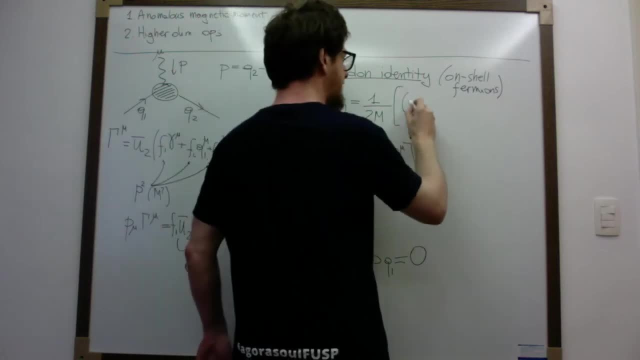 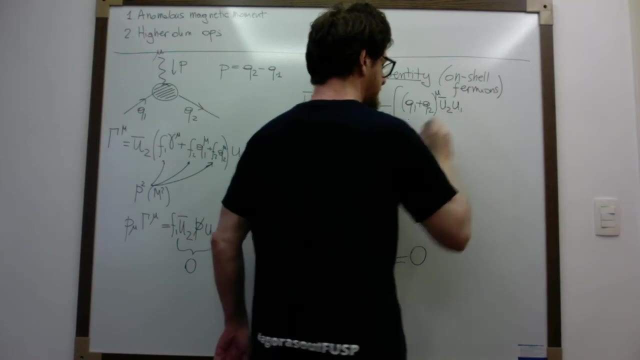 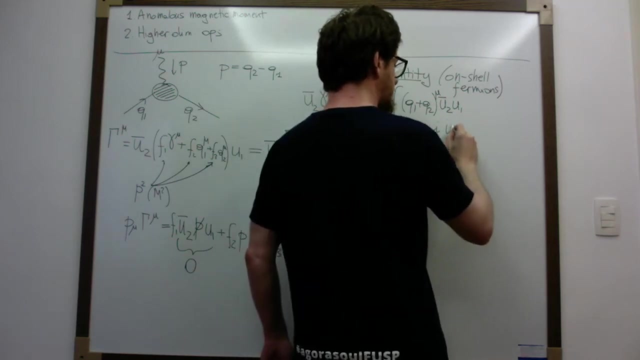 I divide by one over two times the mass, Then I get here the sum of the momenta That multiplies e2 bar u2 bar u1.. And then I get the plus i: u2 bar sigma mu, mu, u1 p mu. 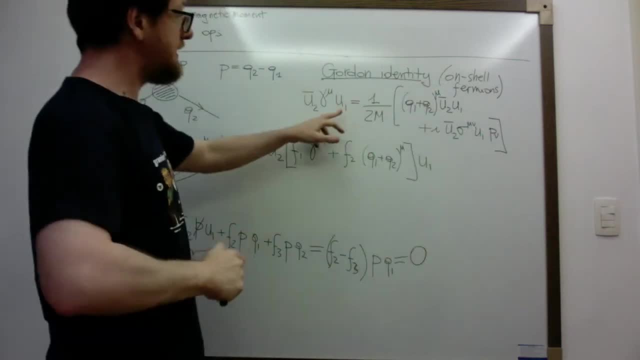 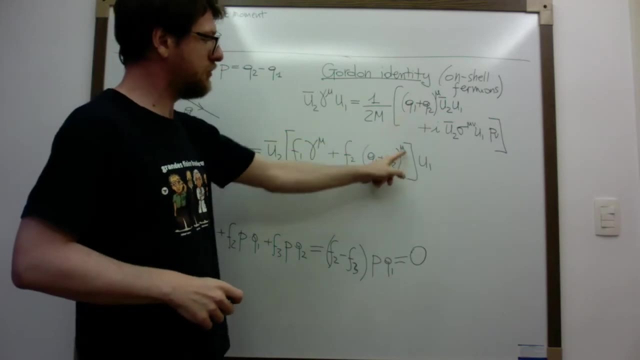 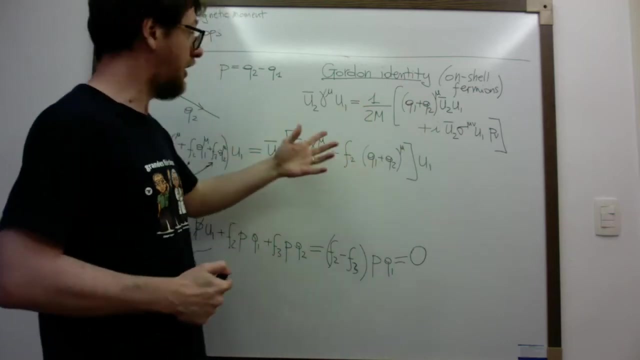 Okay, this is the Gordon identity. So you see immediately that I can use this Gordon identity to simplify this factor of q1 plus q2, mu, u2 bar u1.. And write all, and write this vertex simply in terms of gamma mu. 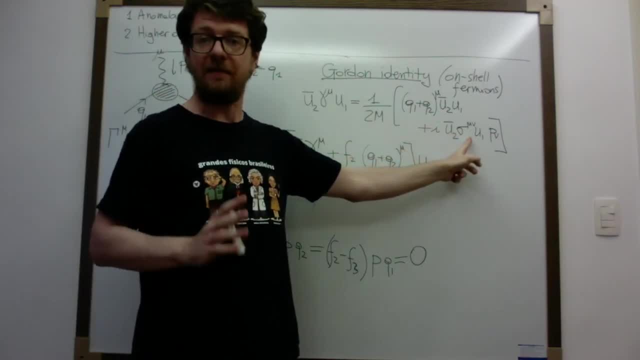 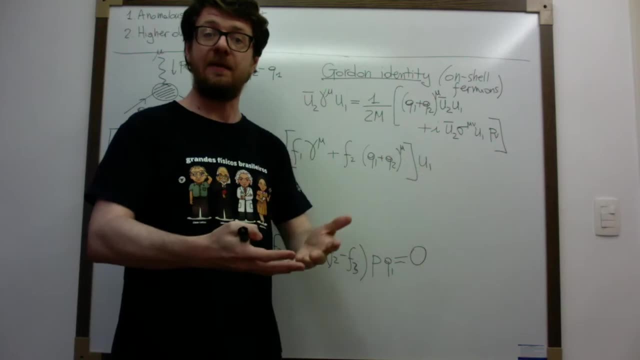 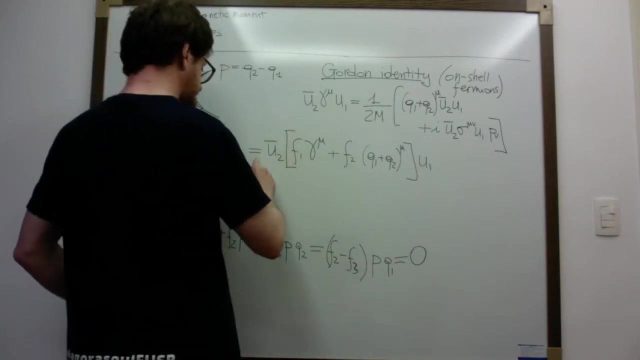 And sigma mu mu. Remember that I want to obtain something proportional to sigma mu mu, Because I know how to connect directly to sigma mu mu With the coupling between the spin of the fermion, the electron and the magnetic field. Okay, so, at the end of the day, this coupling, this vertex, will be written in the following: 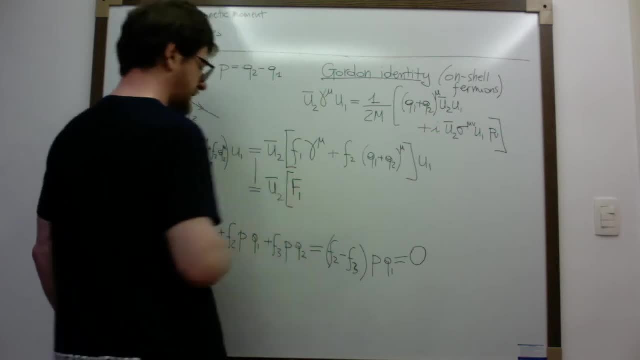 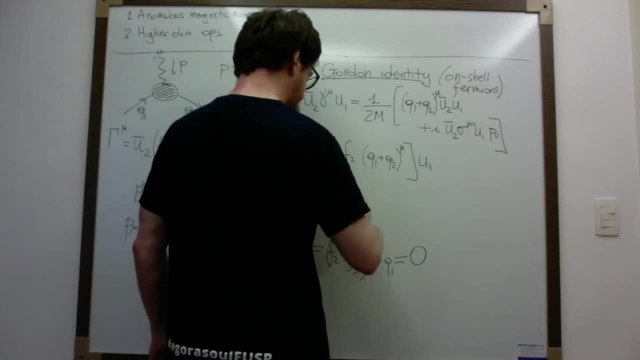 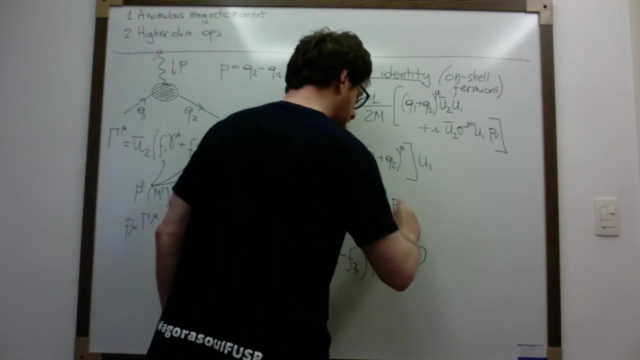 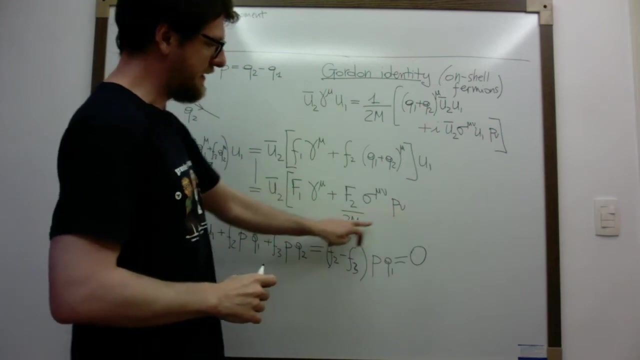 There will be some factor here which is traditionally called f1.. Then multiplies gamma mu, And then I'm going to have another factor which is called f2. Then multiplies sigma mu, mu, p, mu. Okay, and traditionally we divide here by two times m, in such a way that the dimension of f1 and f2 are the same. 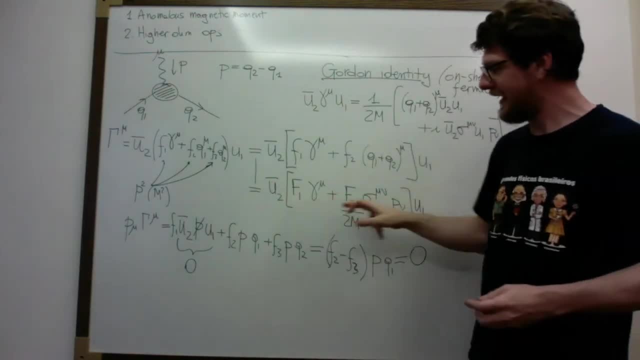 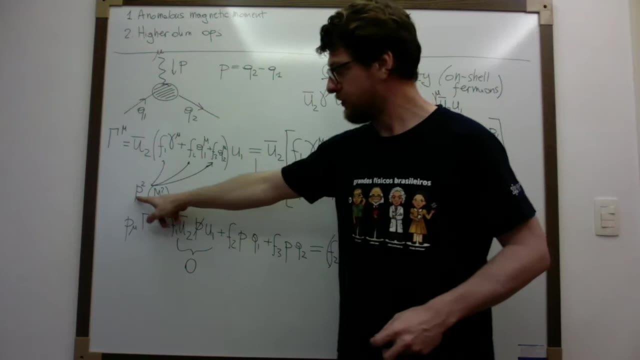 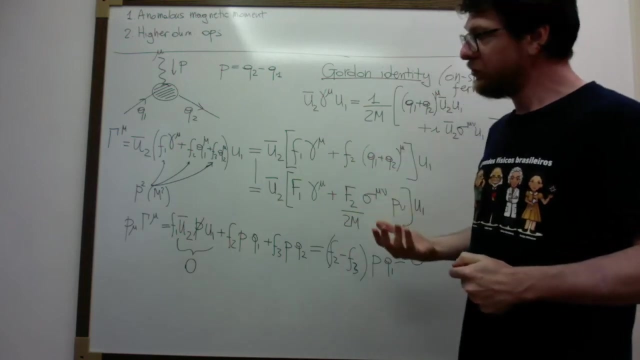 And then this is u1.. Okay, this f1 and f2 are combination of these small f1 and small f2.. And they are themselves Functions of p squared and of the mass of the electron. Okay, so what we're going to do in two minutes is to take this, open it up in one loop. 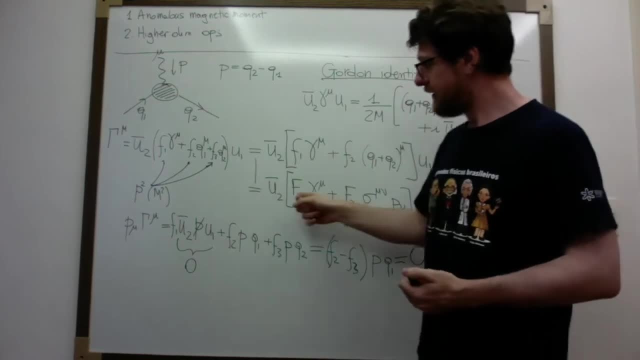 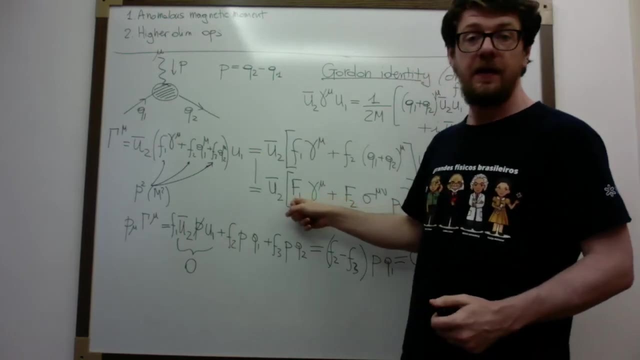 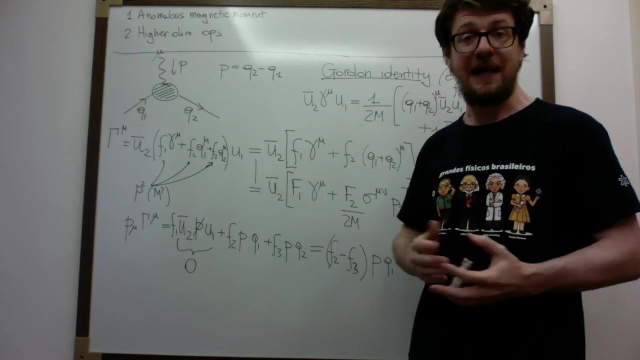 And actually do the computation Okay and see that both f1 and f2 are generated. Now I won't bother writing down f1. Because I can always consider this f1 as fixed by the Renormalization condition that fixes the electric charge. 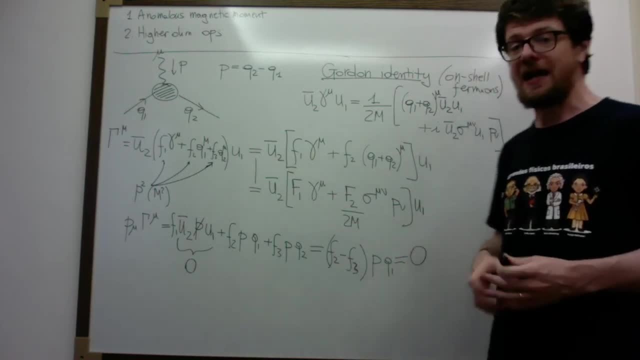 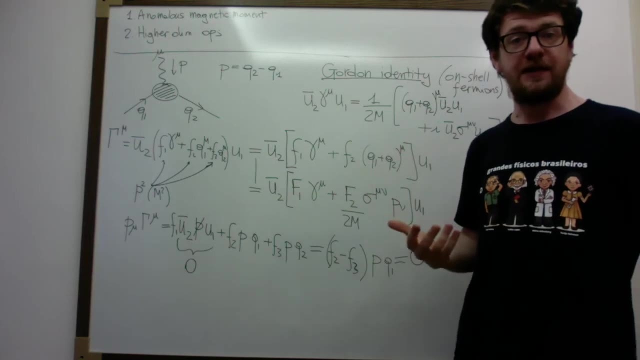 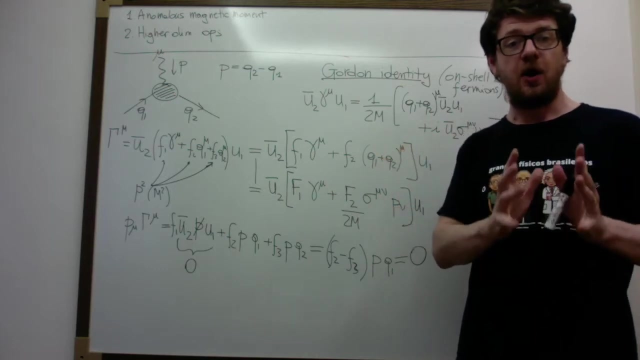 Okay, we didn't see the renormalization of the electric charge from the point of view of the vertex Because, if you remember, when we were discussing the running, the renormalization of the electric charge, what we did was to redefine our photon field and transfer all the effects on the photon propagator. 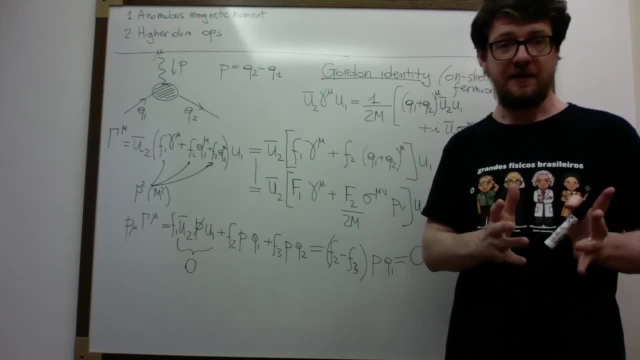 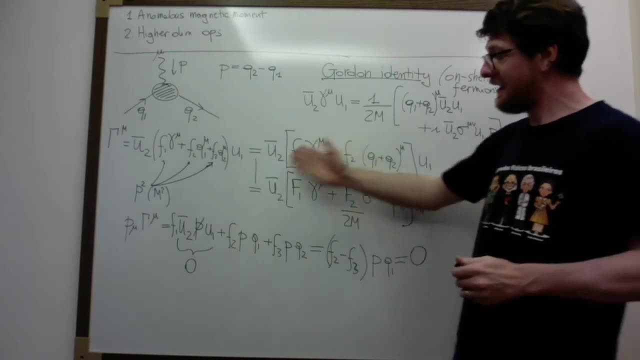 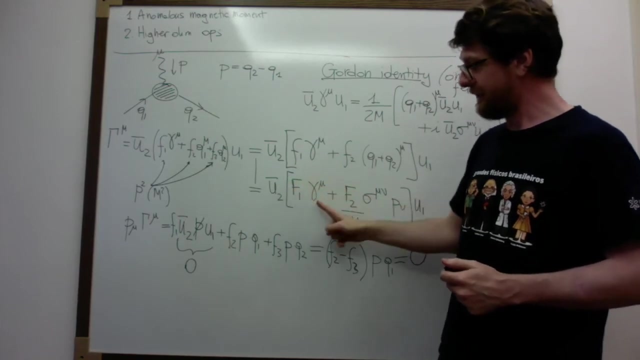 Of course, nobody forces you to do as we did, So you can keep the electric charge, Okay, In front of your vertex, And then in that case, if you do that, the renormalization condition will emerge as conditions on the loops that are proportional to gamma mu. 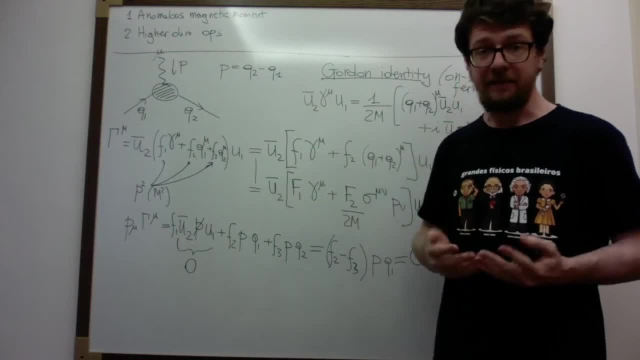 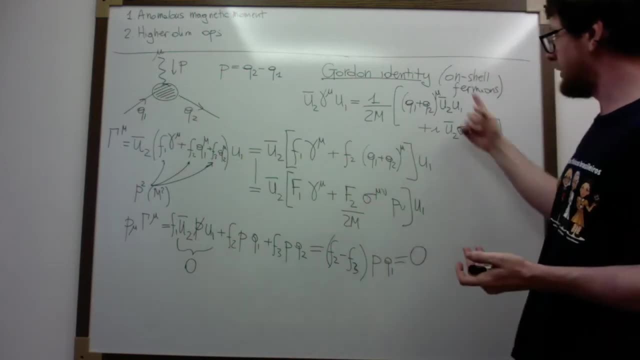 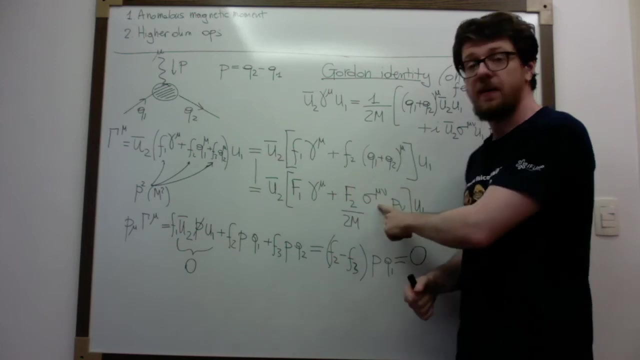 Okay. so the strategy is clear. We're going to open this up in one loop. We're going to see, we're going to use, if needed, a golden equation to put the vertex in this form, And then we're going to just consider the term proportional to sigma mu. 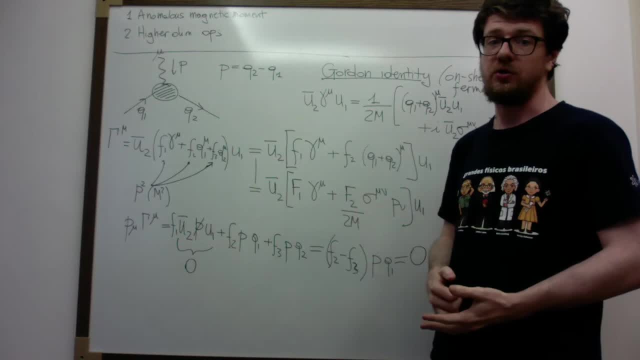 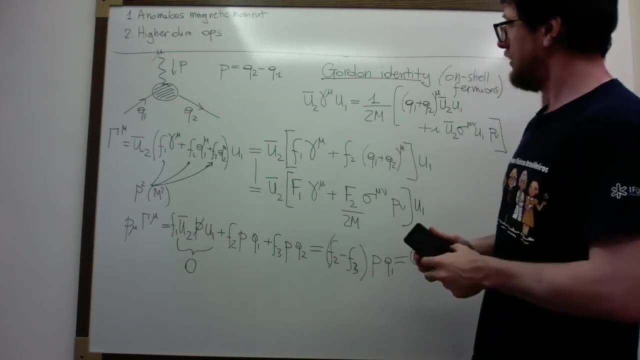 Because the other one will simply enter the renormalization of the electric charge, which is something that we're not interested in today. Okay, So I won't do the computation, but I will show you the design, So let me cancel here. 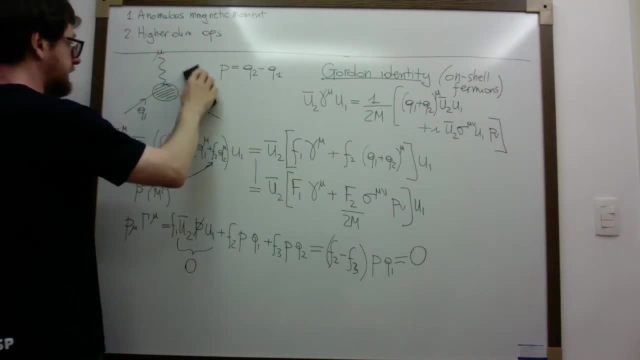 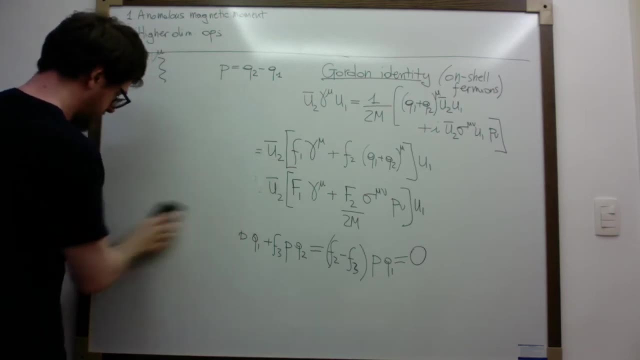 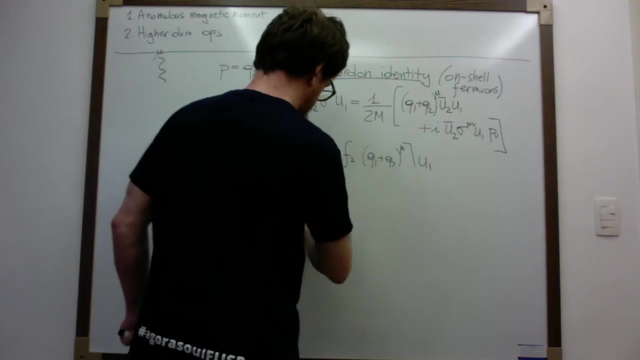 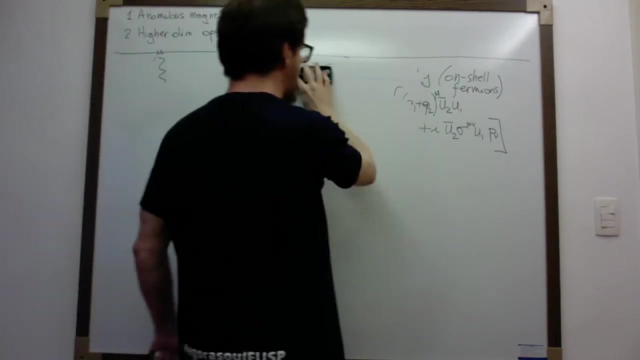 And let's write down the Feynman diagram with the loop which will give us The effect that we want. So of course there are many one loop diagrams that you can think about that should compose that vertex, The one particle reducible vertex. 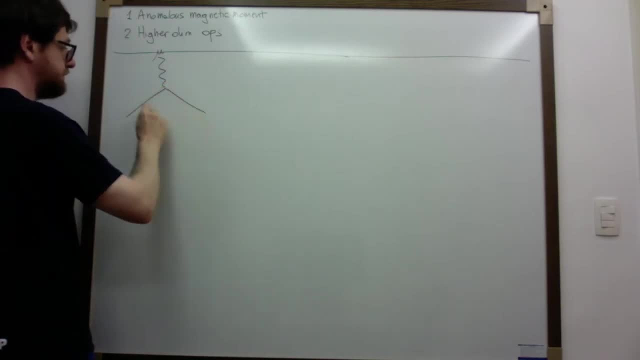 But at the end of the day, the only one that matters is this one: Okay, So this is Q2.. This is Q1. And here I am exchanging the Okay. So this is a loop diagram. You see, this is one particle reducible. 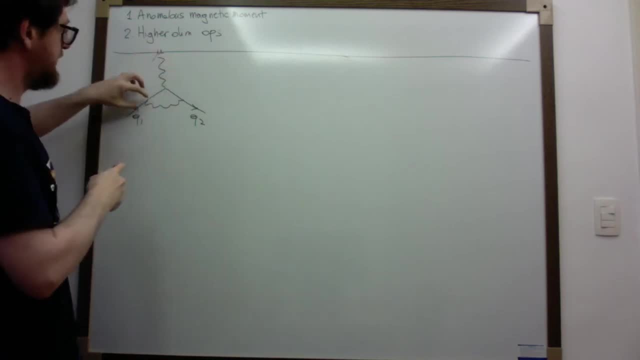 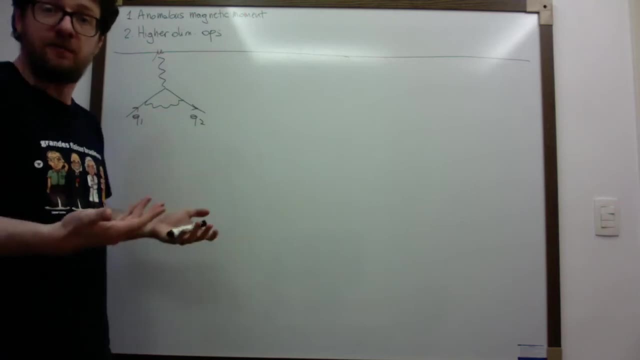 Then you can also think about putting corrections here, here or here. Okay, These are not one particle reducible, So we should consider them somewhere else. But even if you do consider them, you discover that actually the only contribution that they give is proportional to gamma. 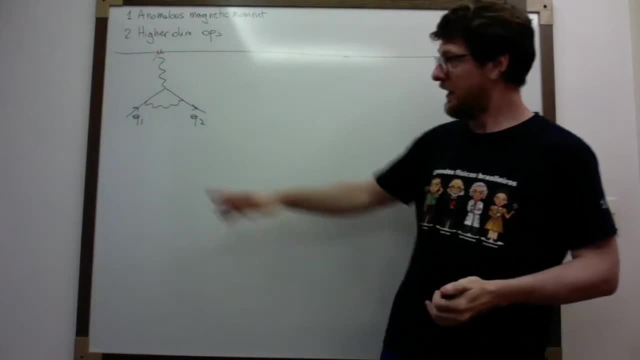 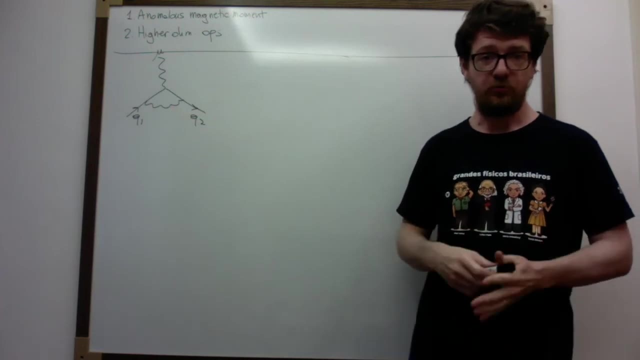 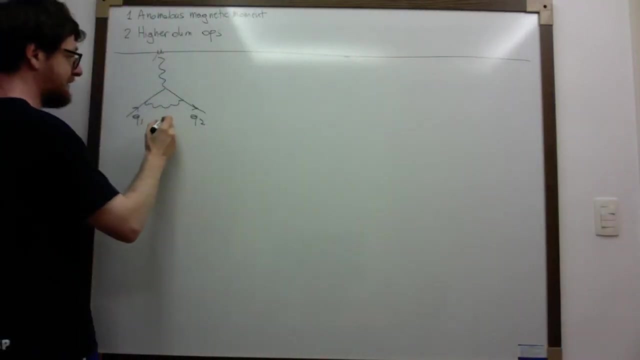 They won't generate any contribution proportional to sigma mu. Okay, So this diagram here is precisely the diagram that we need To compute the sigma mu nu. Okay, So let me just write this amplitude for you to have an idea. So let me say that the momentum of the photon here is called Q. 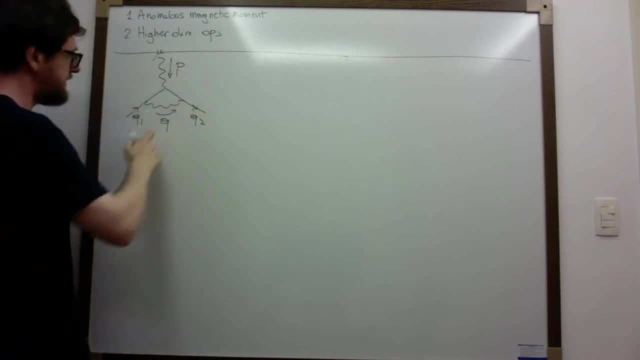 So this is momentum P of the photon. So, if this is, if this is Q, you see that this, this momentum here, must be Q2 minus Q And this momentum Here must be, uh, Q1 minus Q. okay, 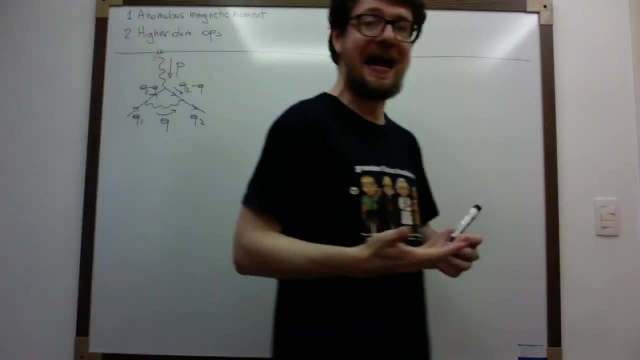 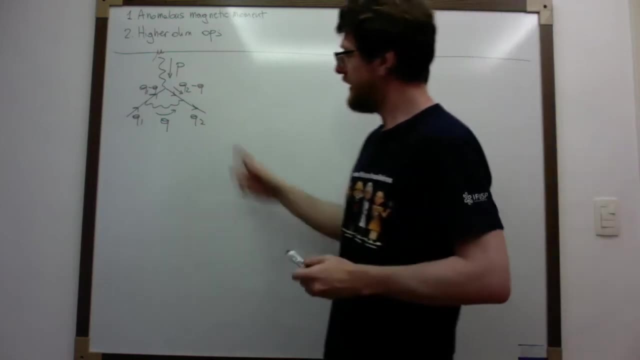 You can order it as you like. The result won't matter. It's completely arbitrary how we fix this, the routing of the momentum, So it really doesn't matter. So let's start. Okay, As usual, we start from the outgoing electric. 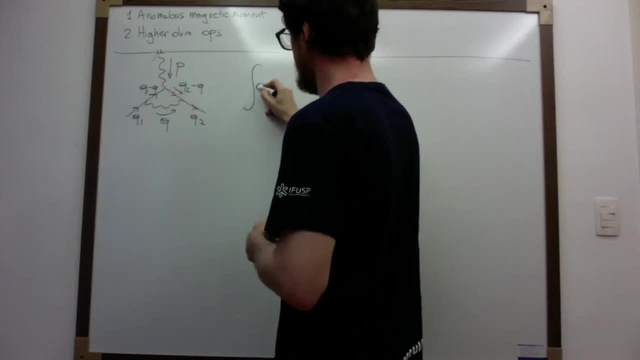 So first of all, there is a loop, So let me already write the integral over the. So this is an integral over Q. Q is the momentum flowing into the loop divided by two, pi to the fourth. Okay, Then we start from here. 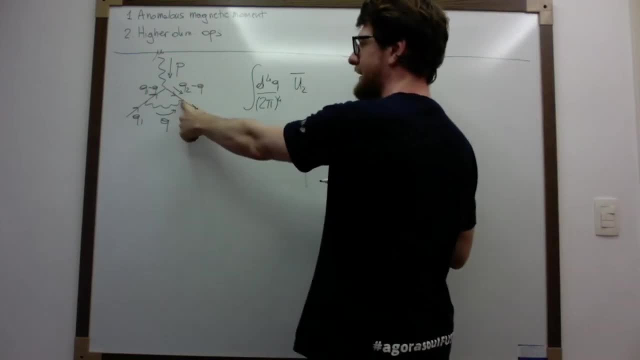 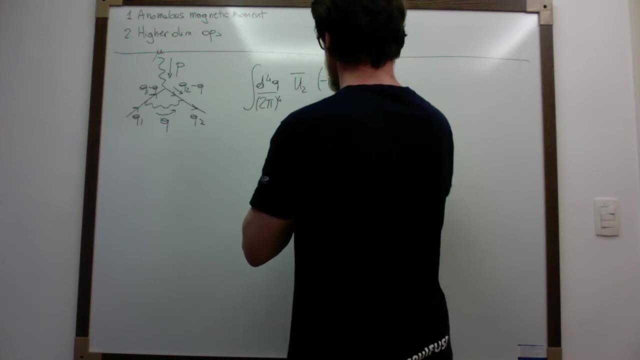 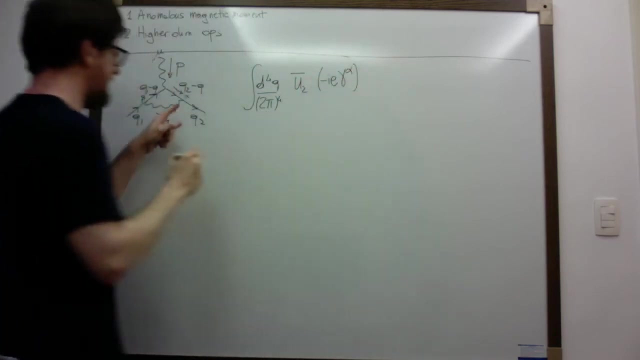 So this is a U2 bar. Then I get to this point and they have an electromagnetic vertex. So the electromagnetic vertex is going to be minus. I E gamma. Let me say that this is alpha. So this is gamma alpha. Okay, So we are here. 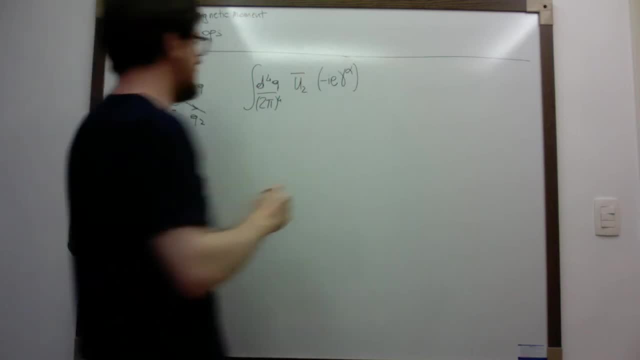 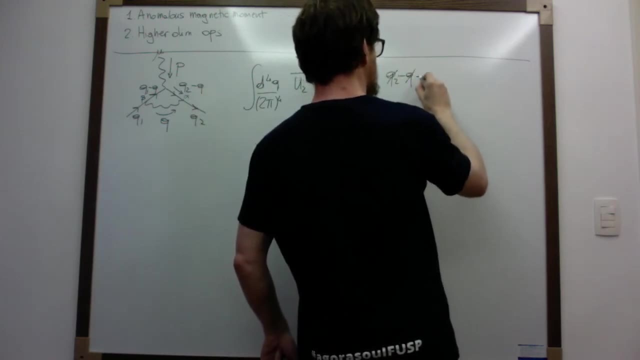 Then we have a propagator, because we have an Electron propagating here. So the propagator is I, Q2 slash minus Q slash plus the mass of the fermion, Everything divided by Q2 minus Q square, minus capital M square. Okay, 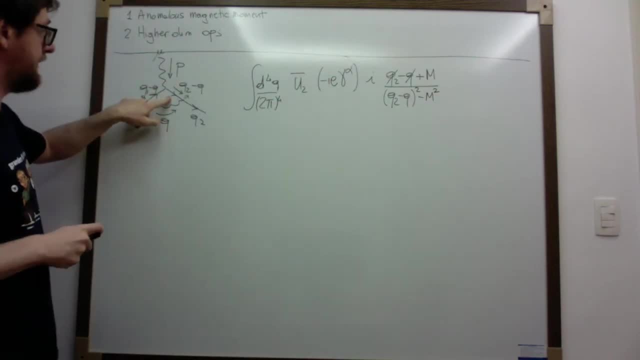 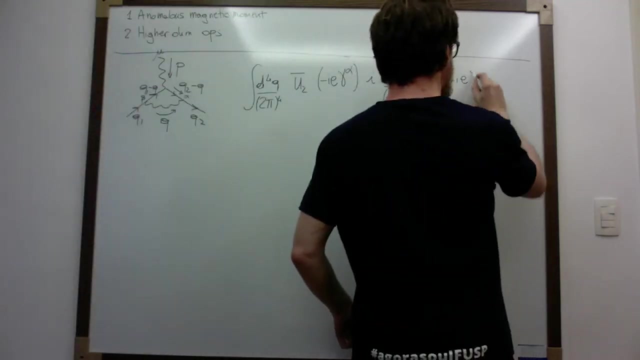 And this is this propagator. Now, if I go backwards and I continue, I get to this other final vertex Right, And this one will have index mu, which is the standard index of the fault. So here I will add minus I E gamma. 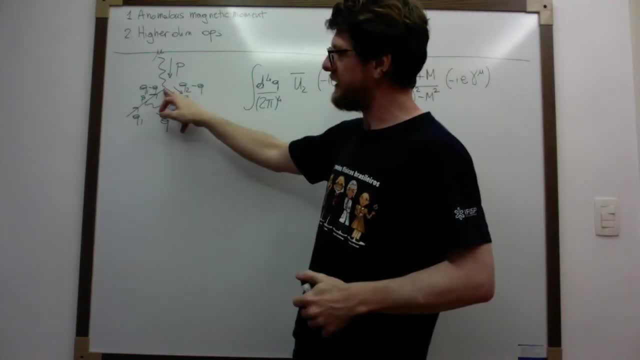 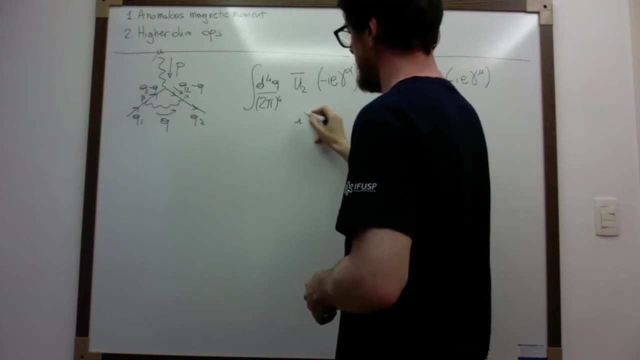 So we are halfway through, So we started from here. We are at this point, So now we need to put here the propagator of these, these other propagators of the electron. So this is- I continue down here. I Q1 slash minus Q slash plus capital M divided by Q1 minus Q square. 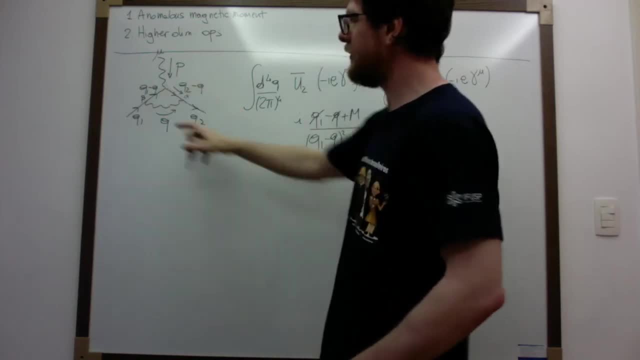 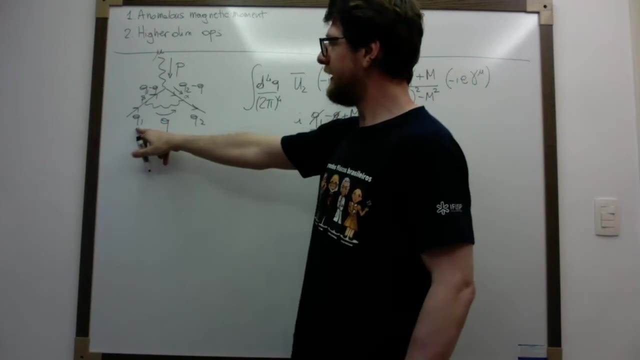 And this is the propagator. then I get to this other vertex, and this is minus E gamma beta, And then here I have the external fermion. So I don't have propagator, but I have the wave function, which is U1.. 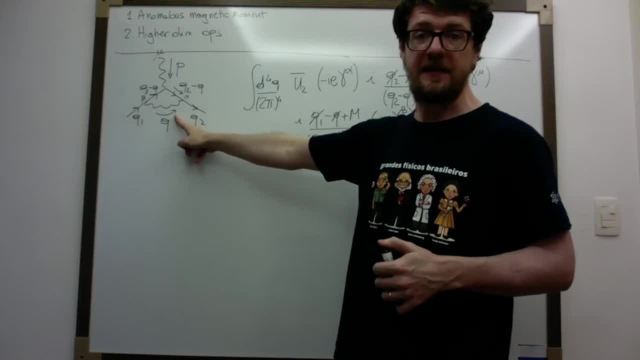 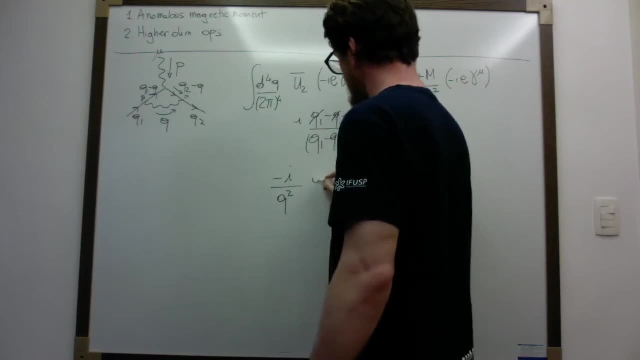 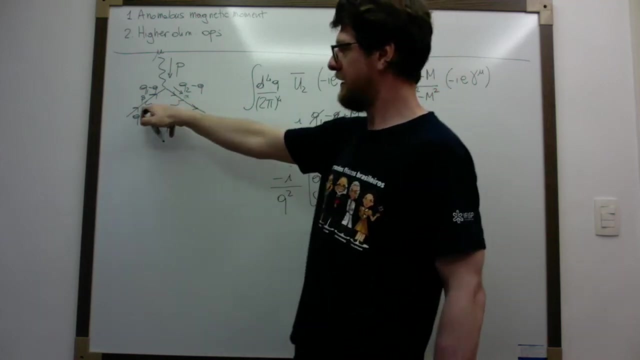 The only thing that I'm missing here is the fact that also the popup is propagating here inside the loop. Okay, So the propagator is minus I divided by Q square, And here I will have G Alpha beta. So I use alpha beta because the photon is propagating between these two vertices, which have the Lorentz index equal to alpha on the right and beta on the left. 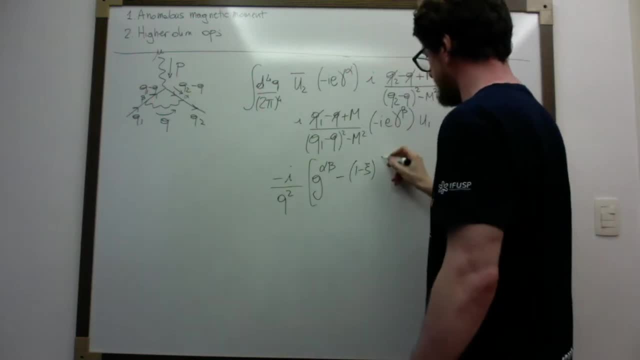 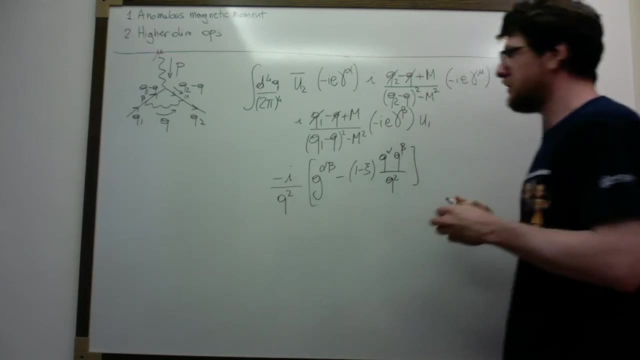 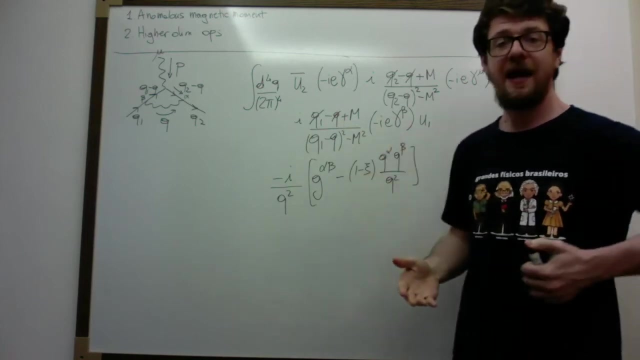 And then I have the term, which is the gauge choice, and it's Q alpha, Q beta divided by Q square. Okay, So I won't do the computation. This is something that, for instance, you can put inside package X and let him do the computation, or you can sit down. 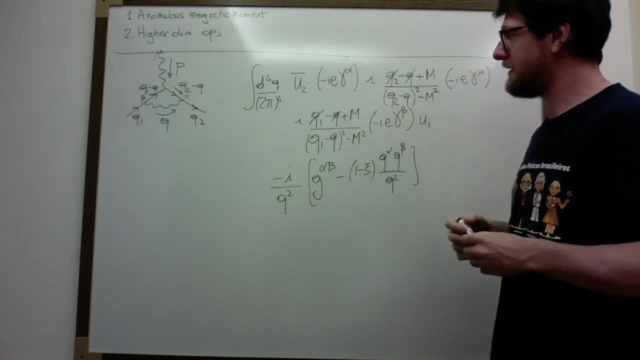 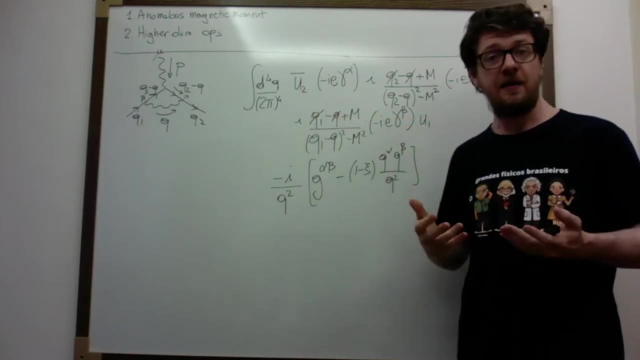 And really open up all the algebra of the gamma matrices. Okay, There are some simplifications that emerge because this U1 and- sorry, this U2 bar and U1 are on shell, So you can, you can simplify some of the terms. 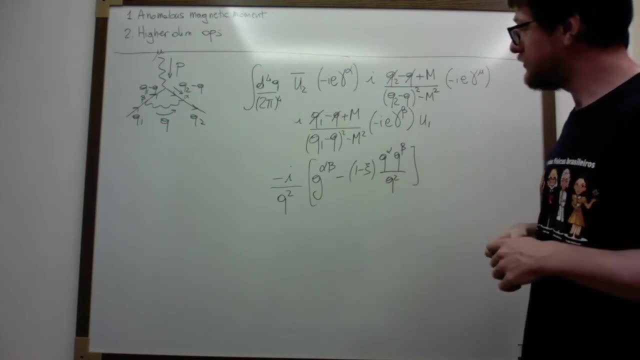 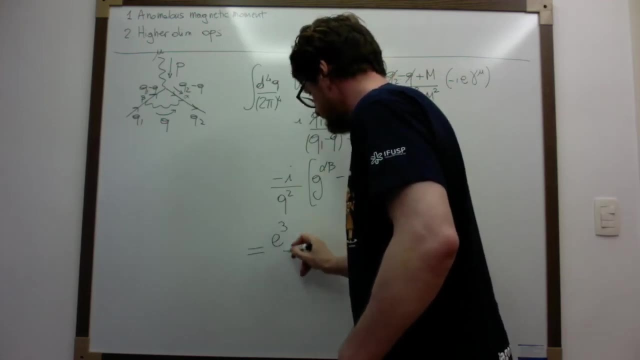 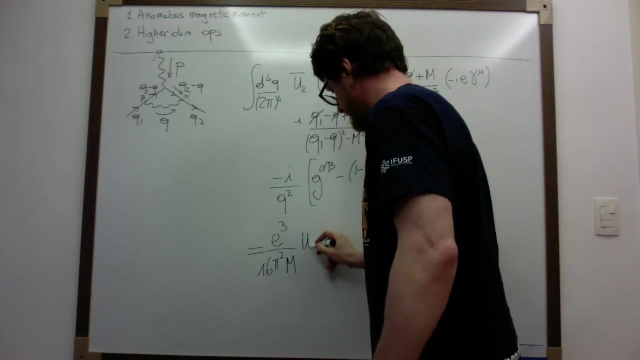 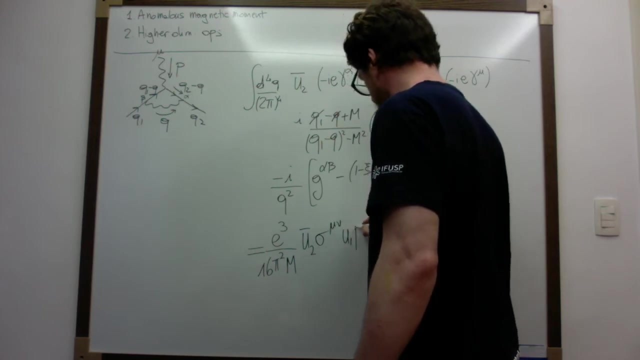 Okay, At the end of the day, after you do all this computation, you obtain the following result: You have an E cube, You have a 16 pi square M, U2, bar, sigma, mu, mu, U1, p, mu, plus terms which are proportional to gamma. 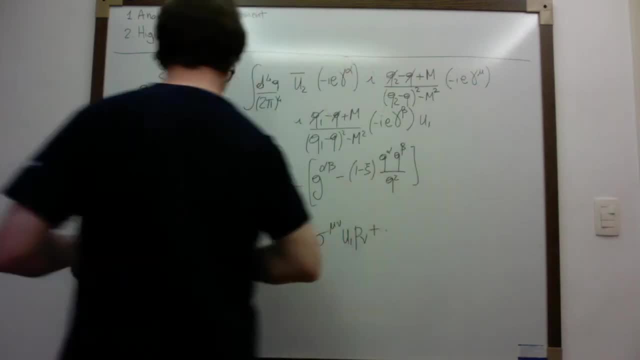 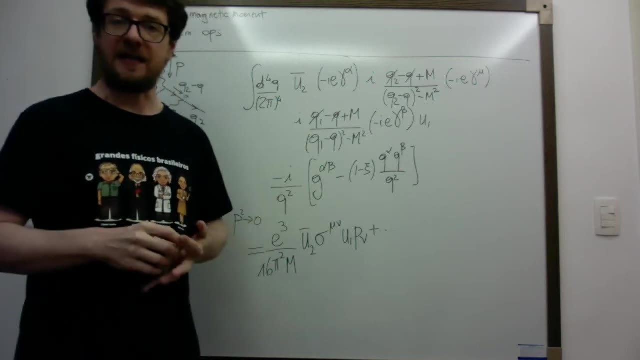 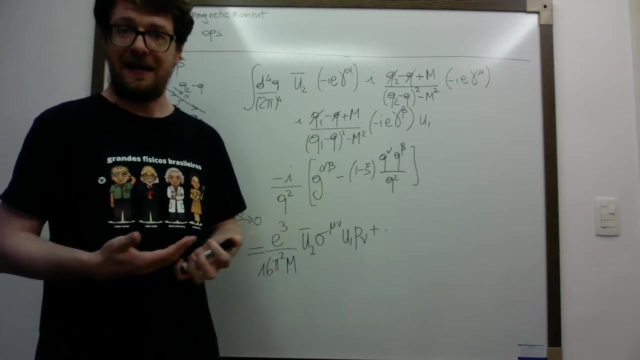 Okay, So in passing from here to here, I took the limit P square going to because, remember that something that we said in this lecture is that we measure the non relativistic, Then we measure The electromagnetic coupling in the non relativistic regime. 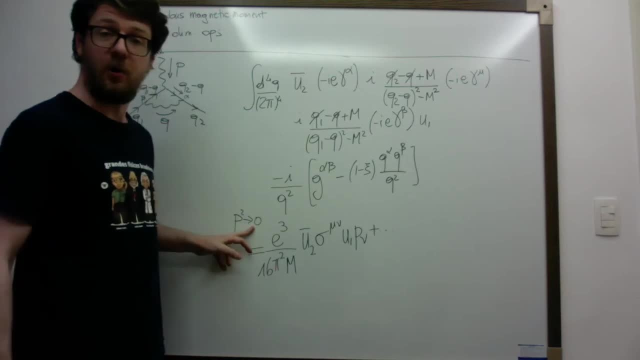 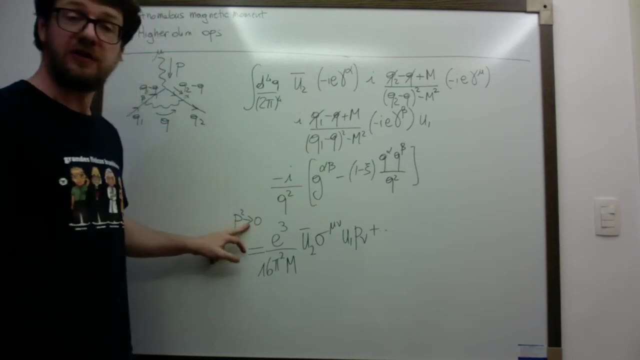 Non relativistic regime stressorize the amounts to have very small energies that are. So I can take the P square going to zero limit. If you do not take this P square going to zero limit, then this object here will be much more complicated with the P square dependence. 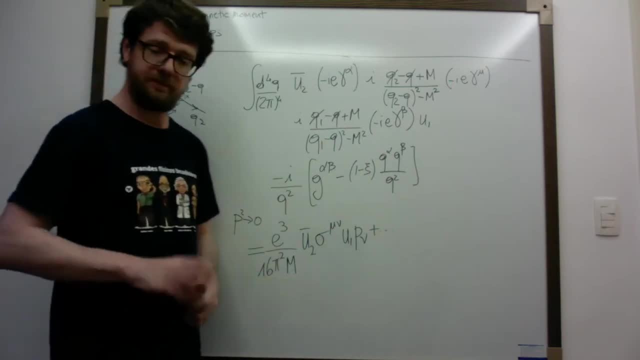 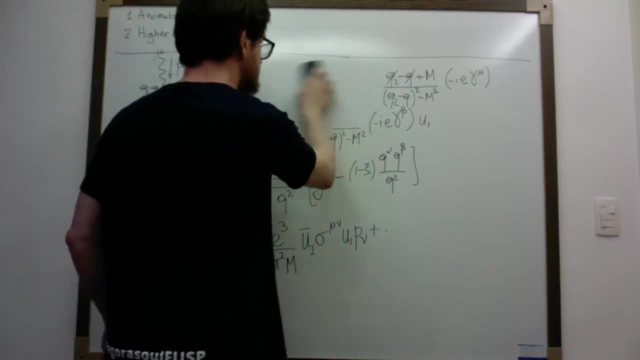 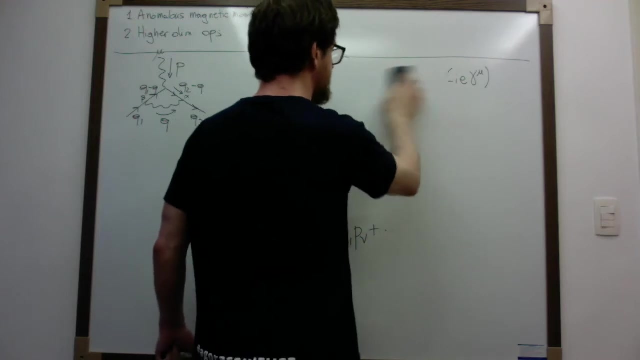 But that's not what we need. Okay, Zero energy: This is the contribution, and that's- and this is the crucial part. Okay, So let me Cancel here And I will just rewrite this result, because now, from here, We are going to. 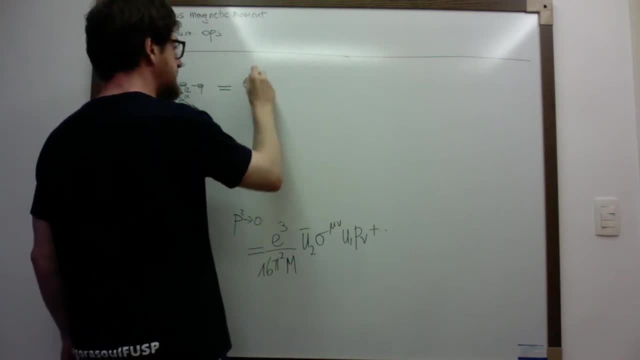 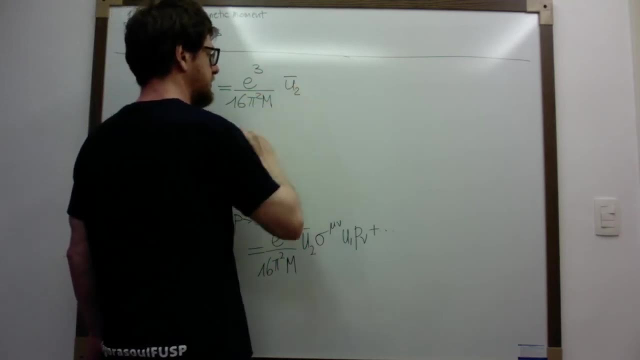 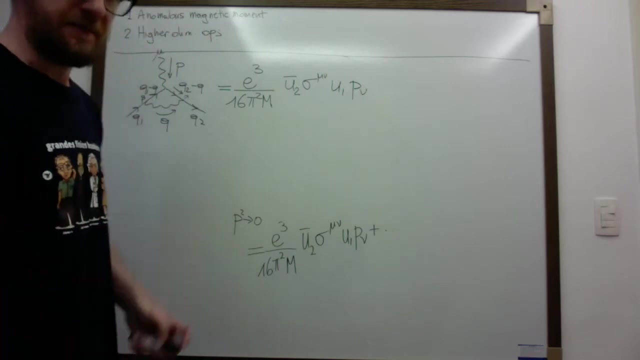 Deduce what is the anomalous magnetic. So this is E cube divided by 16 pi square capital M, And then we have U2 bar, And then we have U2 bar, sigma mu nu, U1 pi 2,. okay, excellent. 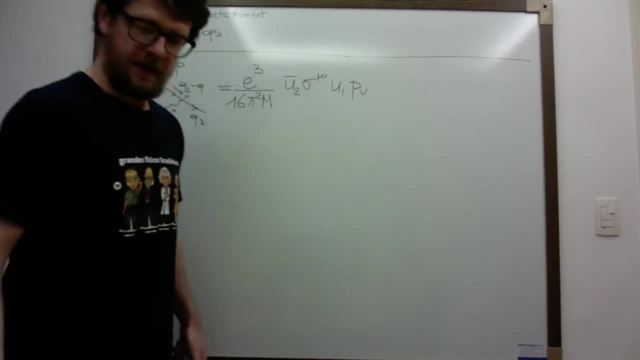 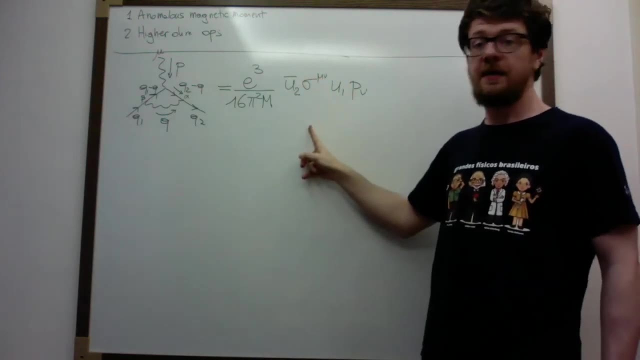 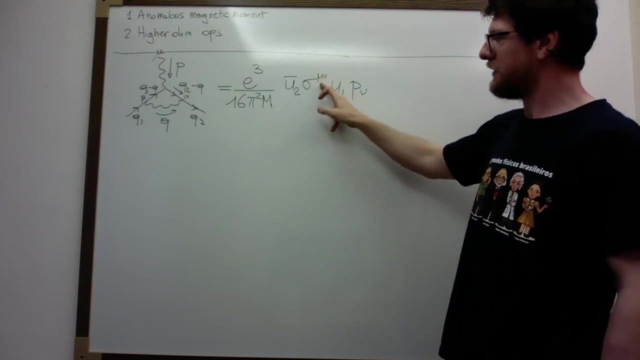 So we're almost done. The only thing that we need to understand now is: this is a matrix element, So what is the operator that corresponds to this matrix element? So the operator, you see that it's it's obvious That you must have. 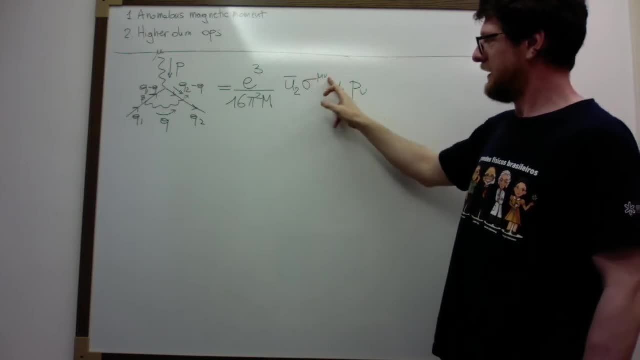 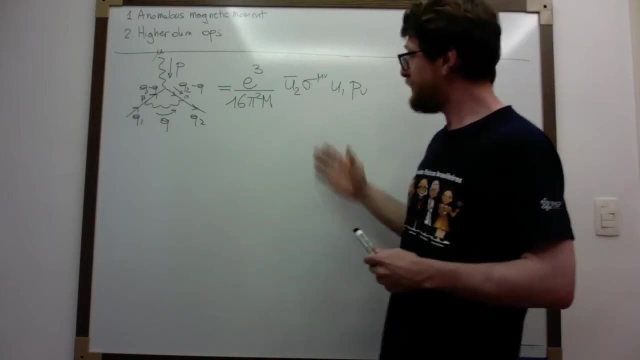 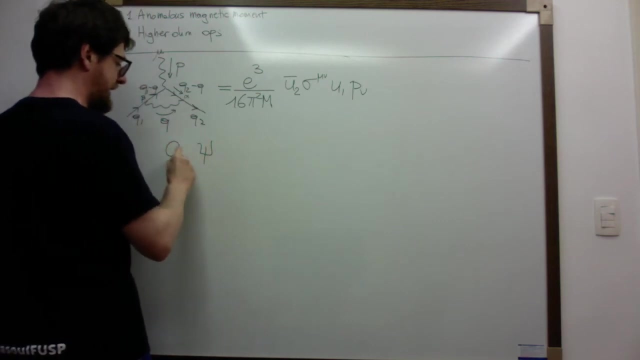 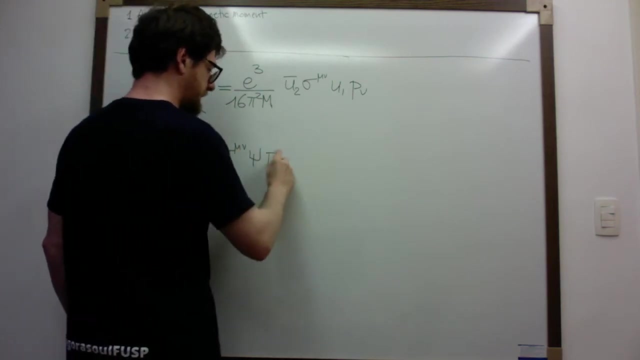 Some, uh, some. you must be connected with the one that we were discussing with the sigma matrix. Okay, If you think a bit about it, let's go back to that operator, what we call it before. So this was sigma bar, sigma mu nu, psi and mu nu. 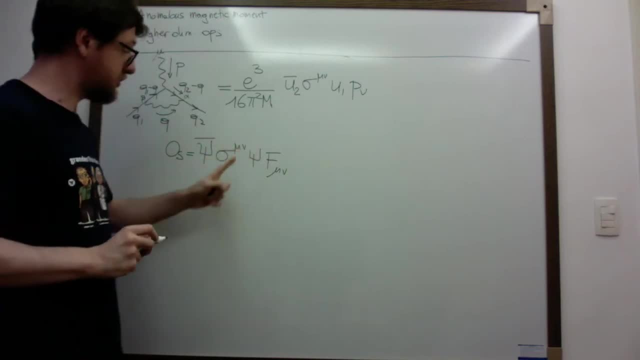 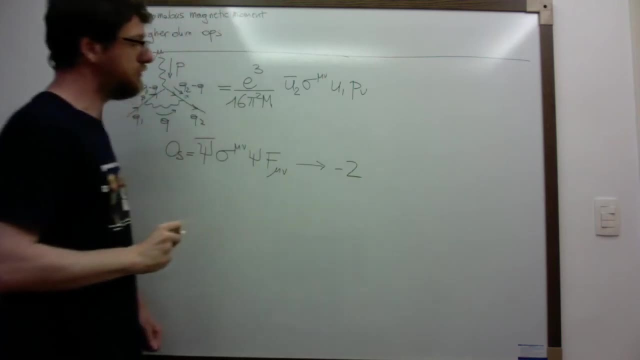 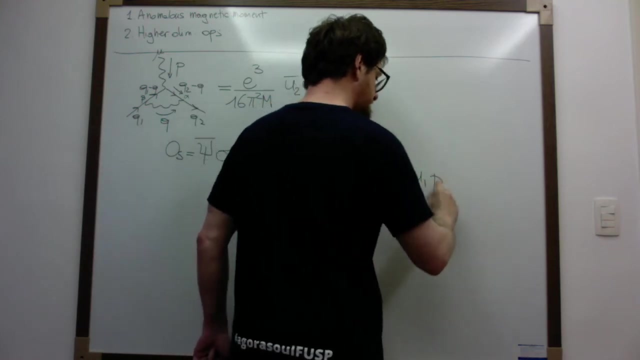 Now, if you try to compute what is the Feynman rule Associated with this operator, then you discover the following thing: You have a factor of minus two and then you will have U2 bar sigma mu nu, U1 pi nu. 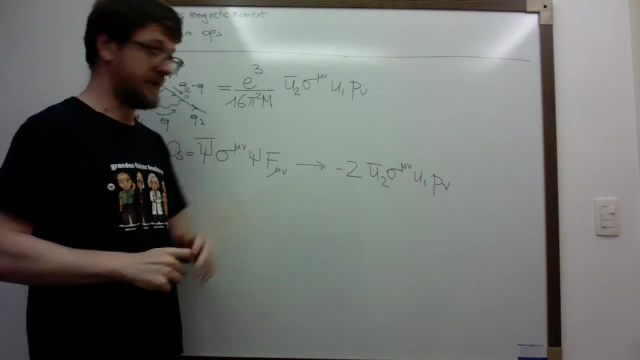 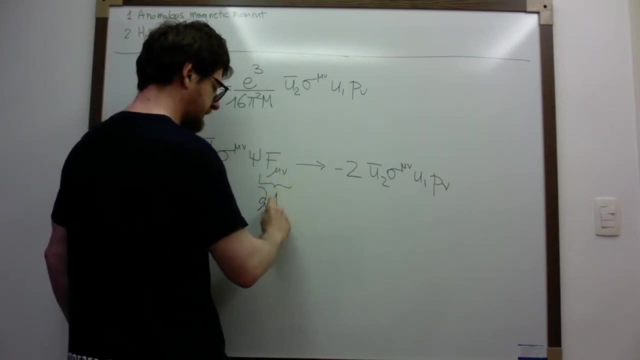 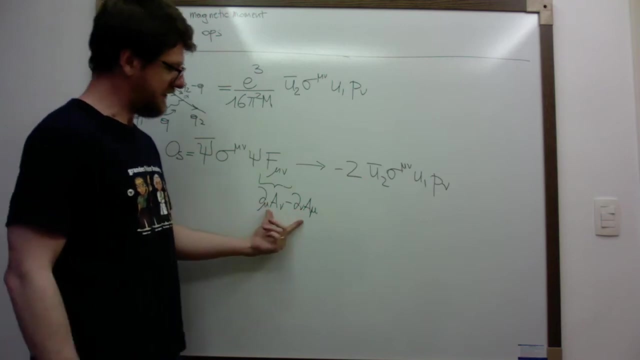 So let's try to understand where this factor of minus two comes from. okay, So the secret is in this f? mu, because, remember, this f? mu? nu is this combination of them. Okay Now, since this combination of derivatives is contracted with something which is anti-symmetric, 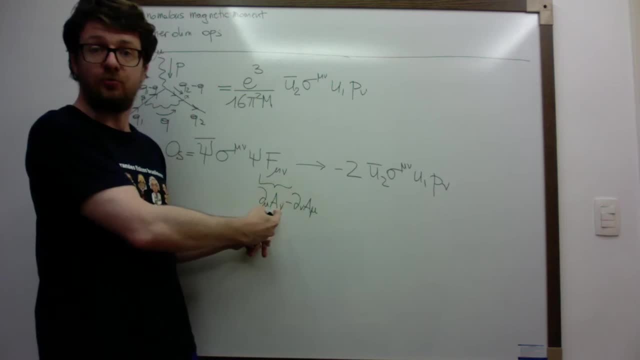 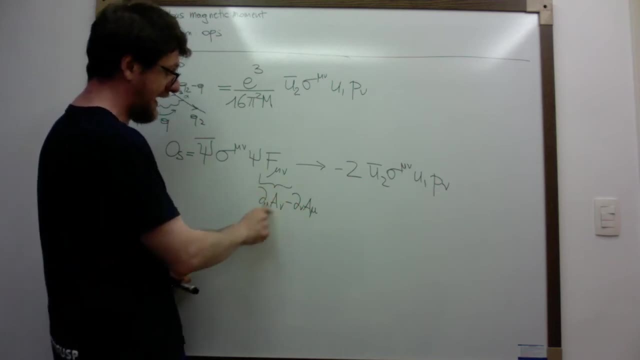 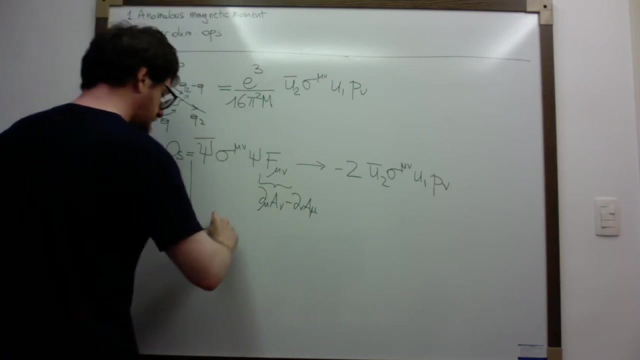 I can consider just one of the two terms and multiply by two, because doing so I automatically take into account the fact that there are two terms. Okay, So let's suppose that I do. I just consider this and I just consider this. So from here I can write this as minus two times. 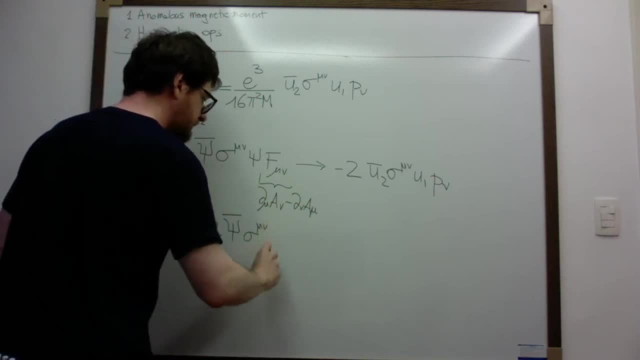 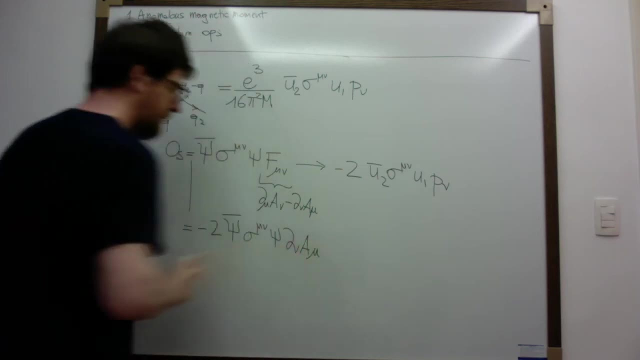 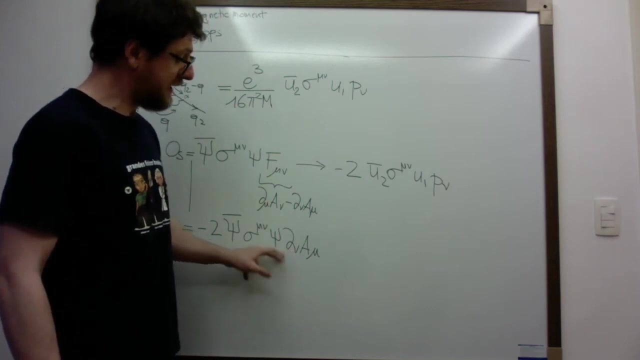 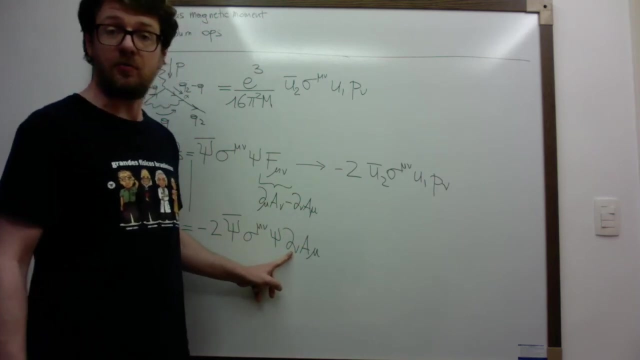 So this is sigma mu, nu, psi, d, nu and nu. And then you use the same trick that we use in the case of scalar qBD to see what is the Feynman rule associated with this derivative, And you discover that you simply have a factor of minus. i, p, nu. 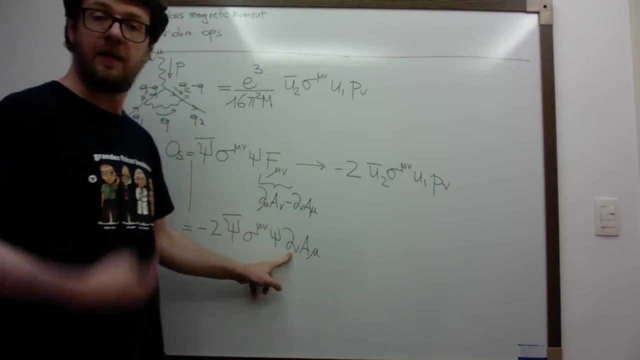 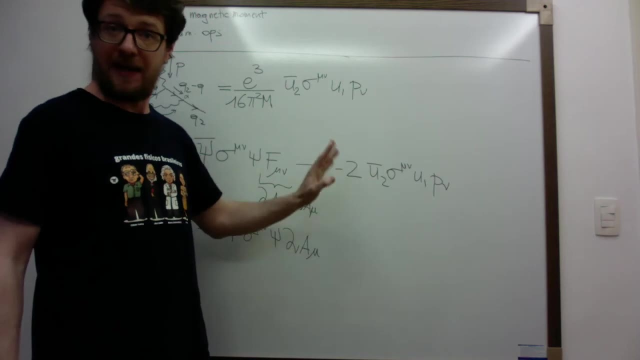 So this is a factor of minus two, minus i p nu. When you go to The final rule, you need to multiply by i. This cancels the factor of minus i and you're just left with minus 2.. Okay, So that's the origin of this factor of minus 2.. 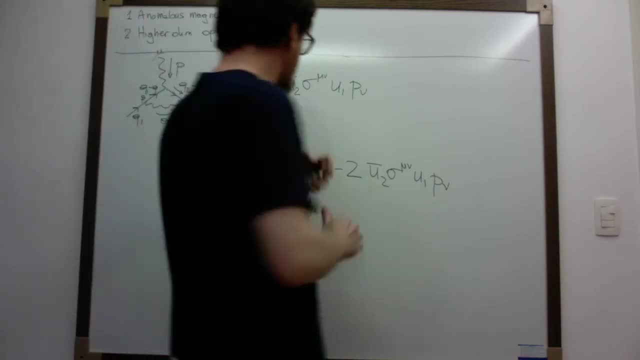 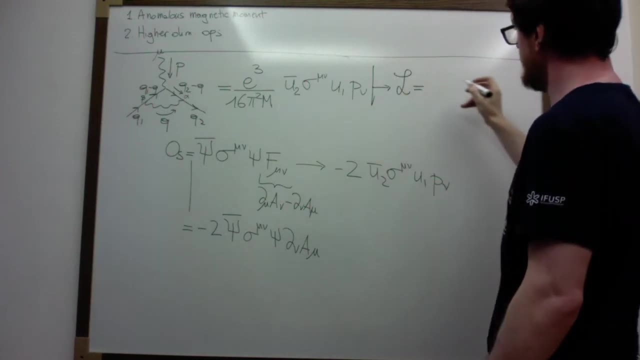 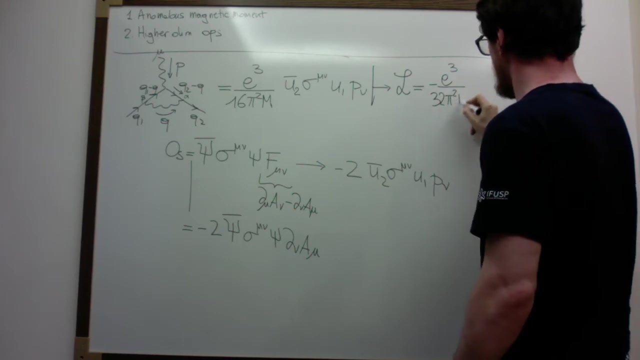 So this means that this term is equivalent in our Lagrangian to a term like the following: It's minus e cubed divided by 32 pi squared capital M psi bar sigma mu nu, psi M mu nu. Okay, So the minus sign takes into account this minus sign. 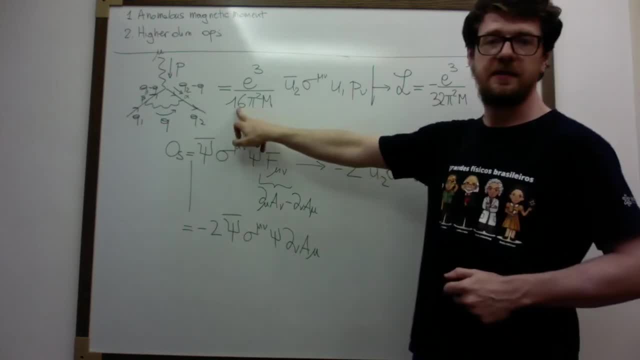 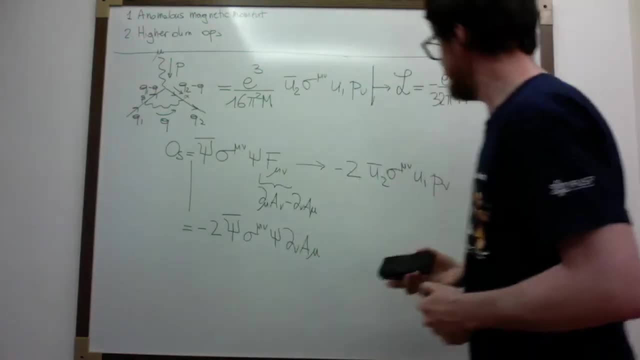 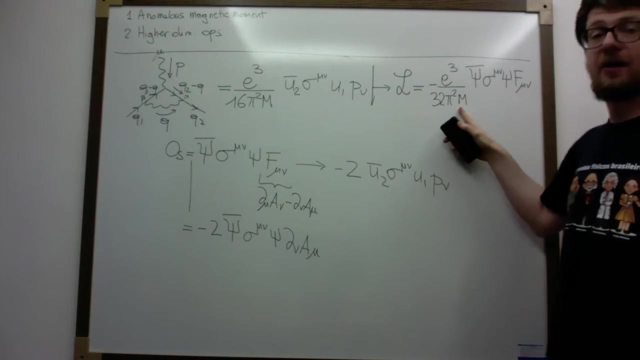 And here I put 32, because when I multiply by 2, I get this factor of 60. So this is precisely what I need. Okay, Excellent. So, having concluded that the effect of this loop at zero momentum can be taken into account in our Lagrangian, 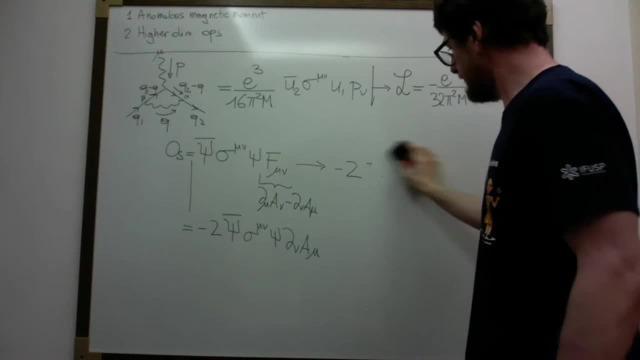 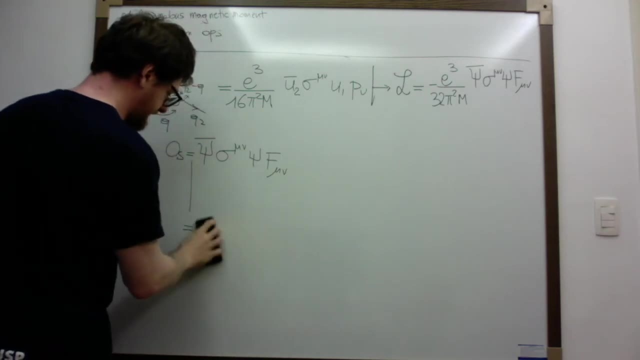 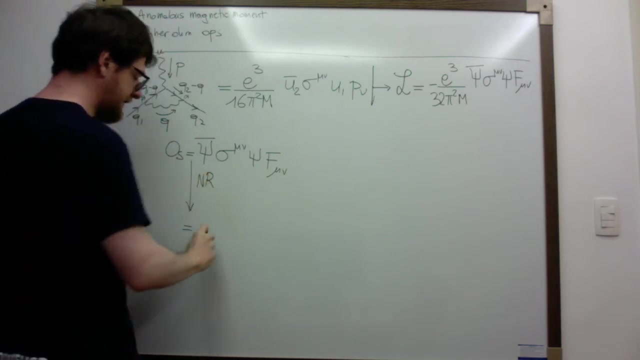 system. Simply adding the following term, we can now see what happens in the non-relativistic limit, Because, if you remember, in the non-relativistic limit, this is something that we computed. actually, I showed you earlier when you go to the non-relativistic limit. 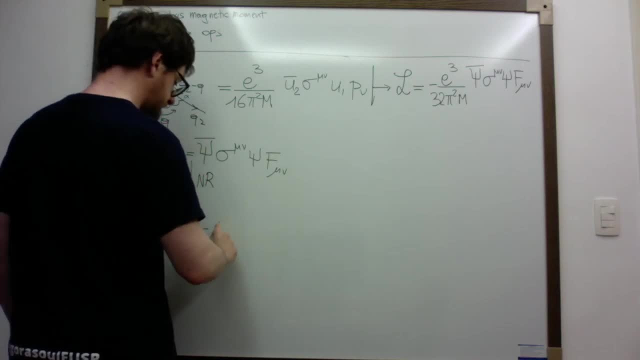 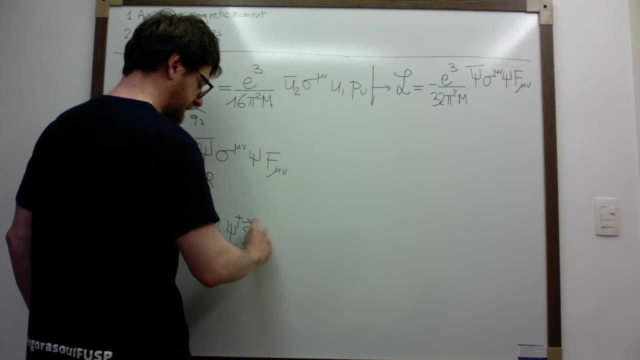 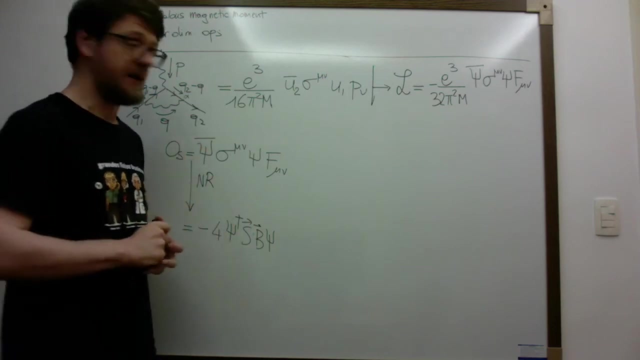 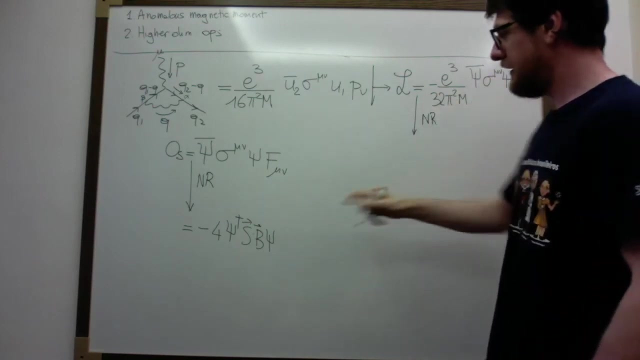 this is giving you a factor of minus 4 psi dagger s dot b. This psi is the non-relativistic component that survives in the non-relativistic limit. So this means that if I take this one and I go to the non-relativistic limit, I get the factor of minus that. 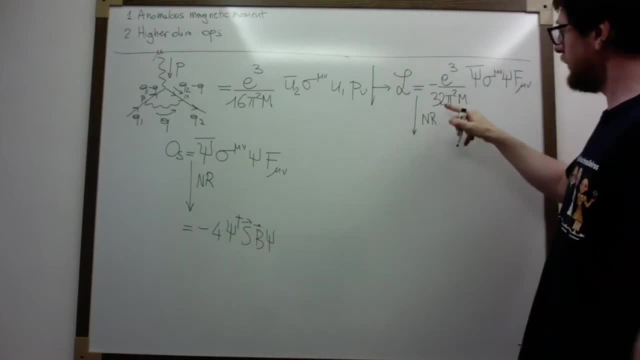 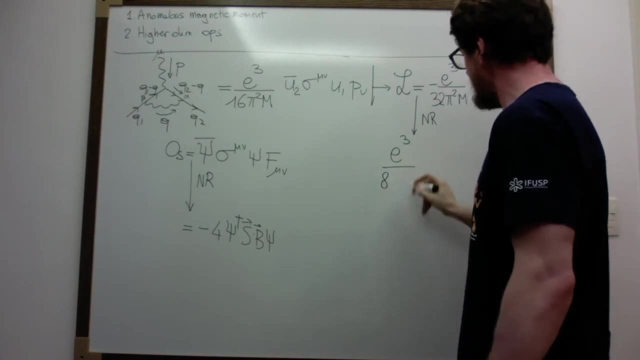 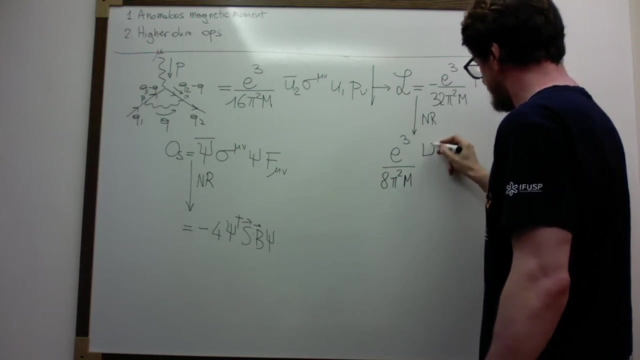 cancels this one. This factor of 4 makes the denominator equal to 8.. So this is e cubed divided by 8 pi squared M, And then I have a factor of minus 4 pi squared M, And then I have psi dagger s dot b, psi. 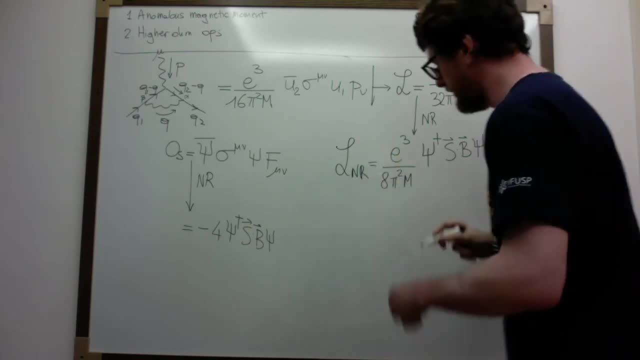 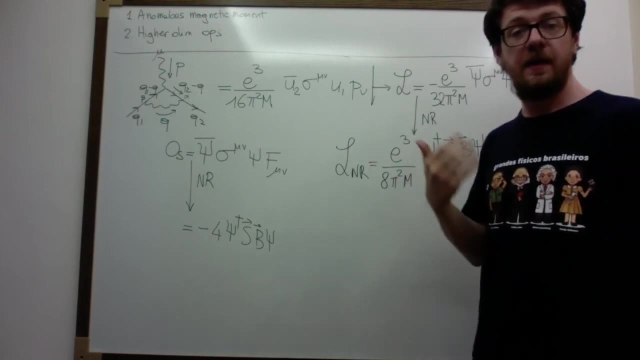 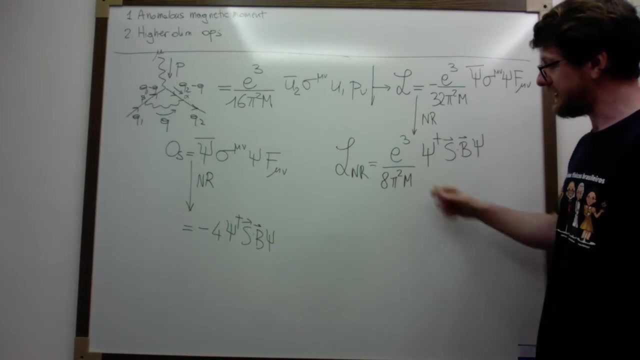 So this is the contribution that we get in the non-relativistic Lagrangian. So this is precisely confirming what we were suspecting. Radiatic correction modified the value of g at the level. At the level it was 2.. Now I need to add this contribution here. 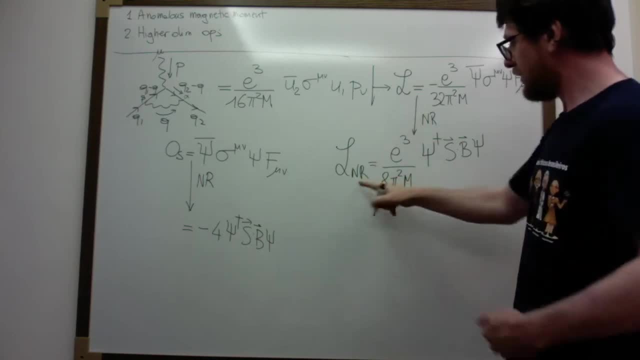 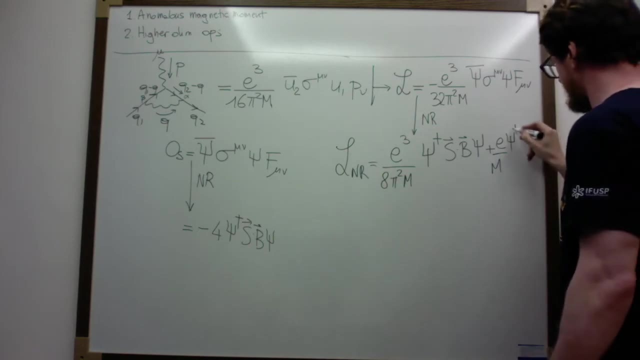 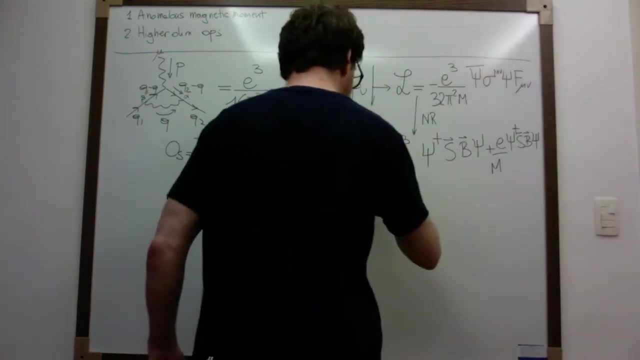 OK, So let's write the sum, Let's write the sum of the two. So n-relativistic also has the other term that we computed in the last lecture. So this is psi dagger s dot b psi. And when I put everything together, 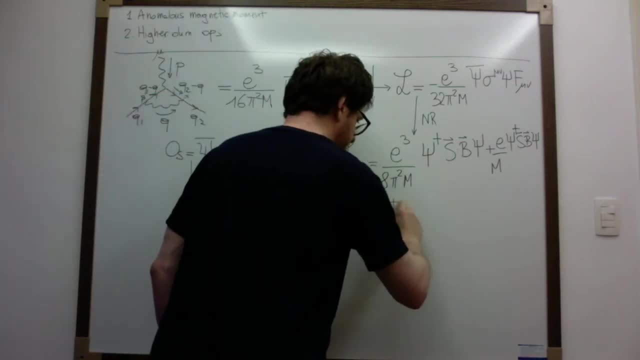 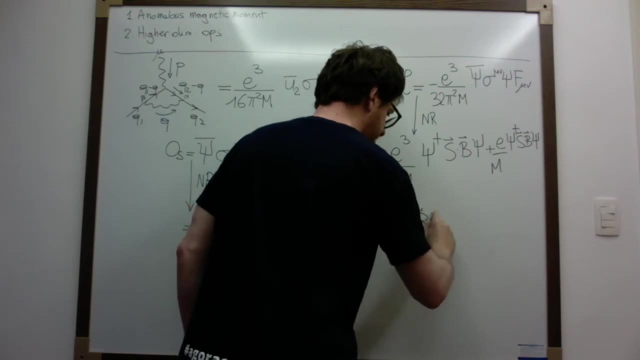 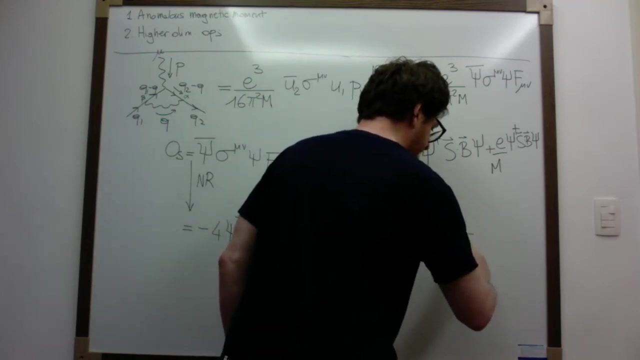 you see the following thing: So I have psi dagger from here, I get, well, I get the s dot b psi, And then I'm left with the following coefficient: E divided by 2 times M, which takes into account this term. 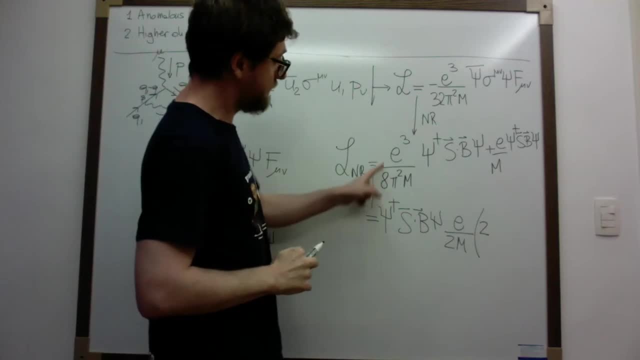 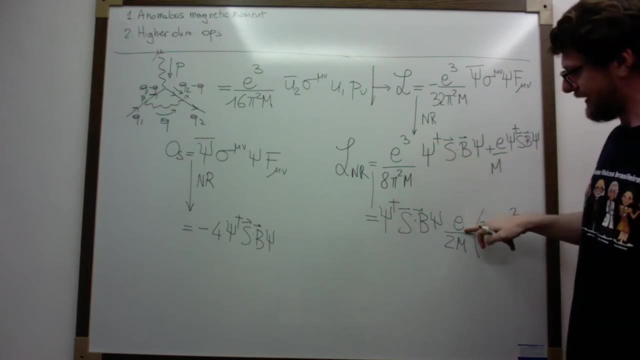 if I put here a factor of 2.. And then this factor is equal to plus e squared right. Because I started with an e cubed, I factorize 1e, So I'm left with an e squared. Now, from here I factorize a factor of 2.. 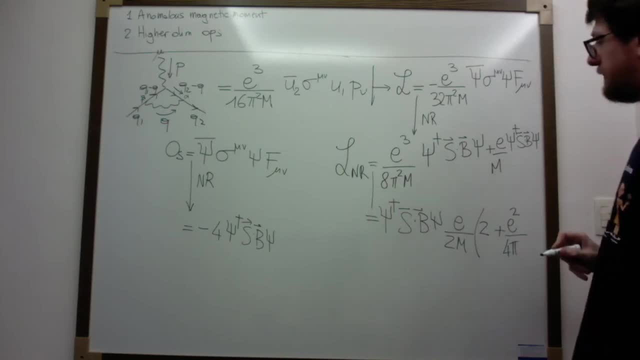 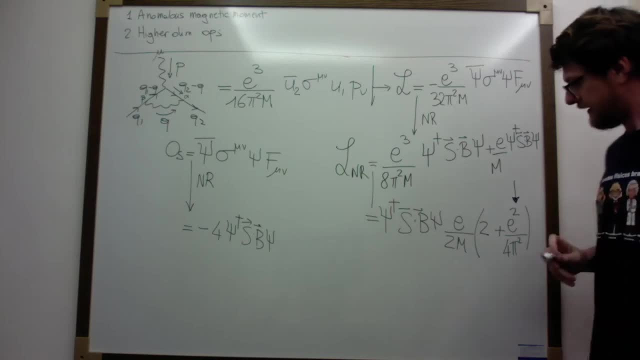 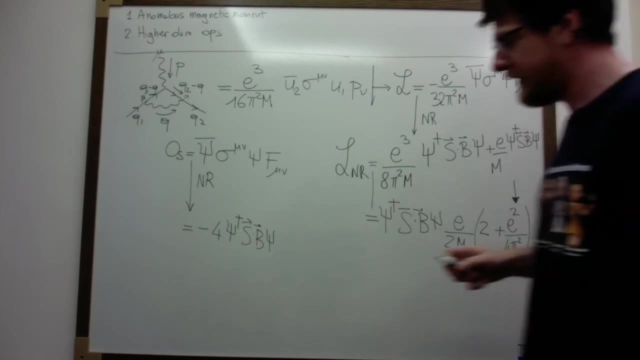 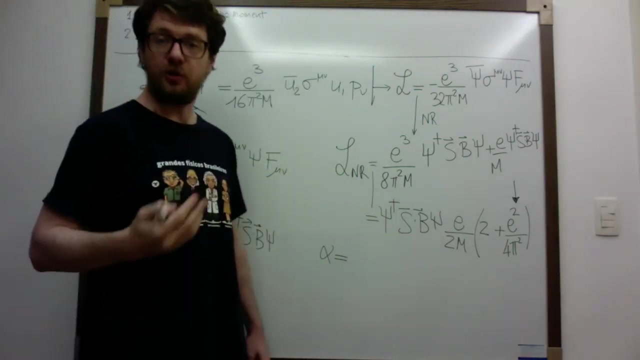 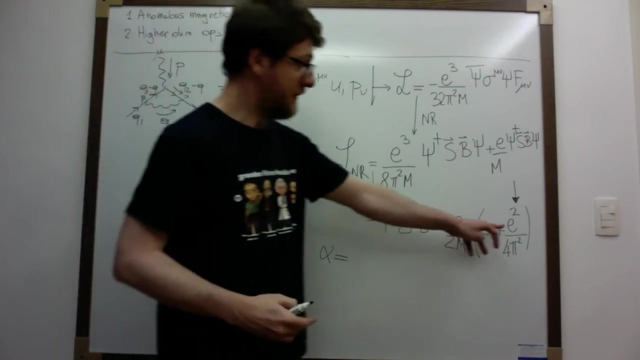 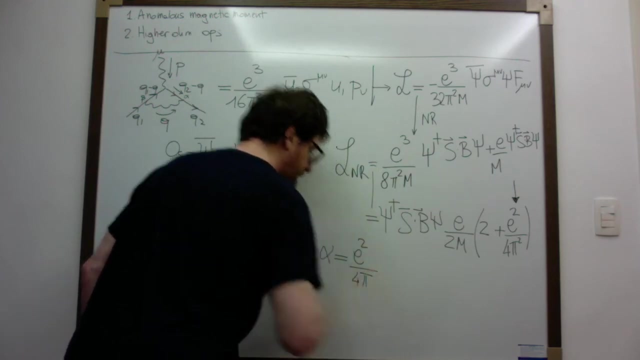 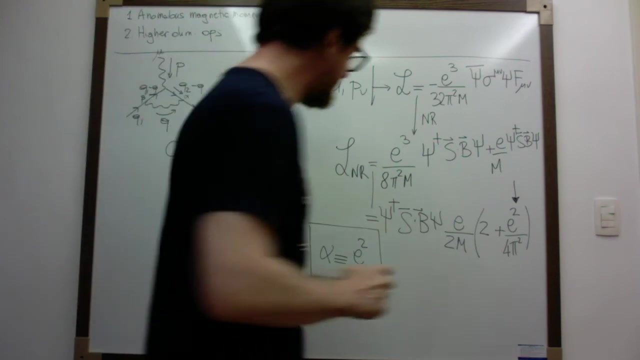 This is the anomalous part of the magnetic moment of the OK. This is a. you see this result written in another way in the literature, Because it is customary to define what is called the fine-structure constant. This is a historical term. This is not a constant, because this thing will be proportional to e squared, and the definition is the following: This is e squared divided by four pi, And so this is the definition of the fine structure constant. So, in terms of this fine structure constant, 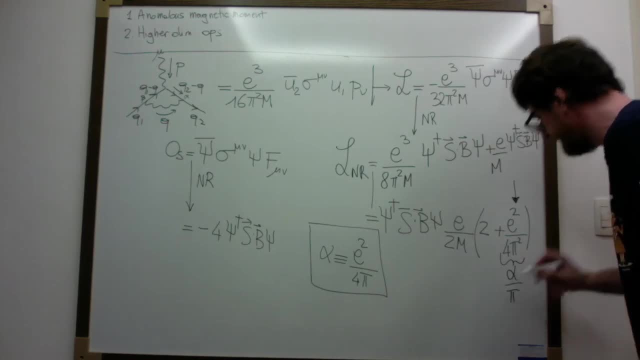 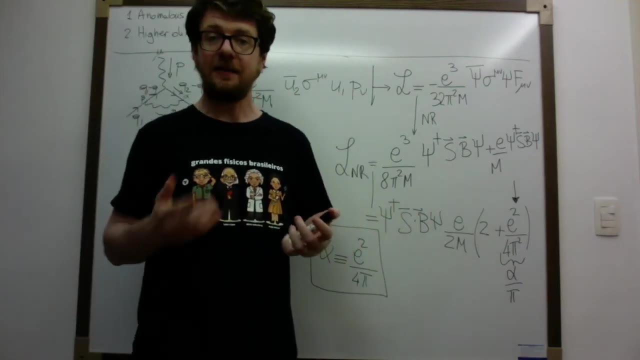 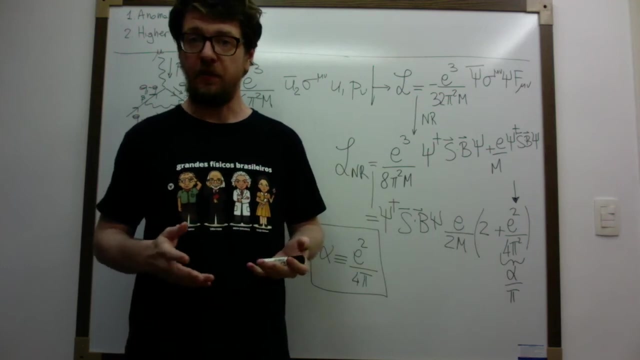 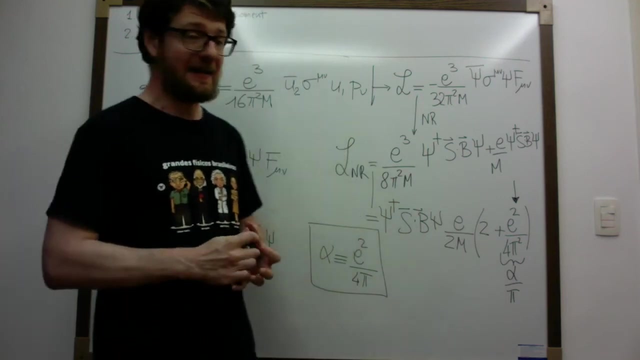 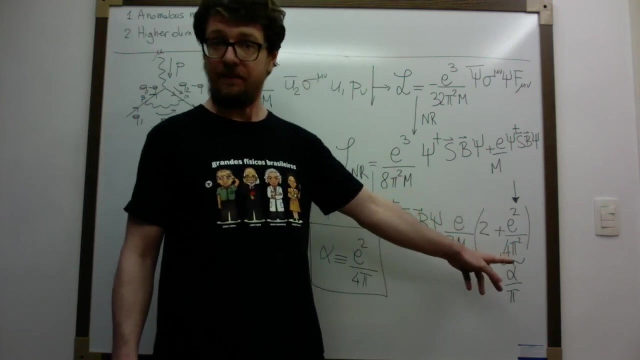 our correction is simply equal to alpha divided by pi. So this was, I think, the first result at loop level computed in quantum field theory. It was computed at the same time by a bunch of people among which Feynman, Schwing and Tomonaga- I think these were the first three- And the comparison of this anomalous magnetic moment with the data. 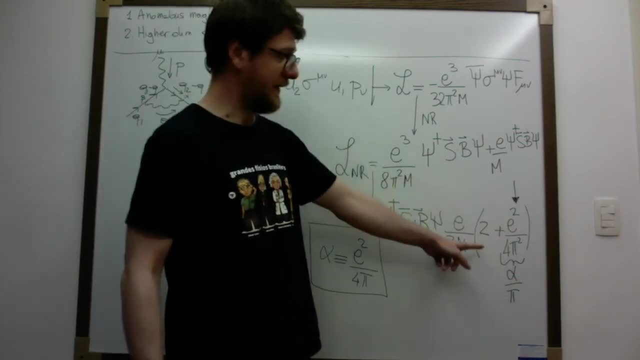 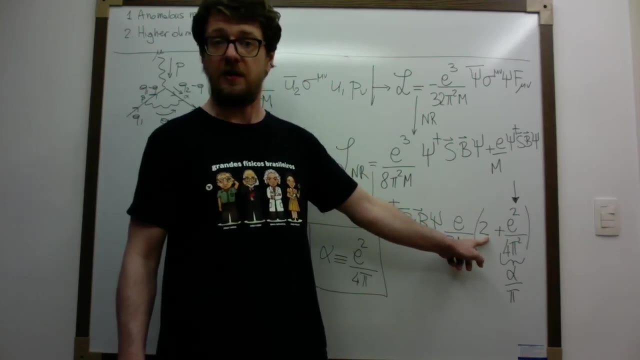 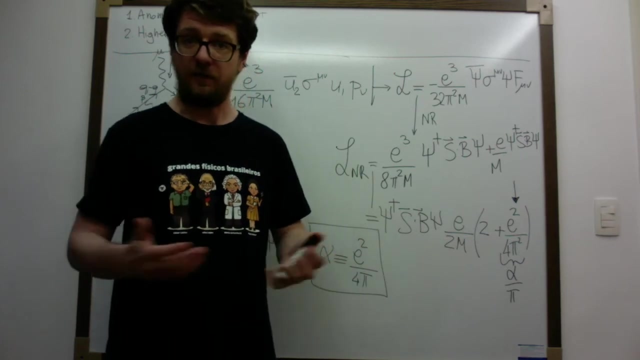 which we're showing in the deviation of the magnetic moment of the electron from two was one of the first great confirmations that quantum field theory was on the right path to actually describe the quantum theory of light and matter, okay, of quity. 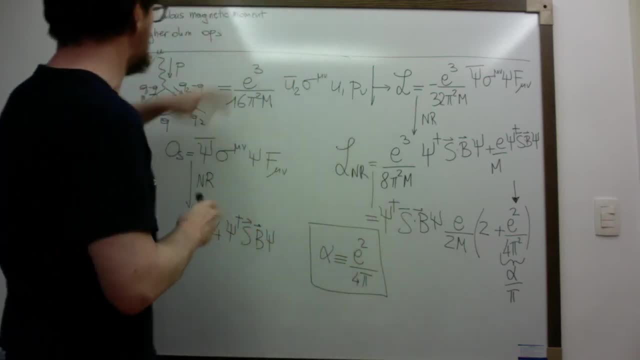 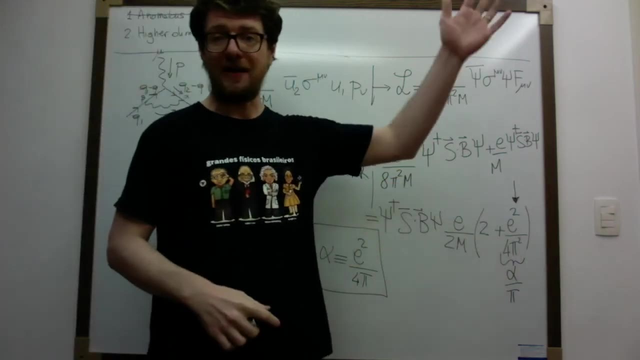 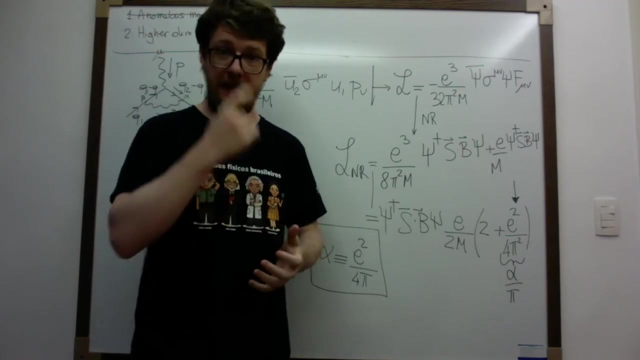 Very good. So this concludes our discussion of the anomalous magnetic moment. So we will get back to this object later on, much later in the course, when we discuss, when we will discuss the experimental confirmation of the standard model, And actually we're going to see that this alpha 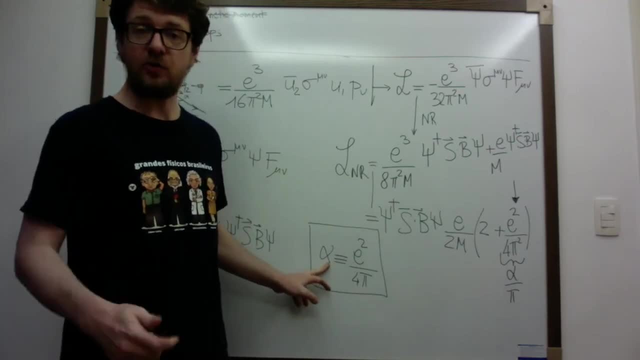 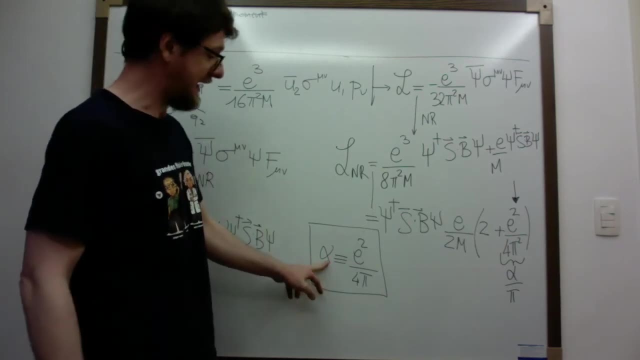 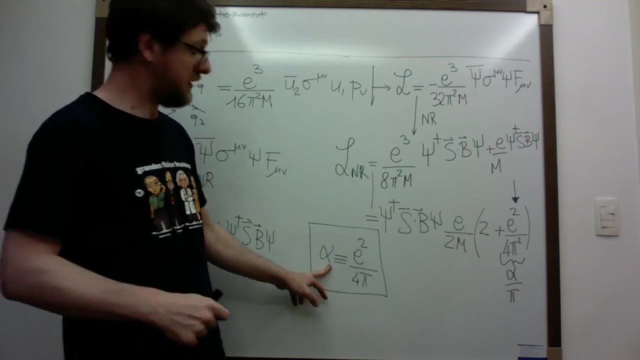 is measured so well at low energy that actually we're going to use it as an input parameter. okay, So we're going to trade some of the parameters in the standard model- Lagrangian for this alpha and something else. okay, some other, some other parameters that are measured very well that we will introduce And then using those. 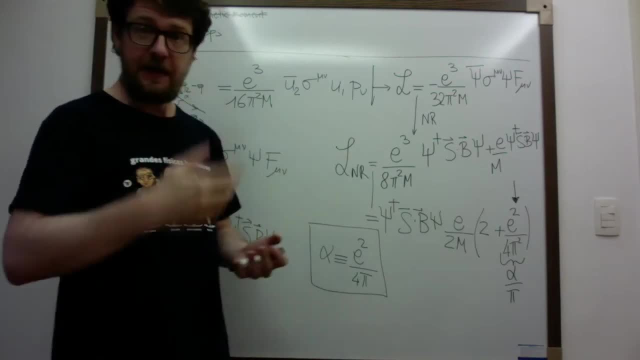 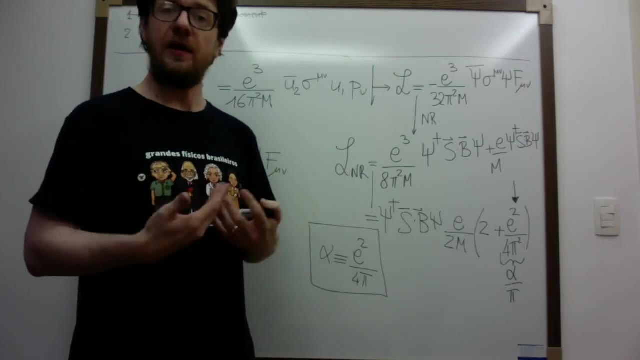 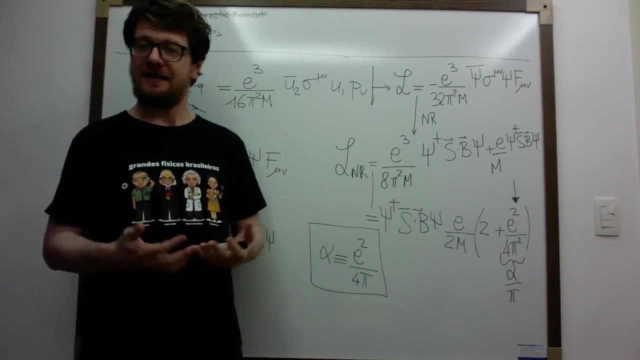 parameters as inputs. so we're going to make predictions. okay, And again, let me just anticipate what will happen. The standard model will be compatible with data only once we consider loop effects. Okay, So in all, the loop effects in quantum field theory are one of the most strange things and it really takes. 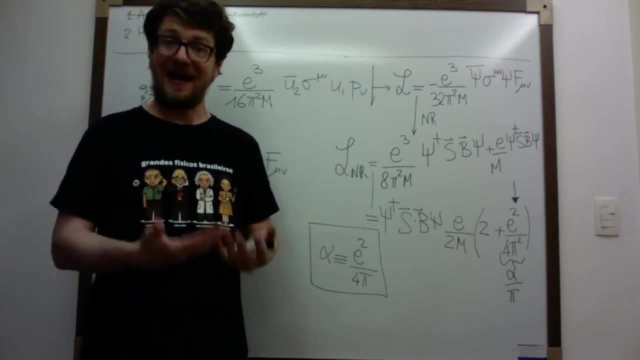 a lot of time to digest them, But it's worth it because, without the effects of loops, the theory, our best candidate for a theory for particle in case physics would miserably fail to reproduce it okay. So always keep in mind that they're very annoying. 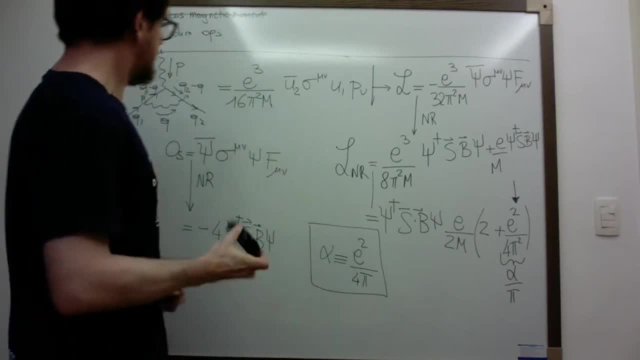 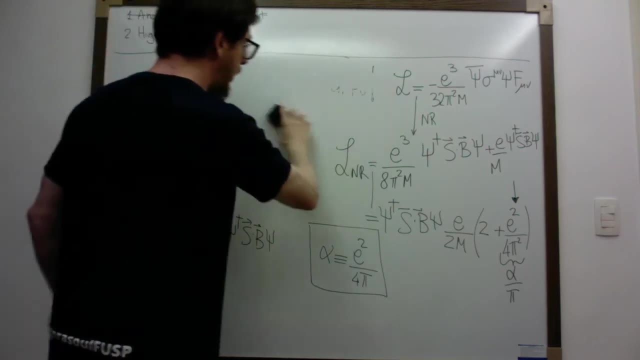 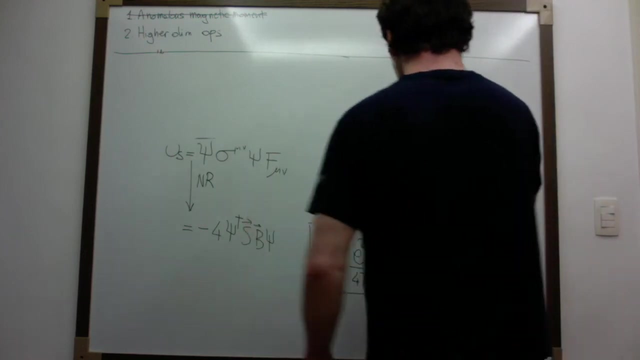 but loops are really, really important. So let's now move on to the discussion of higher dimensional operators. I'm not gonna discuss all the higher dimensional operators because they are thousands. So of course, as you can imagine, it depends on the dimension at which we want to stop. 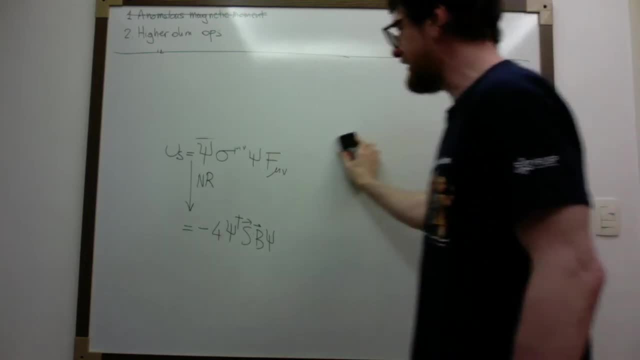 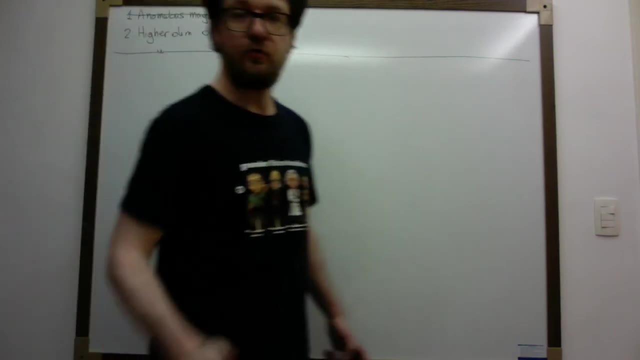 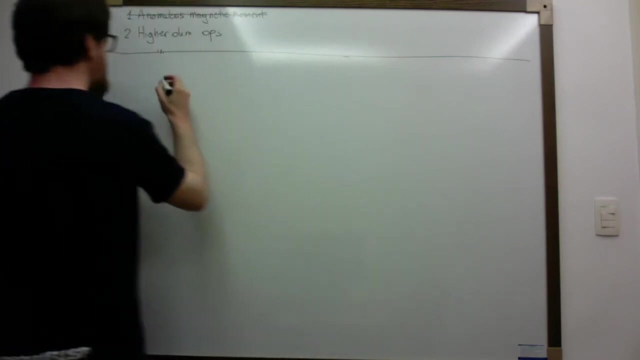 So how much we want to take the suppression in the power of one over lambda, I'm just gonna consider quickly two examples which are two dimensional operators. So the first one we know very well, which is simply the one that we just considered, 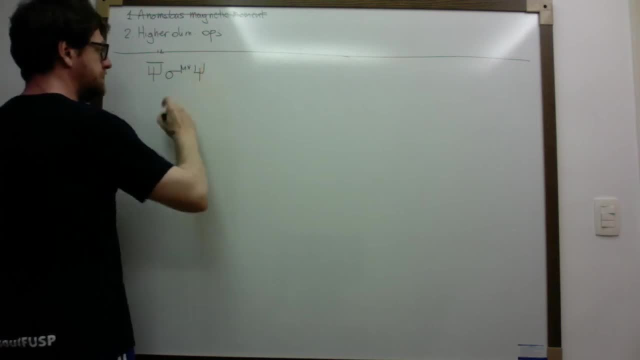 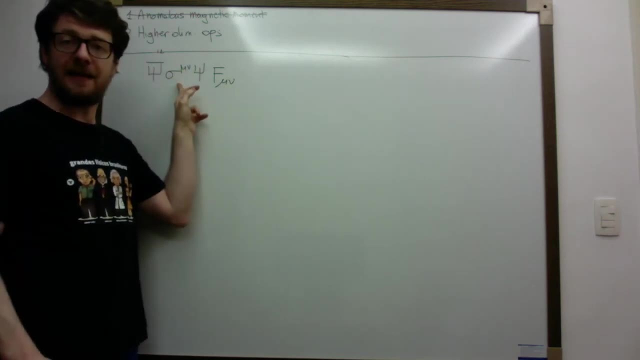 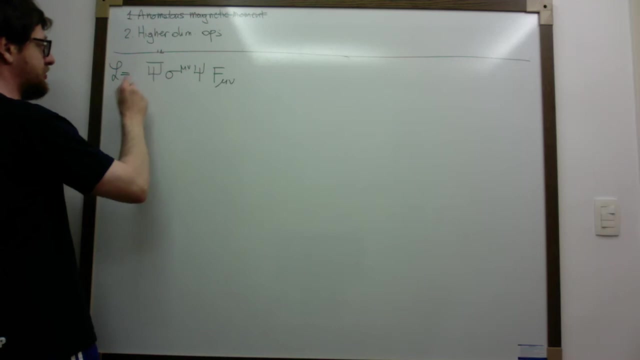 So psi bar sigma mu nu, psi f mu nu. But now I'm not considering the contribution coming from a zero momentum, from the loop, but I'm just saying that this is a possible operator that emerges at the level of dimension five. So the coefficient here is called. 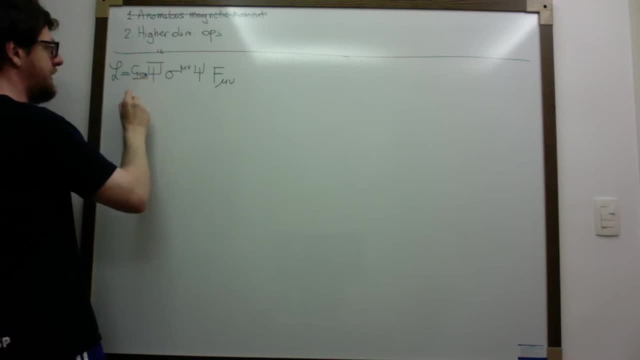 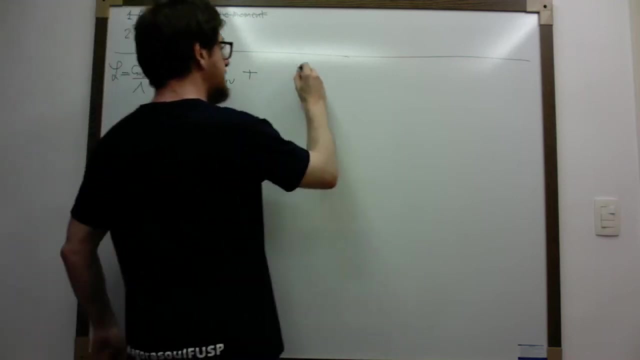 C magnetic dipole moment, MDM. And to remember that this is an independent contribution, it's not generated by loop. let me suppress it directly with lambda, okay. And then the other one is a closed causing of this object and it's given by psi bar. 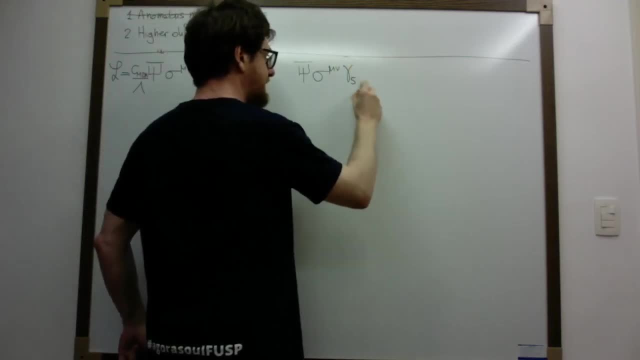 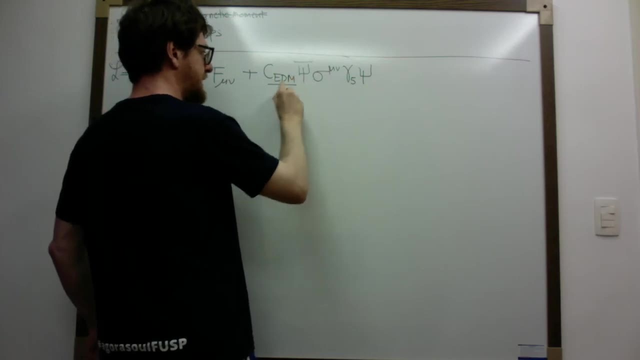 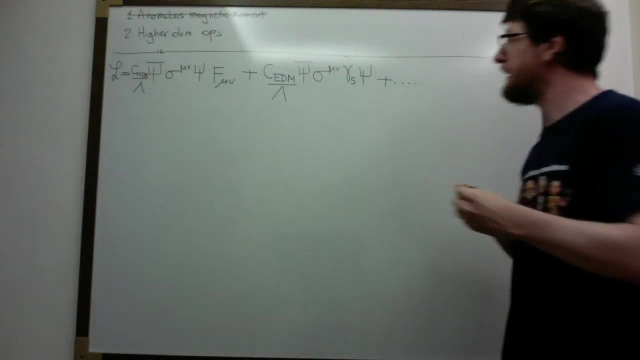 Sigma mu nu. Now I multiply by gamma five psi, And this one is called electric dipole moment operator for a reason that will become clear in two minutes, okay, And then, of course, we have many, many, many more operators. 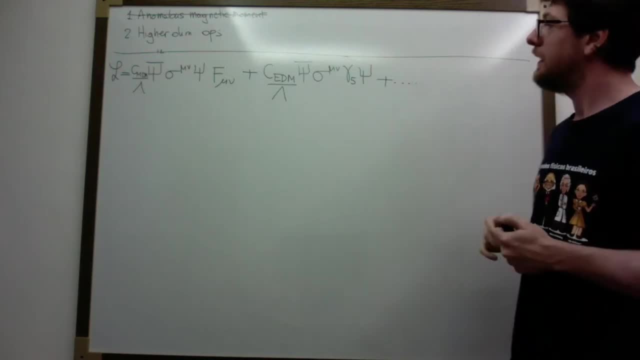 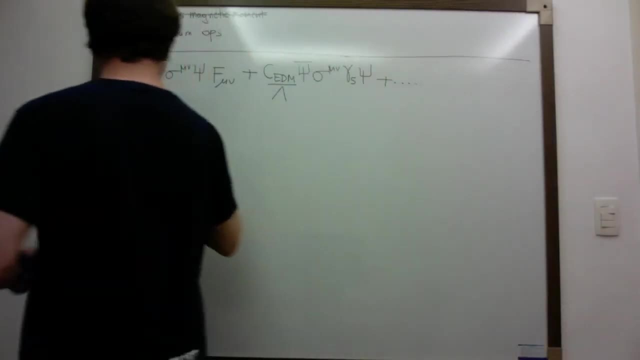 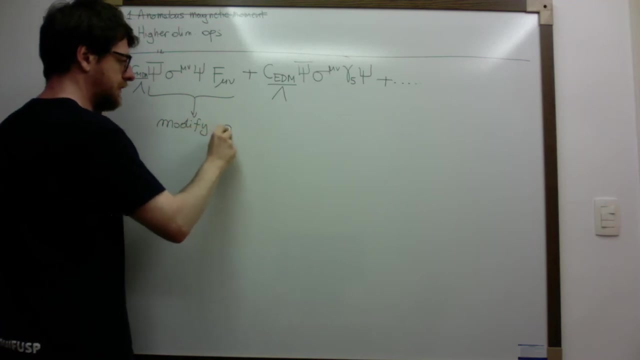 that we are going to complete in this regard. okay, Excellent, So what are the physical effects of these two operators? Well, the physical effect of this one is clear, because this will modify the magnetic moment of the electron in the wavelength. okay, 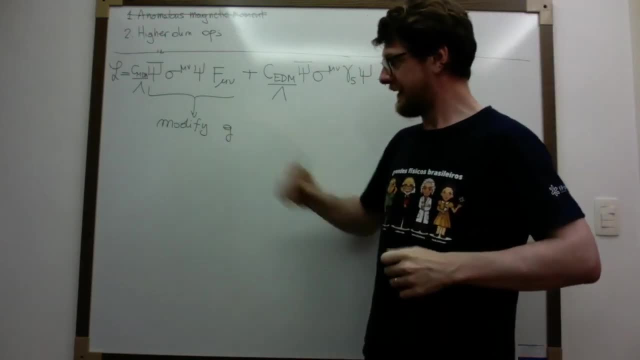 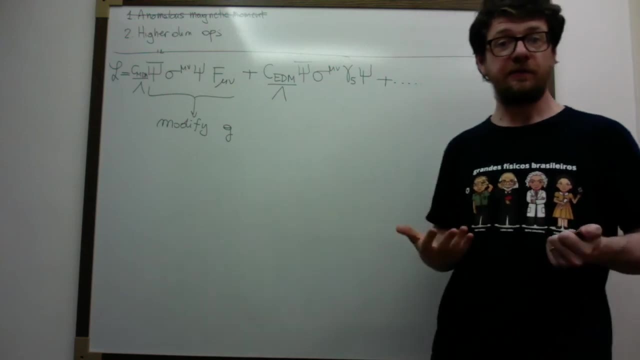 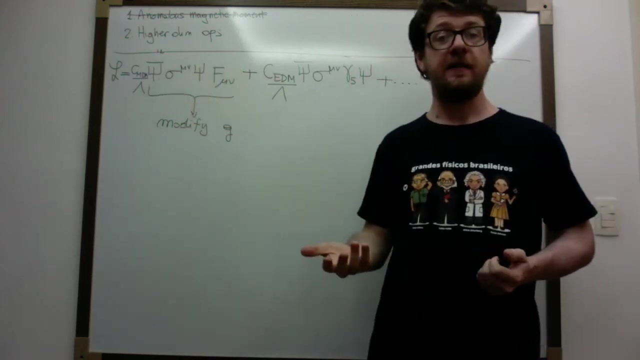 So if it modifies this magnetic moment, it can pollute our extraction of value. okay, So this is one of the first lectures that you need to take: that higher dimensional operators can actually interfere with extraction of data all the time of parameters from it. okay, 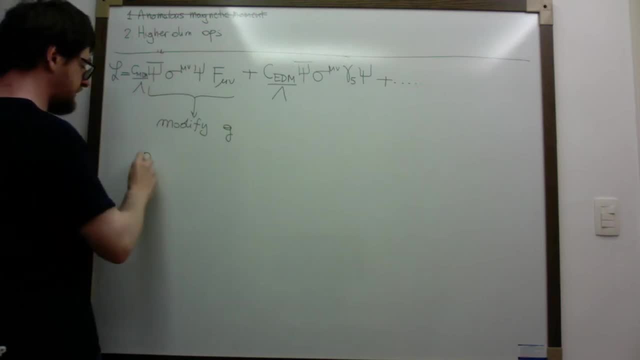 We just saw that without this operator, g was equal to two plus alpha, divided by p, by pi. And now this object here will introduce something which is like minus. let me see if I can get it right. I believe this is minus four times C, MDM. 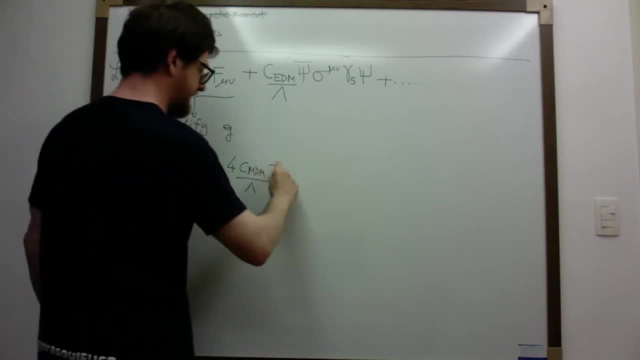 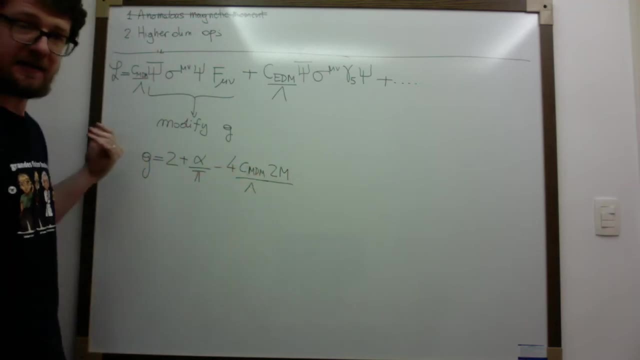 that is divided by lambda, And I guess there is a factor of two times N up here. okay, To compensate from the one that I am factorizing out. So you see that, if this is the situation, what we're actually measuring is a combination. 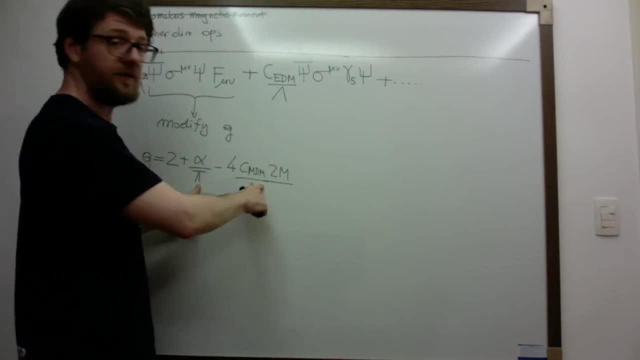 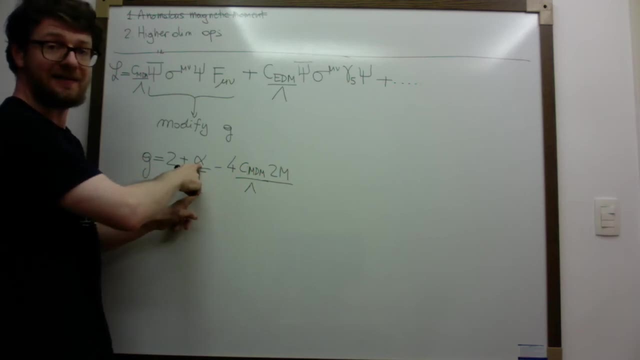 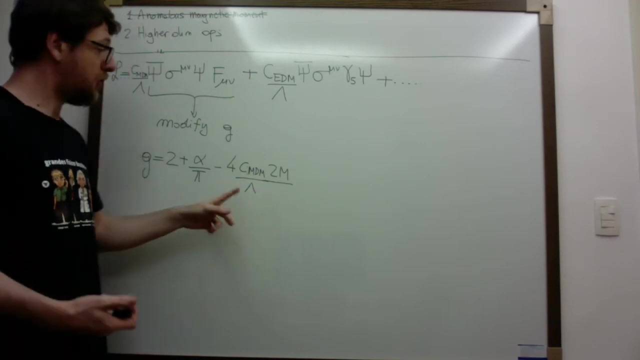 of the three level effect, the loop effect, and of this higher dimension operator. So we cannot trust the value of alpha that we extract because we think it is just due to loop corrections, but actually there is something in C. Of course, this happens only if this term 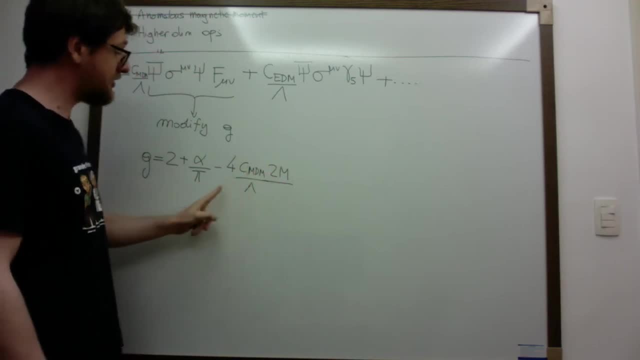 is comparable to this term. If it happens that this term is much, much smaller than this one, then we have no problem whatsoever. okay, But since we don't know a priori what is lambda or what is this C MDM, then this is something. 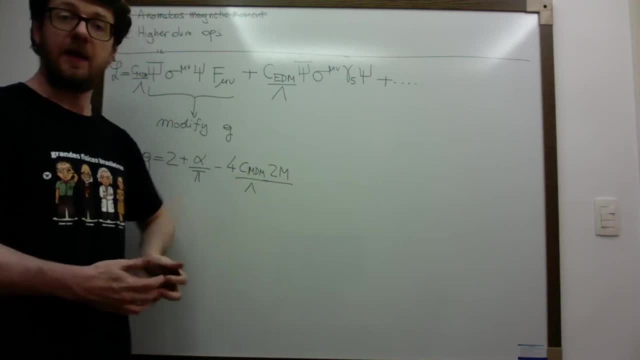 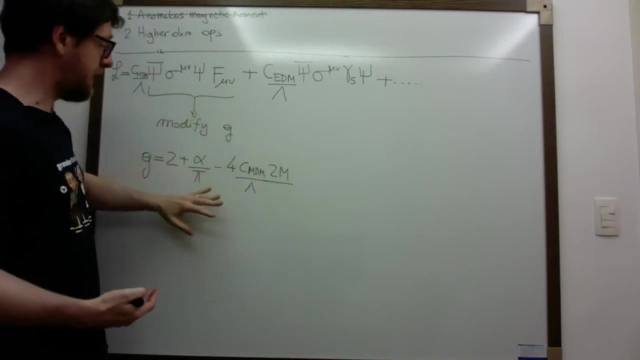 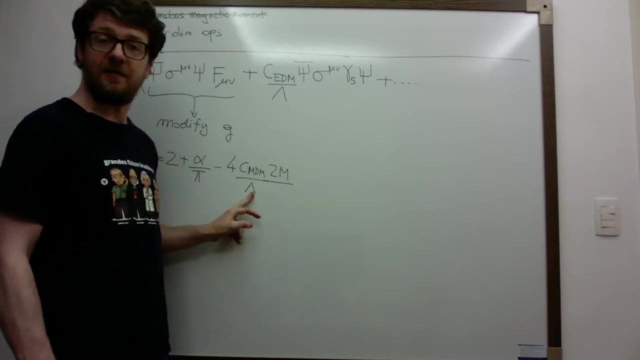 that, at a certain point, we must take into account. okay, What is usually done is that you start by ignoring this and then, after you discover all the when, after you discover that your theory is well compatible with data, you start to turn on these other terms. 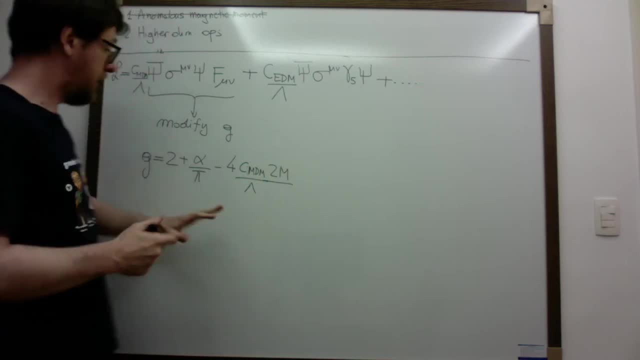 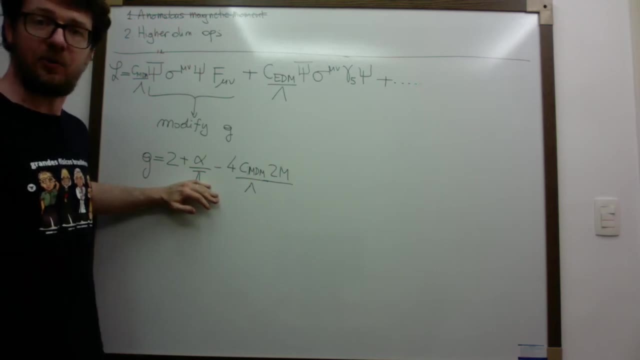 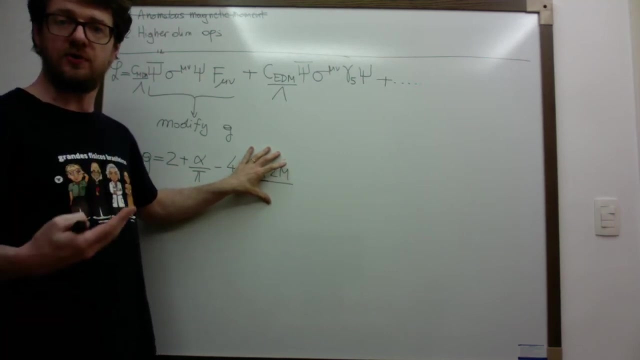 considering them as more deformations of the results that you already have. okay, This is what is done in the case of the standard model. The standard model has an excellent agreement with data, without considering the contribution of the higher dimension operators. So what we do up posterior is to use this compatibility. 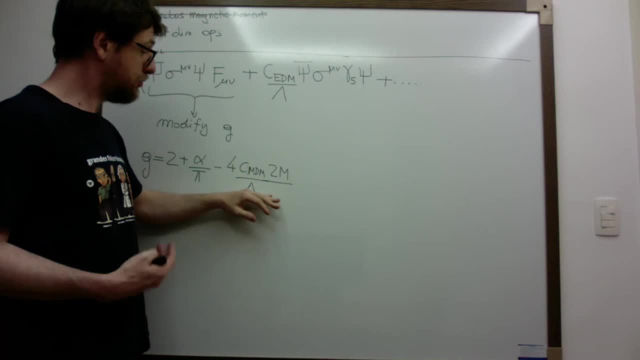 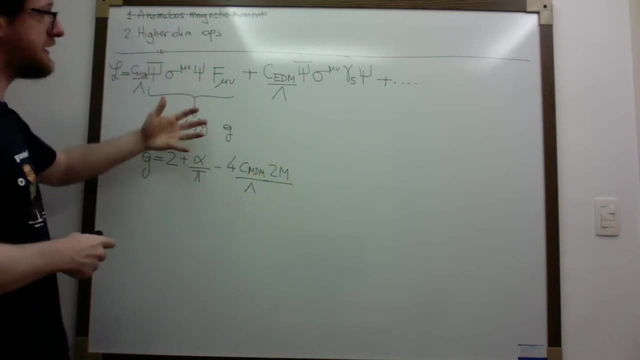 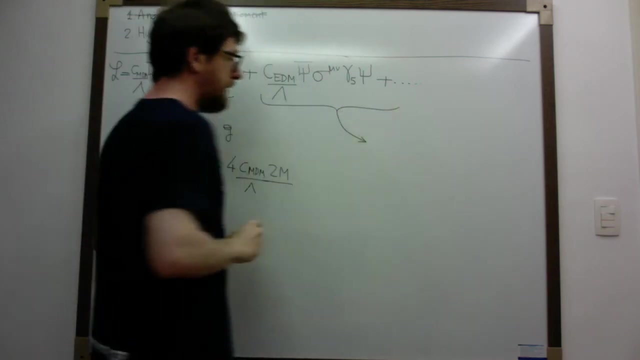 with data to say that these corrections, these deformations, must be small. okay, So the physical effect of this one is clear. Now, what is the physical effect of this other one? Well, this other one is a operator that gives rise to what is called an electric 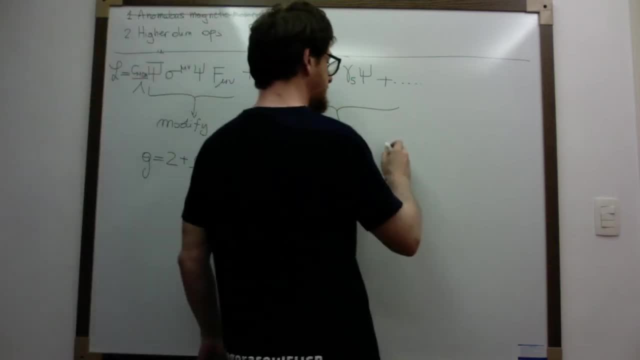 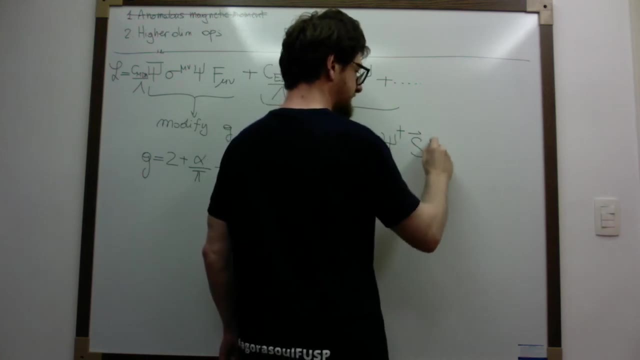 Okay. so when you go to the non-relativistic limit from this object, you discover that actually you obtain a term which is proportional to this Psi dagger S Psi. So this is exactly the same kind of spin that we saw already, but now this time. 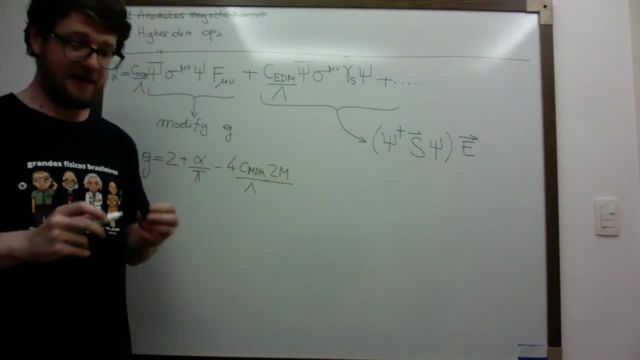 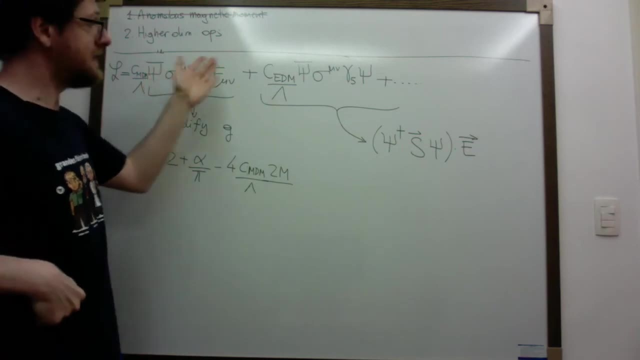 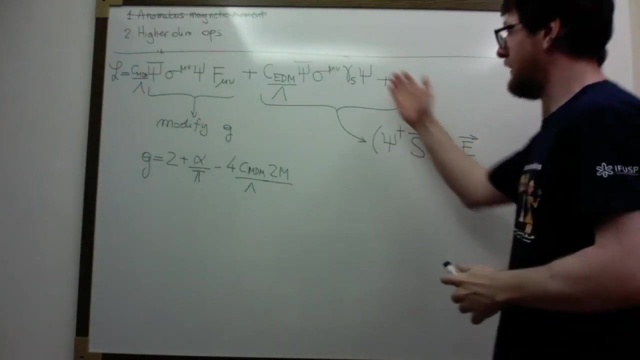 you couple this with the electric field and not with the magnetic field. okay, So this was the magnetic moment and this is, by analogy, the electric diaper moment. So why is this a term? Why is it special? Well, you see, first of all this is a physical effect. 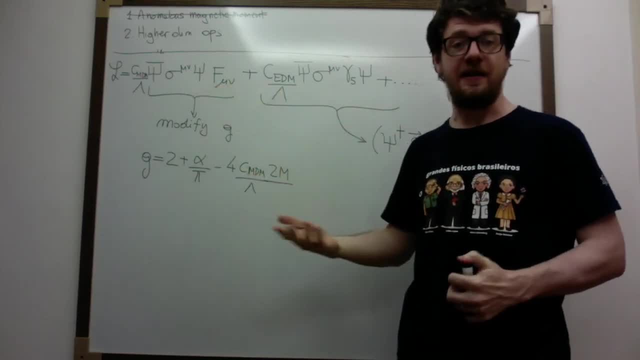 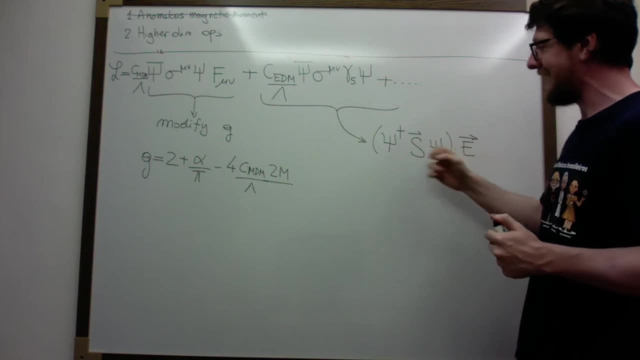 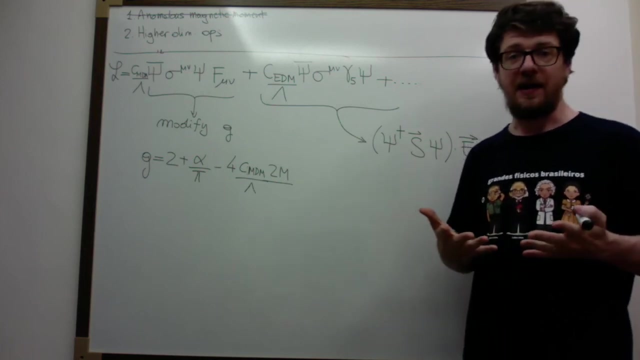 that was not present, not even at loop level in 3D. okay, In the normalizable QED we do not produce this electric diaper moment, So this is something that we already saw. we already mentioned once in our lectures that higher dimensional operators can actually give rise. 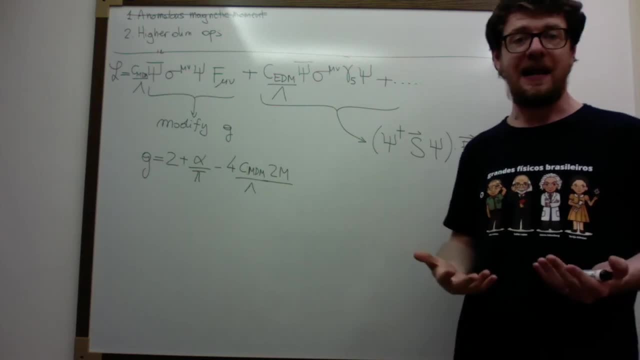 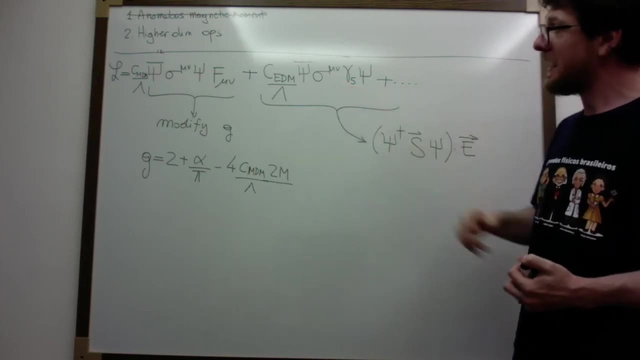 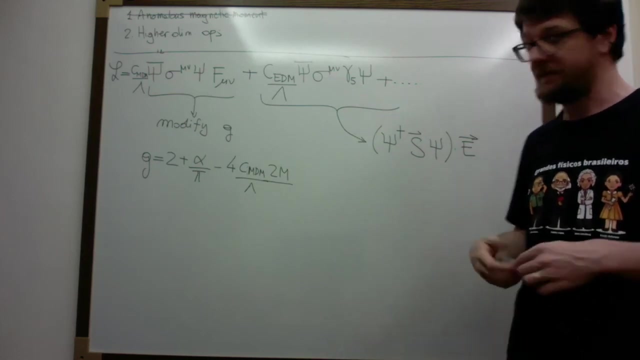 to new physical effects which are not predicted by the normalizable operators, And so we can search for these new effects, okay. This operator, by the way, has also an additional feature, because it's breaking a symmetry of the normalizable electric field. okay. 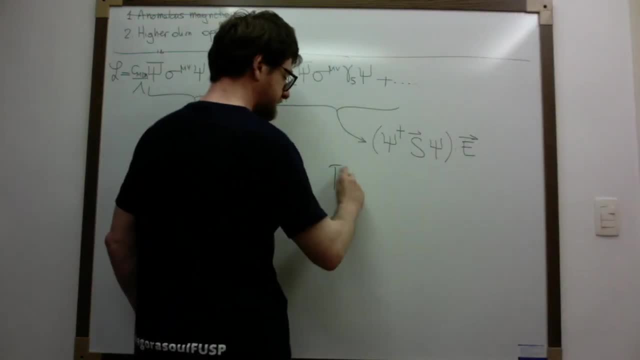 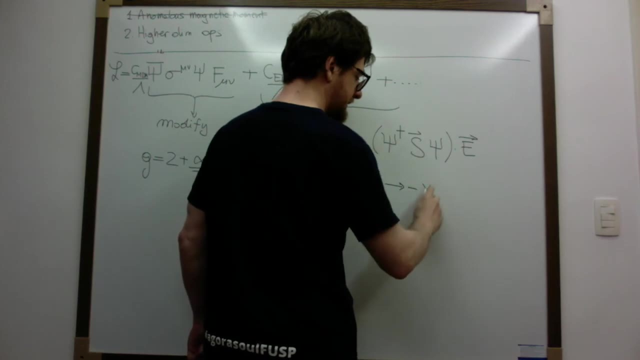 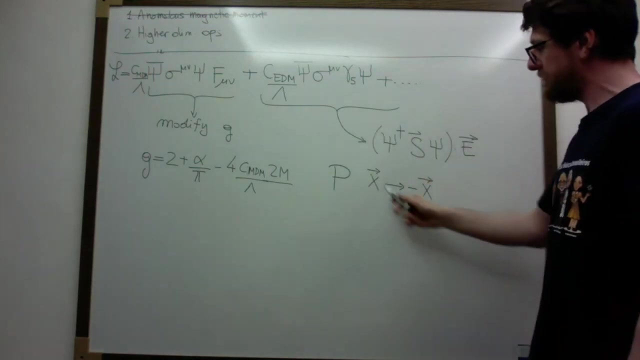 So the symmetry that it is breaking is a parity. Parity is the symmetry that takes the special part of the full momentum and sends it to minus itself. okay, So this is a transformation that can be predicted- sorry, that can be extended at the level of spinors. 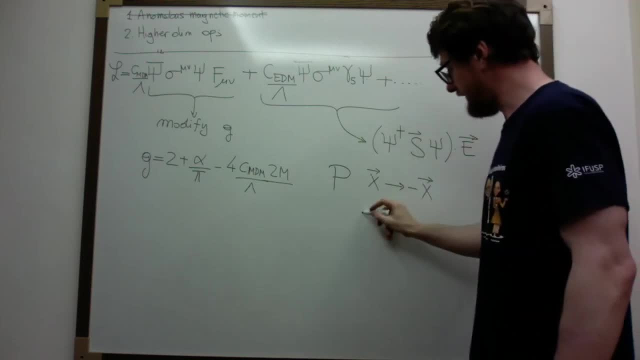 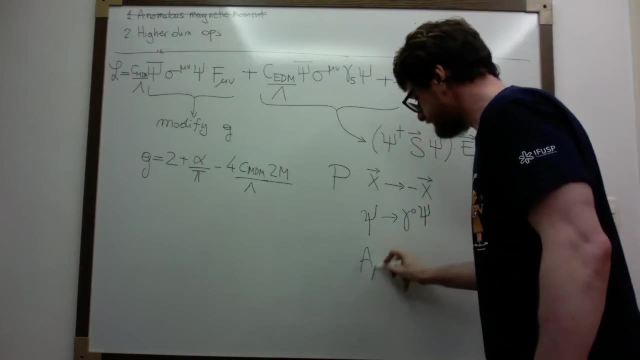 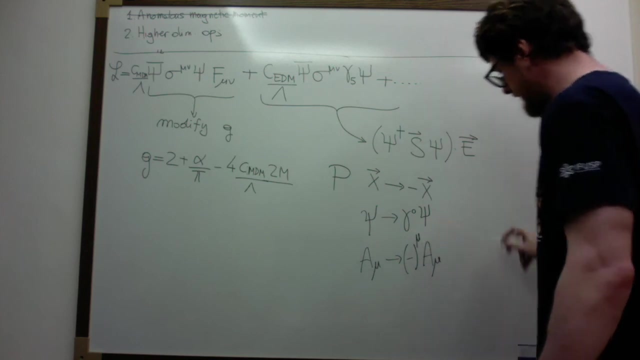 and of four vectors. So when you do that you discover that your psi under the parity transformation goes into gamma, zero psi and a mu goes into itself, apart from a factor which let me call minus to the mu. and this minus to the mu 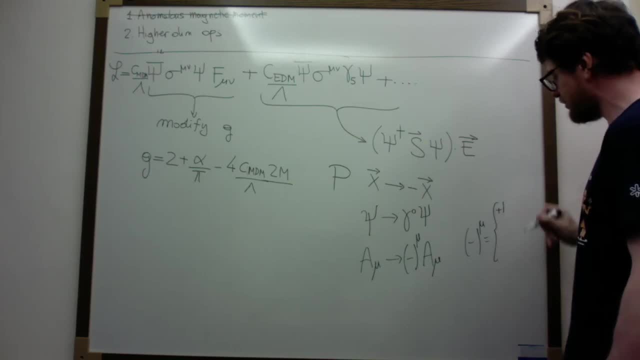 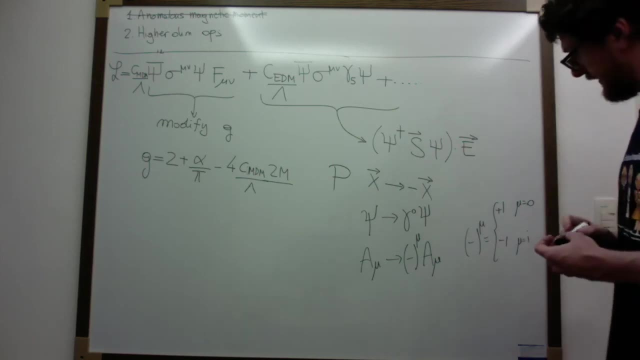 is equal to plus one when mu is equal to zero and minus one when mu is a special index. okay, So you see that parity has a strange behavior here. twisted behavior, because it modifies the sign of the components in a different way. 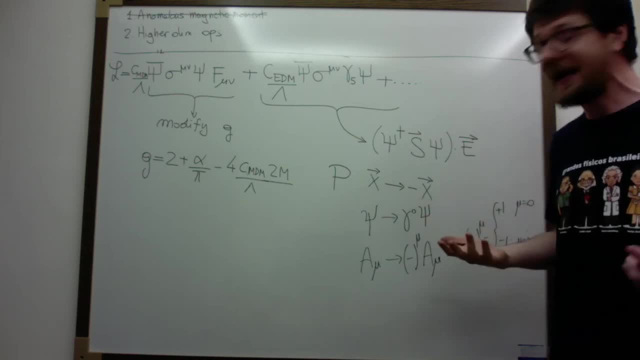 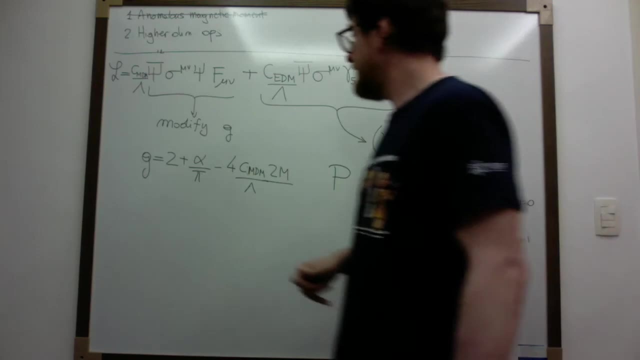 So the time component is, of course, an effective, because we're not doing any time, but the space components are affected by this kind of sign, which is consequence of this microsecond. okay, So now you can ask yourself what is the effect of this transformation. 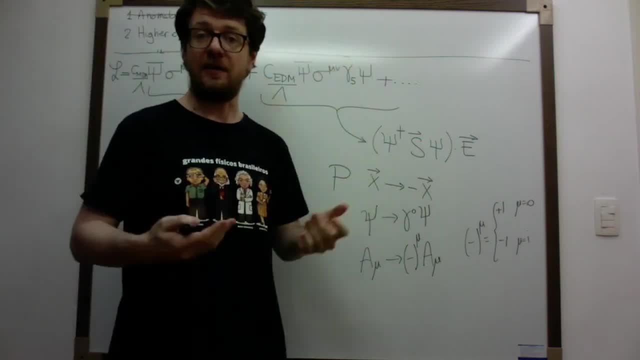 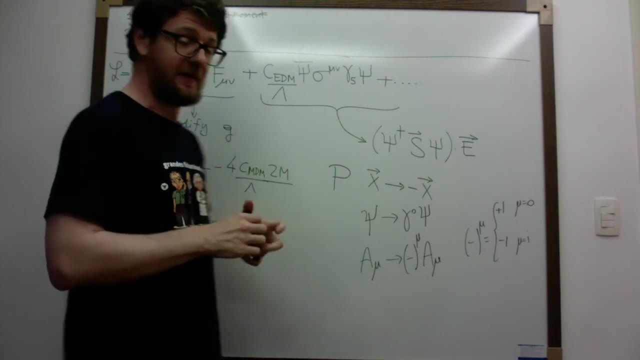 at the level of these operators or at the level of the operators in the renormalizable Lagrangian. okay, And you can easily see that the operators at the level of the renormalizable Lagrangian are completely invariant under this transformation. 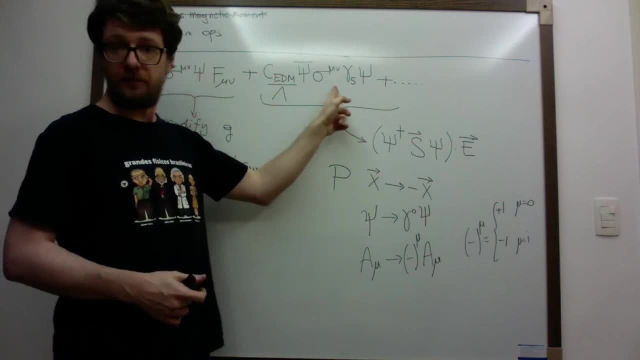 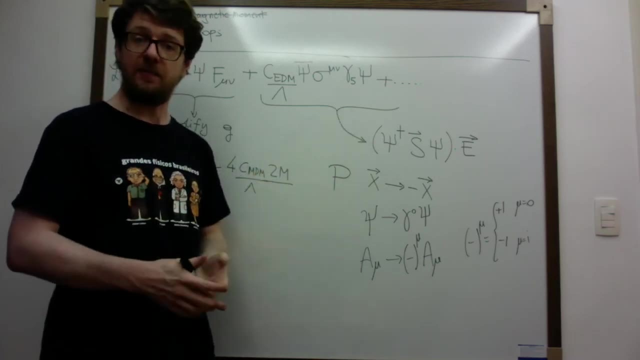 This operator is invariant and this one is not okay. So this is an operator that explicitly breaks a symmetry of the renormalizable Lagrangian. I'm not going to show you in detail this. this is just algebra. it's really just algebra. 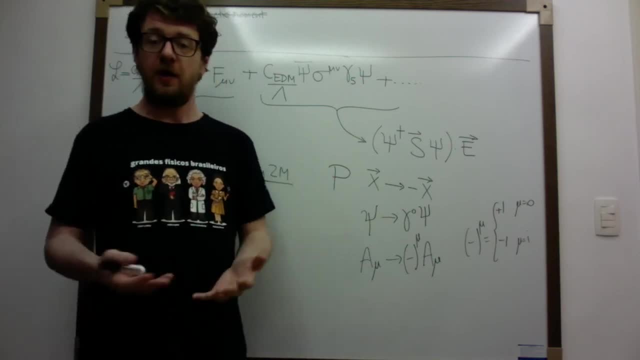 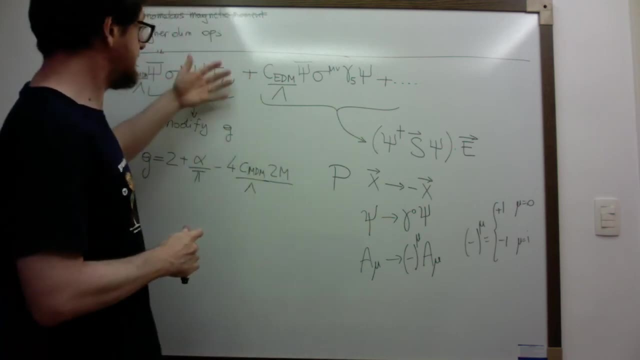 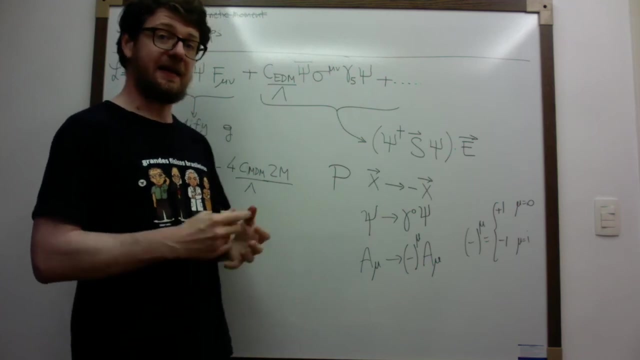 so it's just a matter of sitting down into the computation. You can find more details in the notes, but the conclusion is the correct one. This respects parity. this violates parity. it's not invariant. So this means that if we can measure, 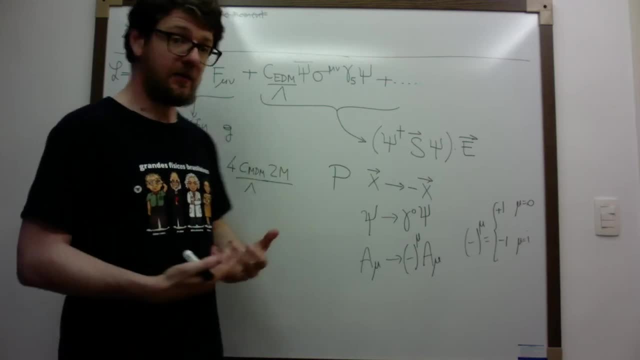 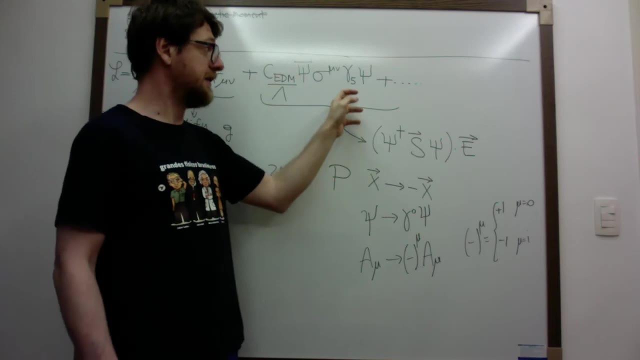 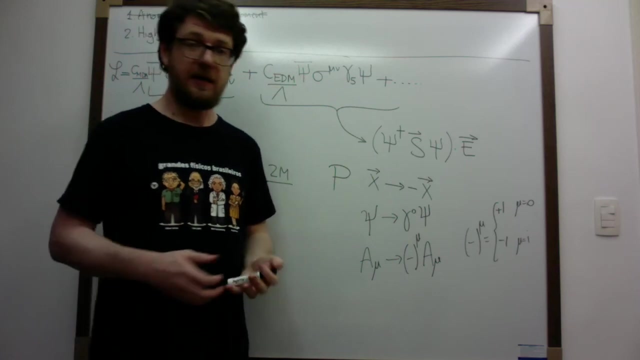 this violation of parity at low energy. then we will have access to this coefficient here, to this Wilson coefficient, of this dimension of five OPA, And of course, this effect has been searched and has not been found. okay, So the latest result comes from the ACME. 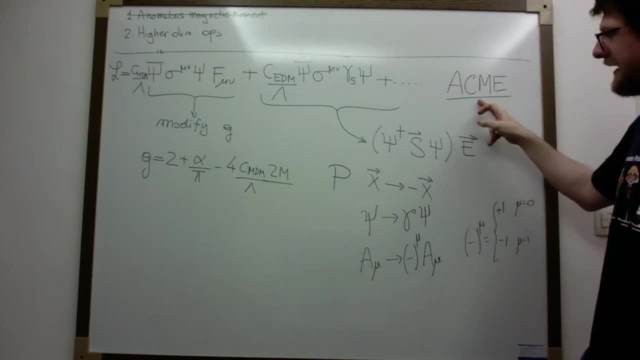 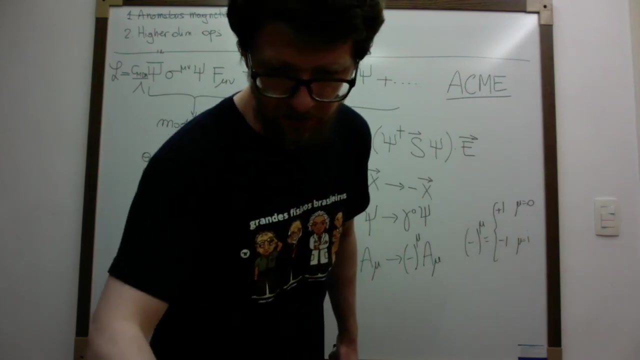 the ACME experiment. So the ACME experiment is an experiment which is designed to search for the electric vapor moment of the electron. So this ACME result, the ACME experiment finds a result which is extremely strong. So let me check just the number. 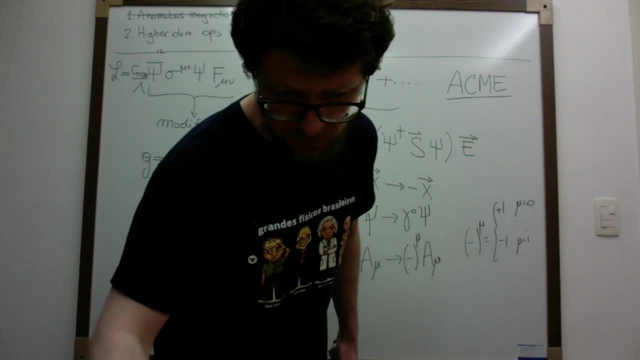 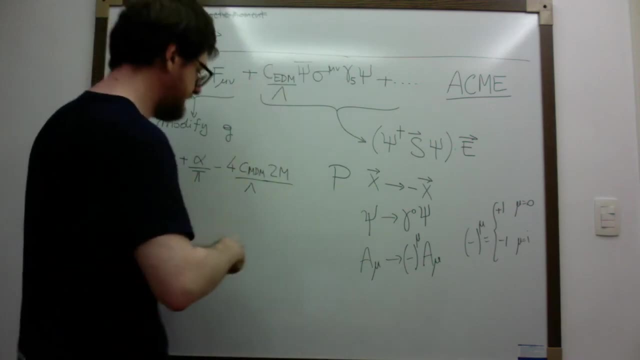 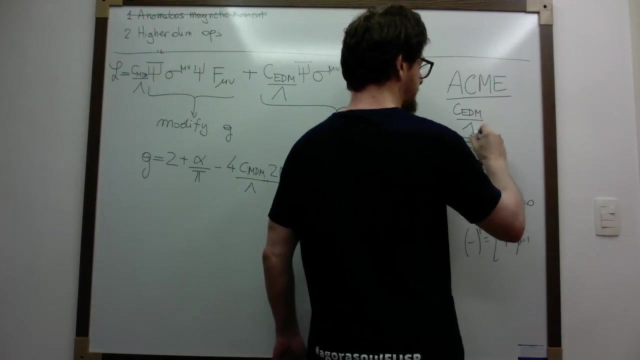 which I do not remember by heart. So the effect, the bound that you can put on this, on this coefficient here from the ACME experiment, so let me write it here- is that one See, electric vapor moment over lambda must be smaller than something like 10 to the minus 19. 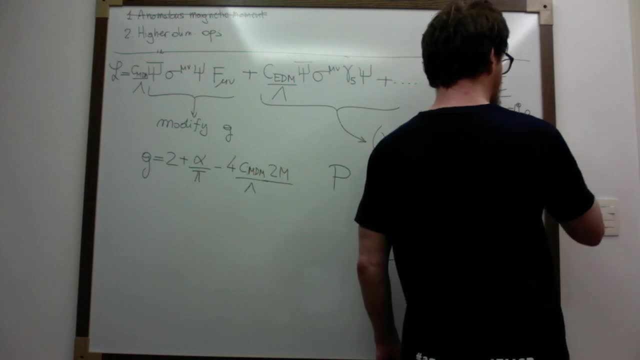 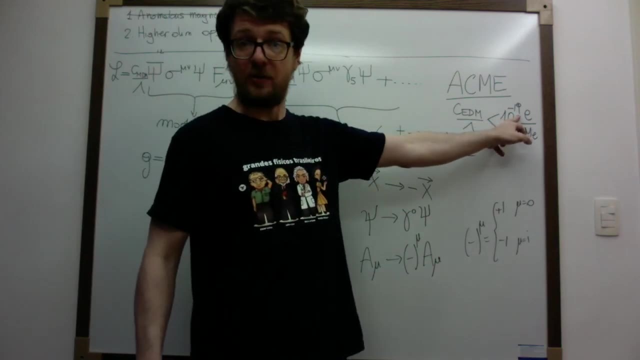 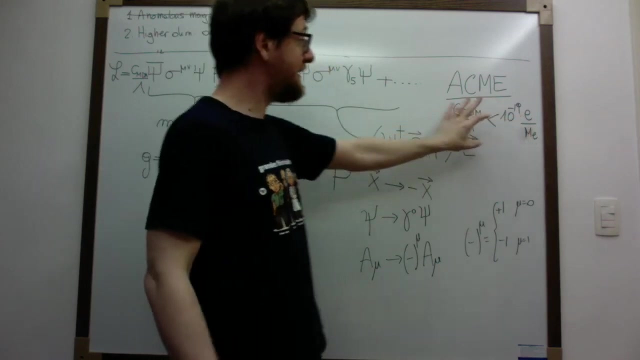 electric charge divided by the electric electron mass. okay, So this is an extremely small number: 10 to the minus 19.. And this so, since this is an extremely small number, this means that this bound is extremely aggressive, okay? So, for some reason that we do not know, 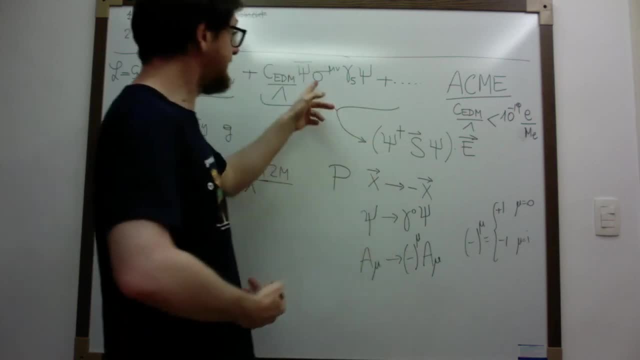 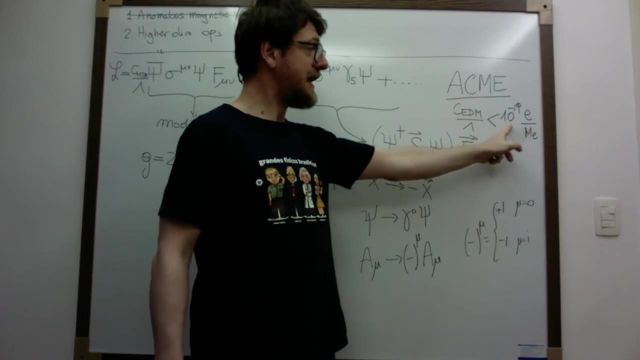 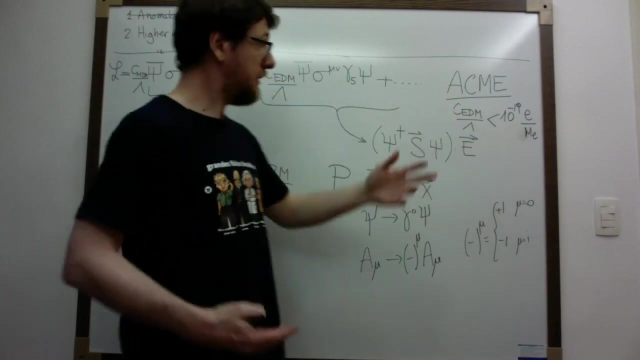 we do not understand. what this is telling us is that this operator, which appears at the level of dimension five, must have a coefficient which is extremely small to be compatible with our current experimental data. This can happen for two reasons. Either lambda is huge, so QED. 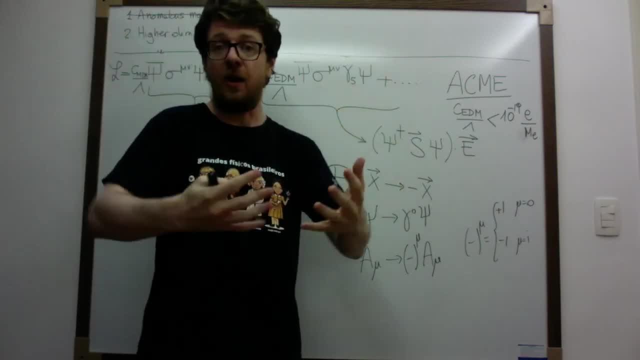 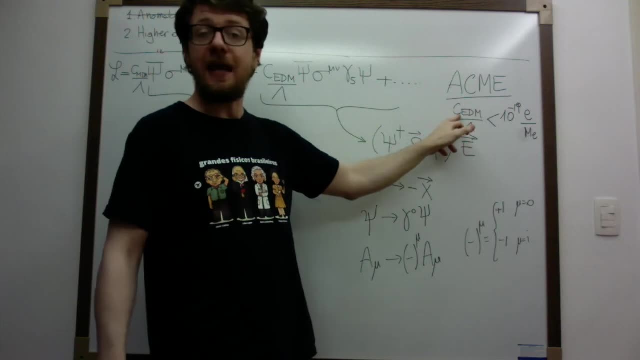 or, in the case of a particle, in the complete theory, the standard model is really valid up to very, very, very high energies, or for some reason. this coefficient, CEDM, is extremely small, And so it will allow, can allow- for a lambda. 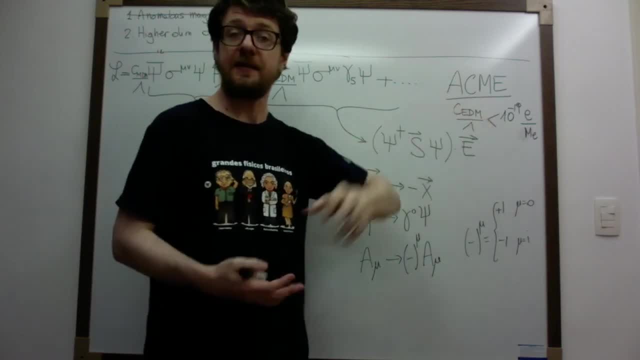 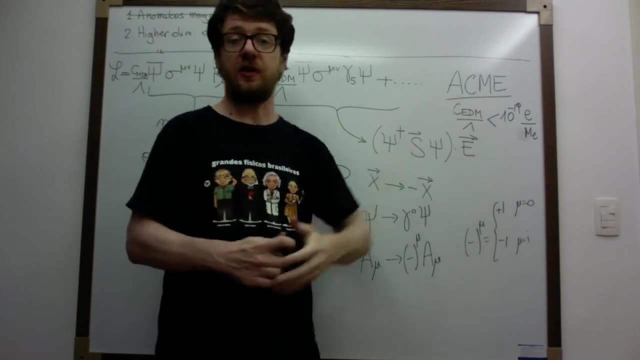 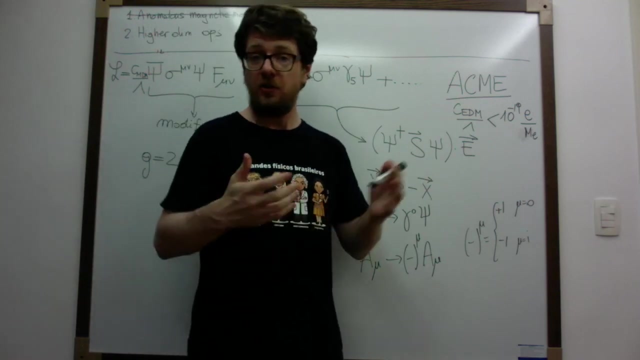 which is not extremely large, but still it will suppress this effect. okay, There are ways in which this coefficient can be smaller. It can be a small breaking of this parity symmetry. So this is a, this is a possibility. You need to see, essentially, what is the. 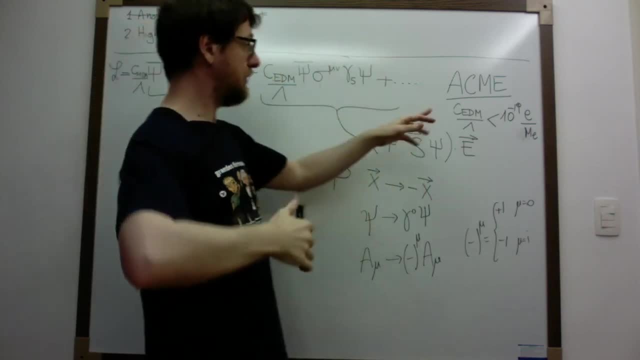 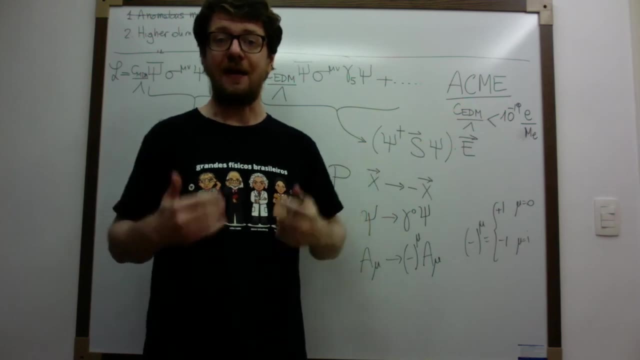 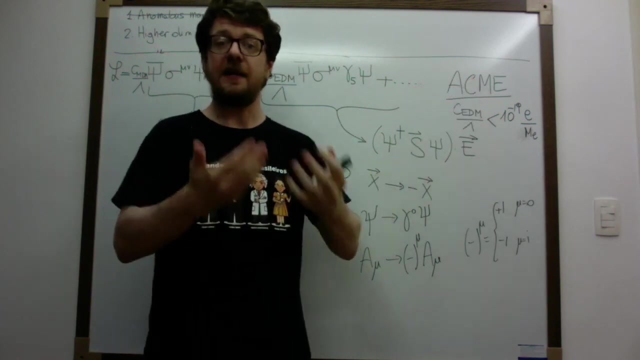 what is that is going to replace the standard model high energy, to infer. if there is something special about this coefficient- Since we do not know what comes after the standard model- higher energies- then we can't really predict this. So this is an indication that experiments are giving us. 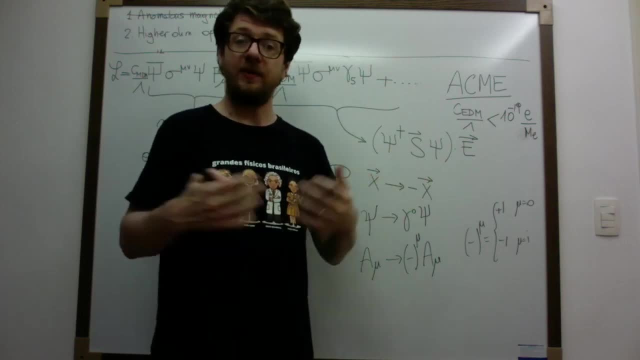 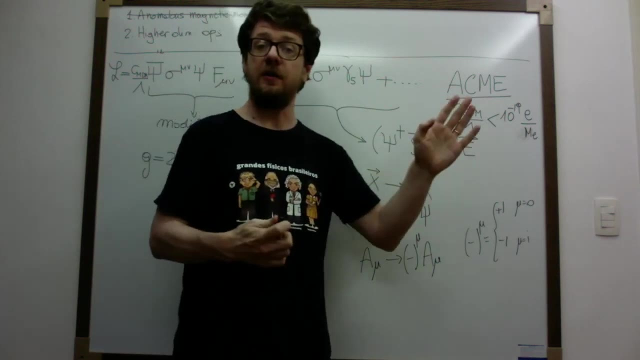 in order to, in order to be aware that whatever is that goes beyond our standard model theory, our standard model, then you should produce such coefficient or such combination C over lambda to be extremely small. Okay, So this is the first lesson that we learn. 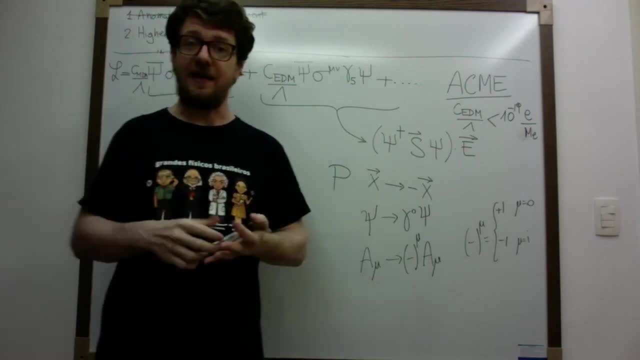 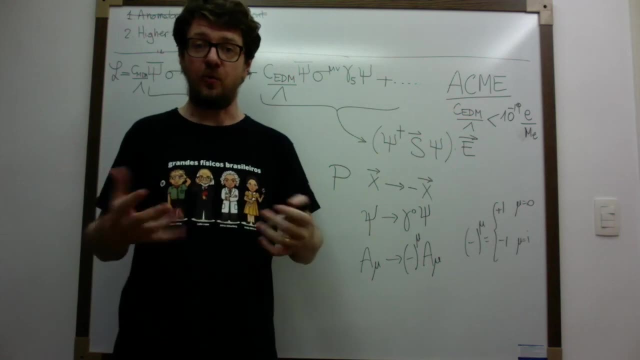 The second lesson that we learn is, that is about something that we already commented when we were talking about effective field theories, which is precisely the fact that a low energy, a very, very low energy, when only the, the renormalizable Lagrangian, 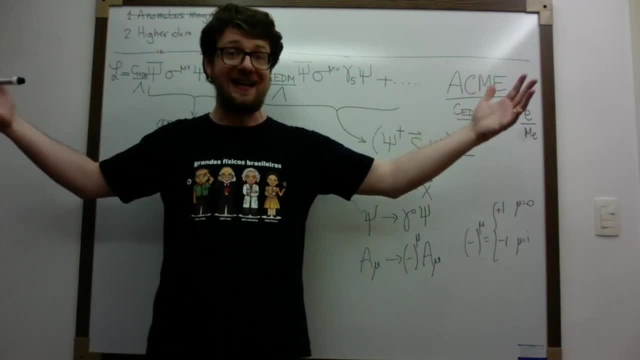 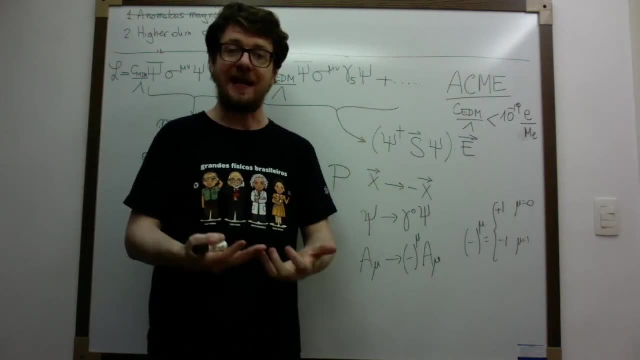 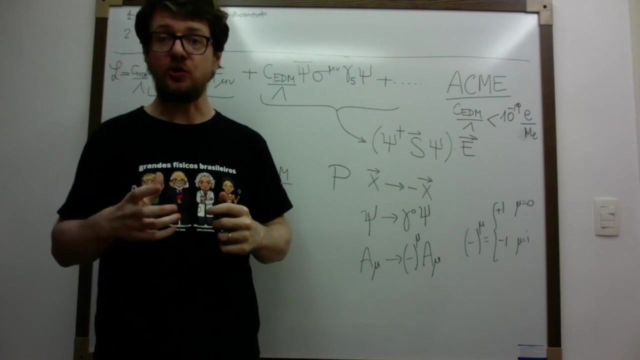 is sufficient to describe our physics. So in very large distance, in very large distance limit, we have more symmetries than the symmetries we have when we start to include higher dimensional terms. right, This is an example that we showed with our computation. 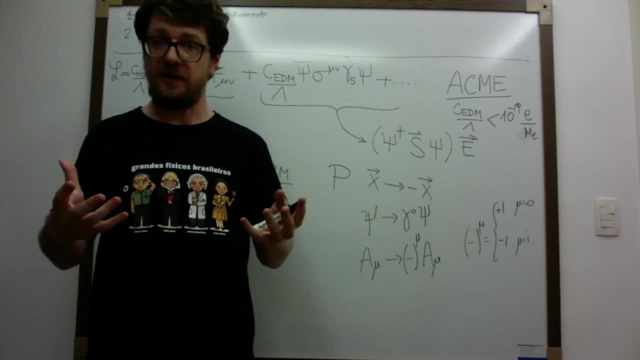 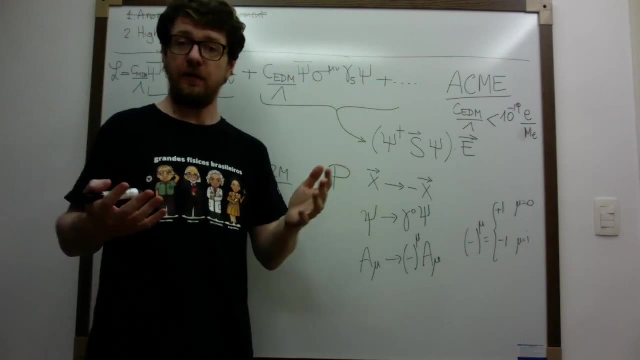 in terms of multipolar, of the potential of a charge distribution, And what we have seen here is precisely the same kind of phenomena. At the level of dimension four, Lagrangian or dimension four operators, parity is a symmetry. At the level of dimension five: 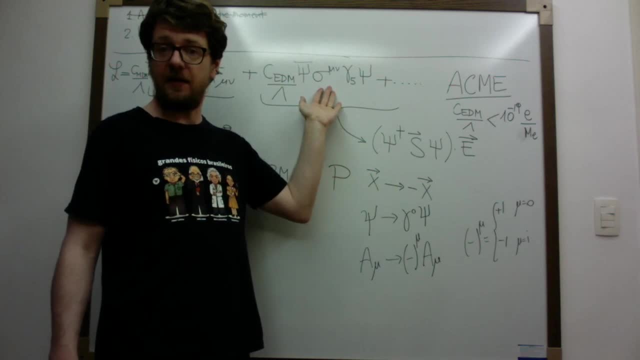 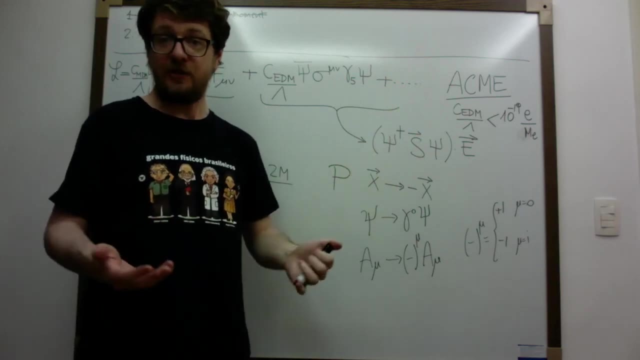 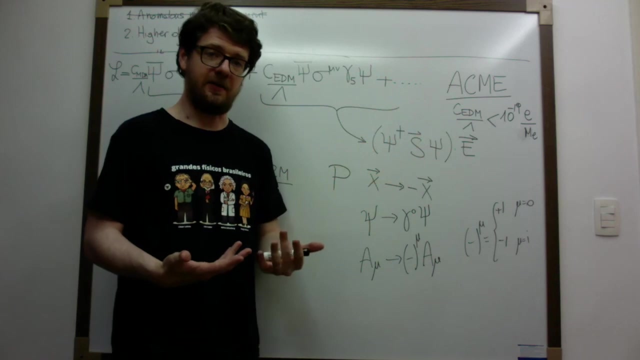 we already have a term that breaks that symmetry. Okay, At the level of dimension six, we have many, many terms that actually break parity And and so you see that we keep losing these, these kind of okay. So this is another lesson. 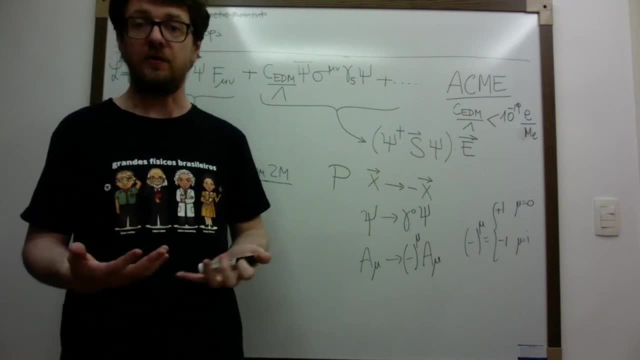 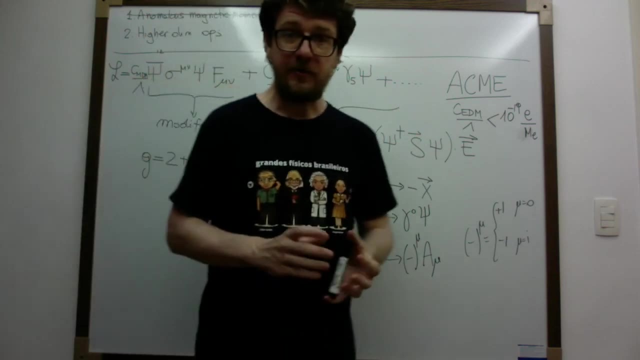 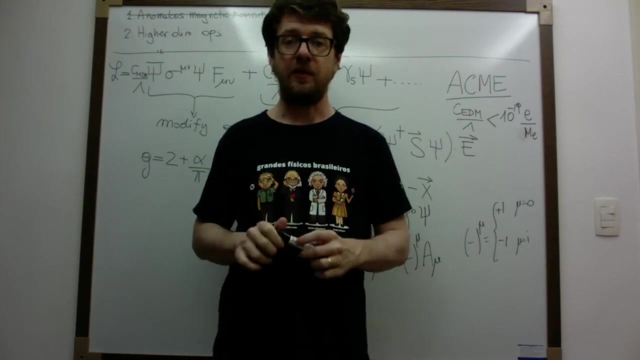 We already mentioned it in a context that was not quantum field theory, And now we are actually seeing concretely in a quantum field theory example- Excellent. So this was all I wanted to tell you about QED, So we close here this part of the course.